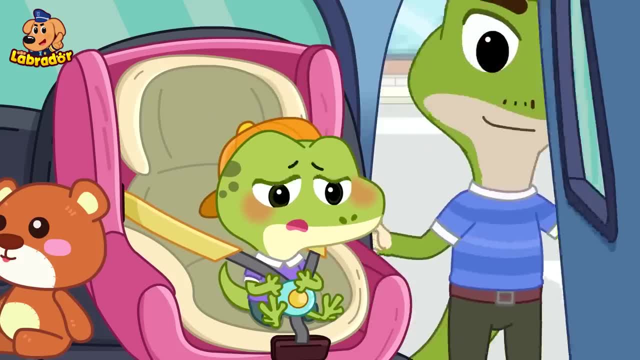 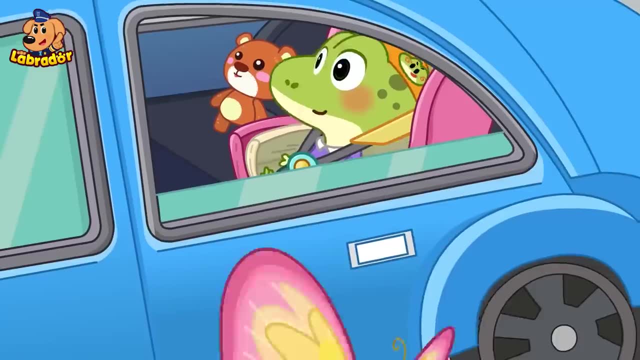 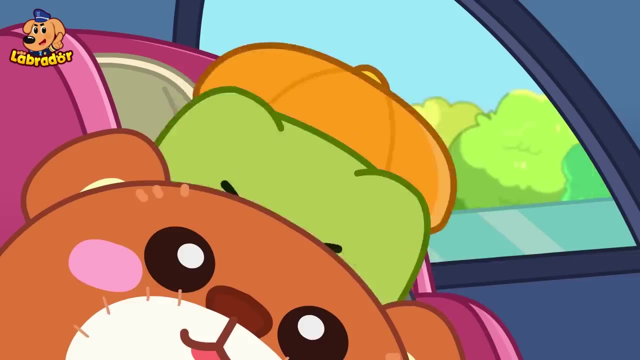 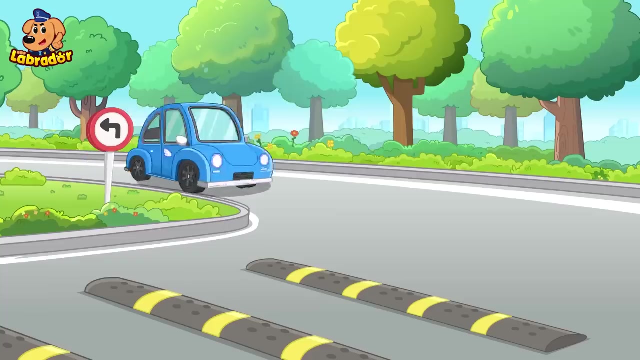 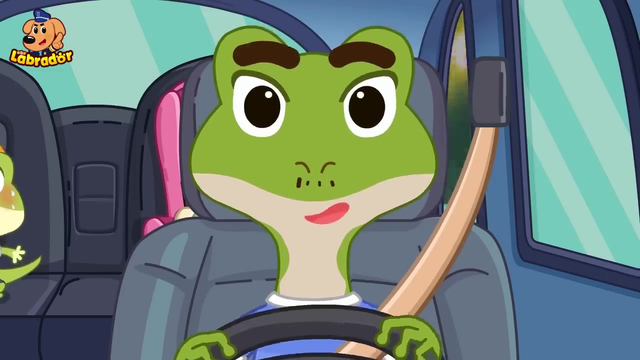 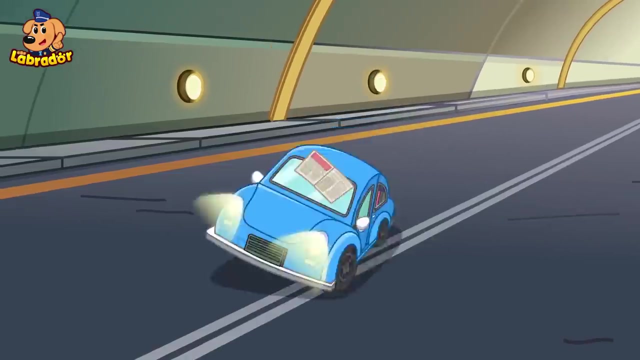 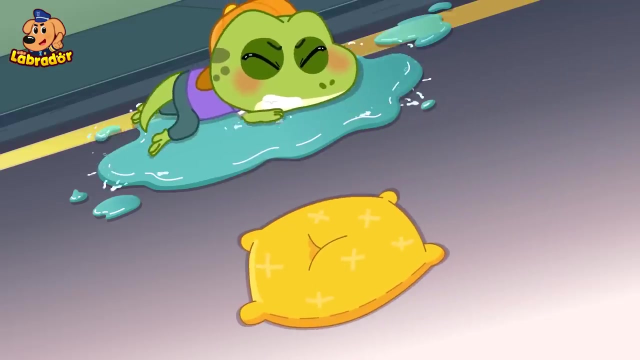 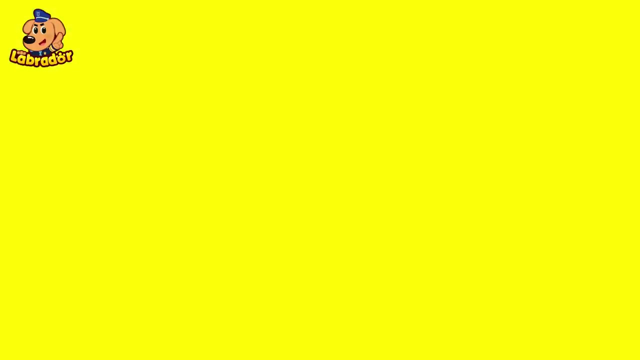 Sweetie, you should. It will keep you safe. Buckle up, Let's go. You can sit here. Sure, I can't see anything. Oh, Oh, Oh, Oh, Oh, Oh, Oh, Ready, It's all done. 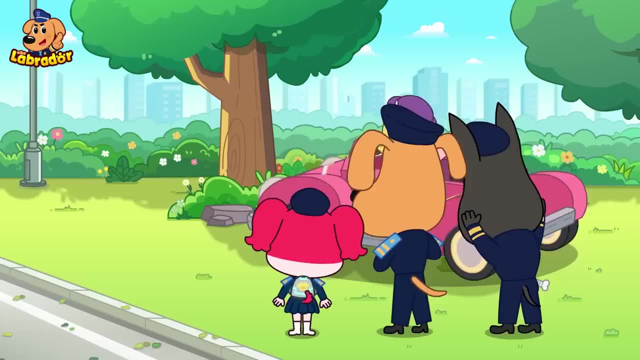 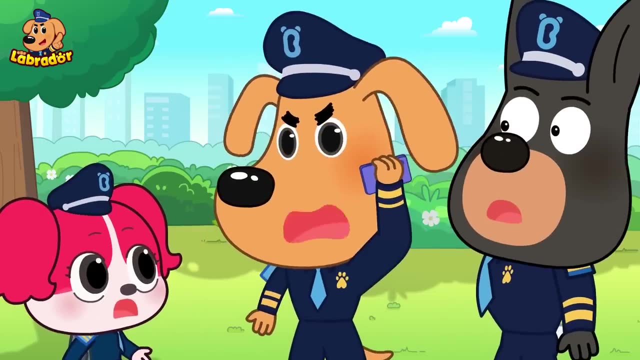 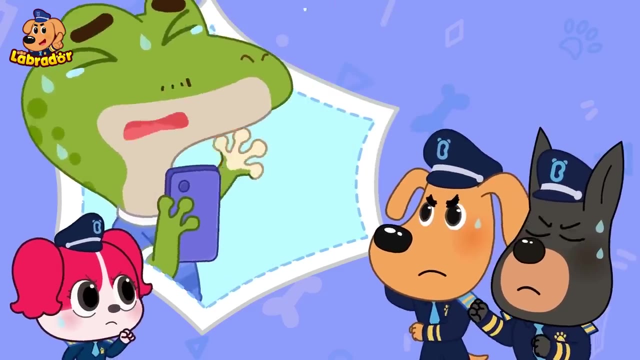 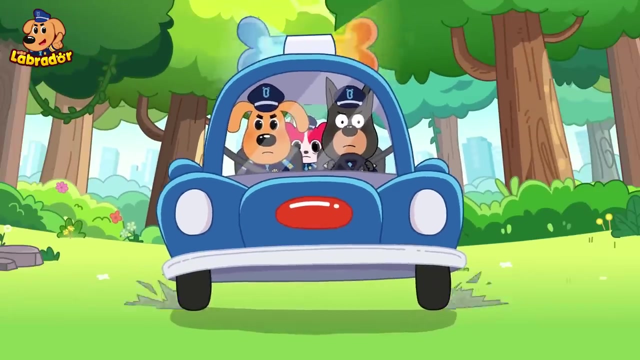 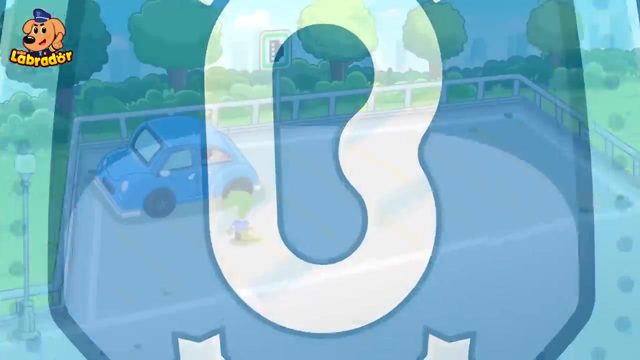 Thank you so much. Bye-bye, Bye, Woof. Hi, I'm Sheriff Labrador. Sheriff Labrador, My son was just in the car and suddenly disappeared. Please help, We'll be right there, Sheriff Labrador, Don't worry. 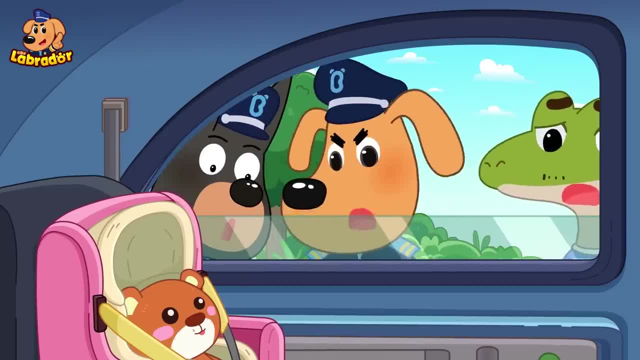 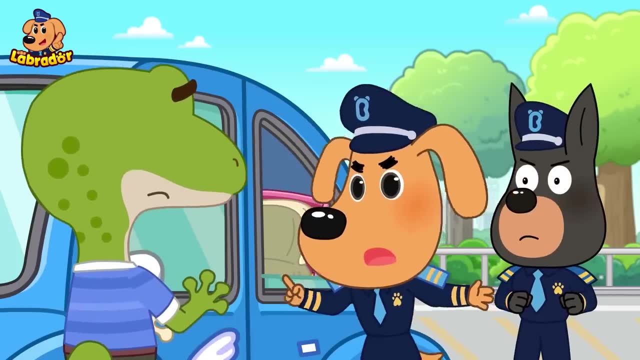 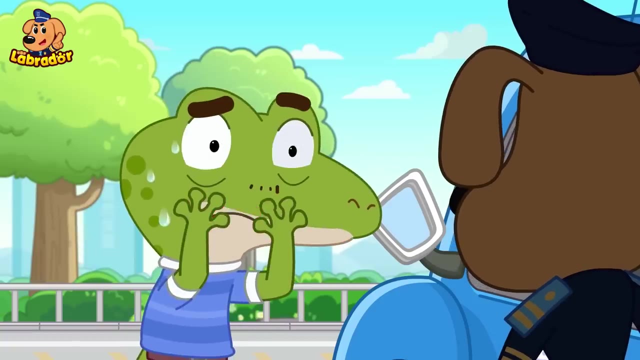 Let us check first. Ah, looks like he wasn't sitting in his car seat. Mr Gekko, did anything unusual happen while you were driving? Yes, A piece of newspaper blocked my view, so I had to make a sharp turn. 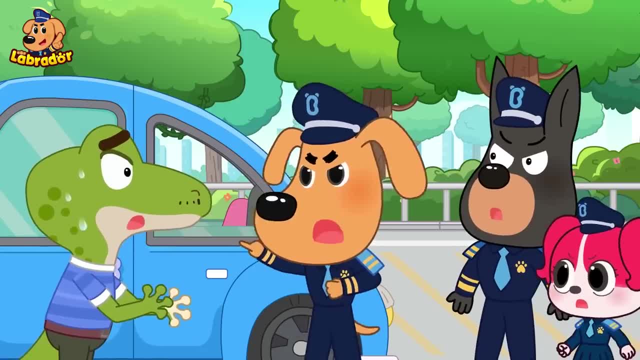 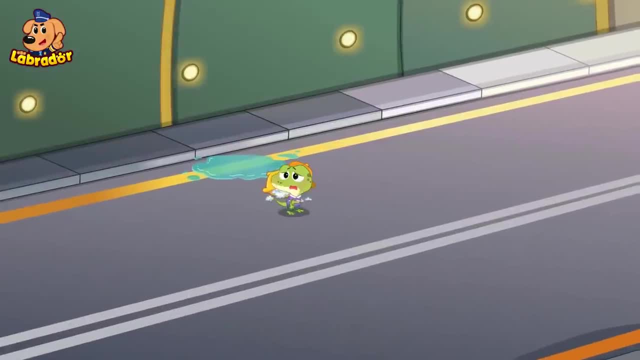 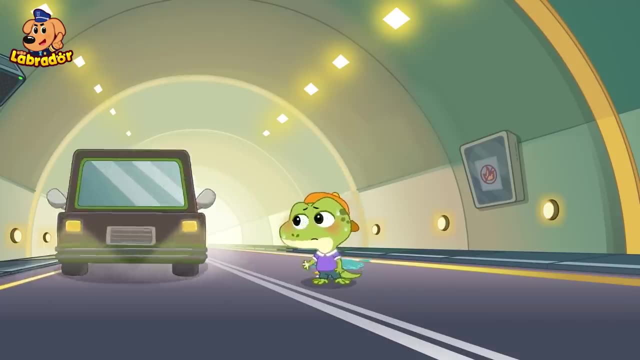 It seems like little Gekko was thrown out of the car because he wasn't sitting in his car seat. Ah, Let's go find him now. Ahem, Ahem, Oh, my arm hurts. Oh, Daddy, Ah, Oof. 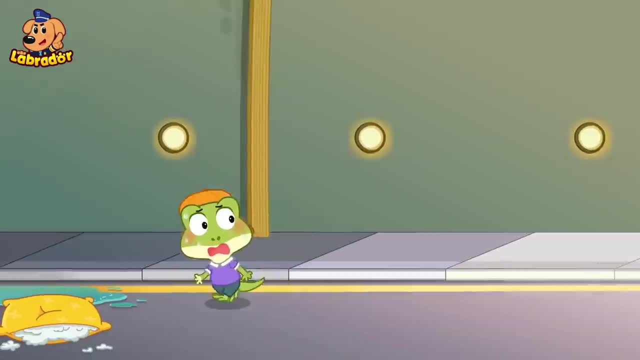 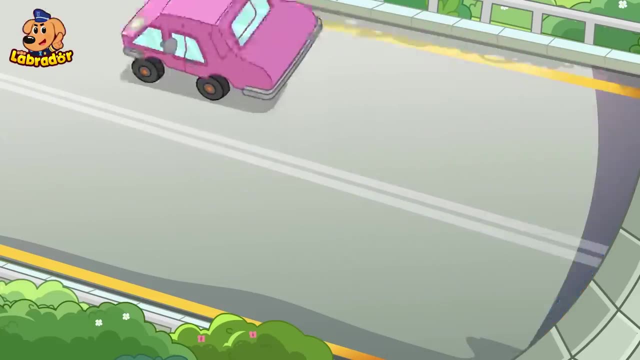 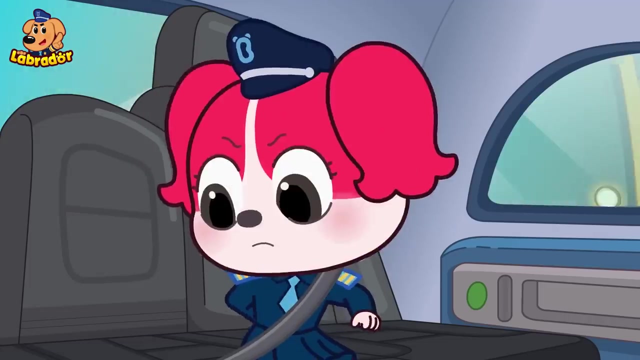 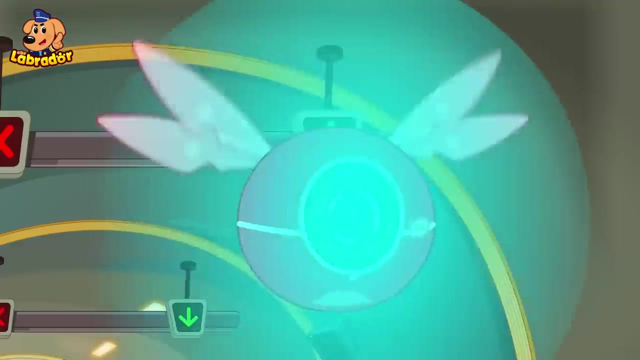 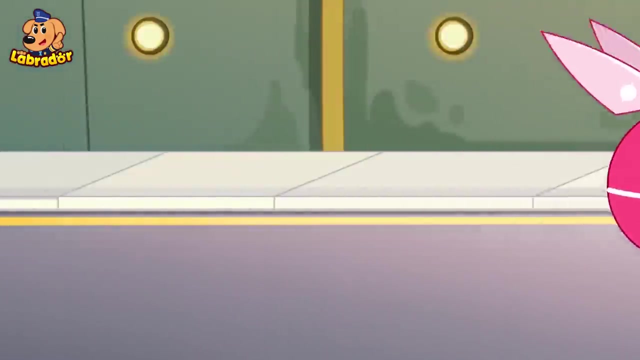 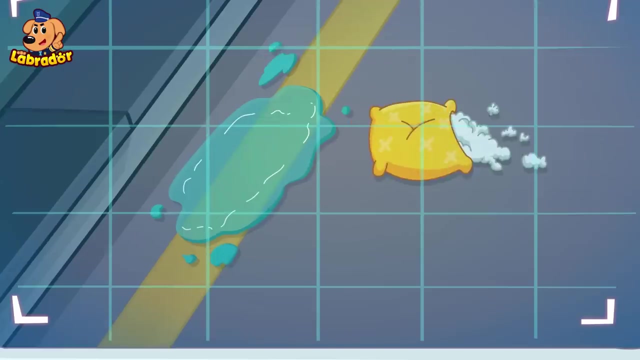 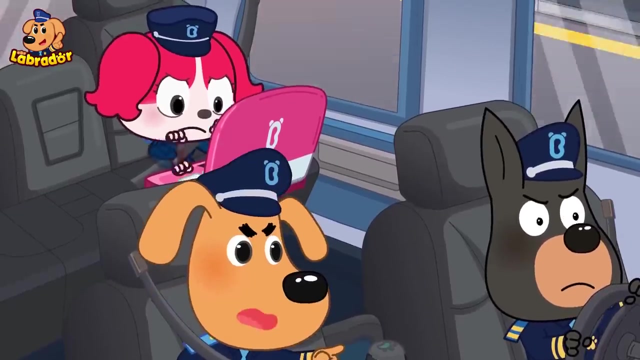 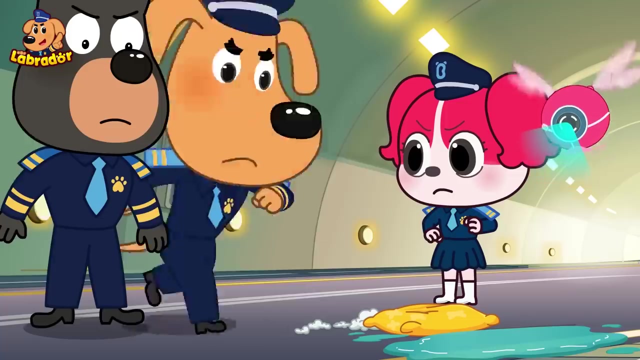 Ah, Ah, Daddy, where are you? Papillon search with your super flying eye. Got it. Little Gekko, where are you? I found a cushion on the ground. ahead, Let's go. I think this is Little Gecko's cushion. 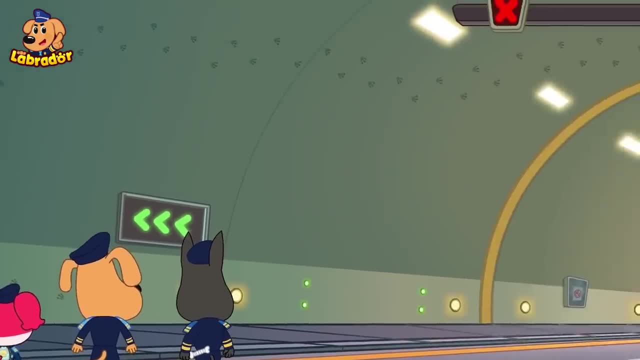 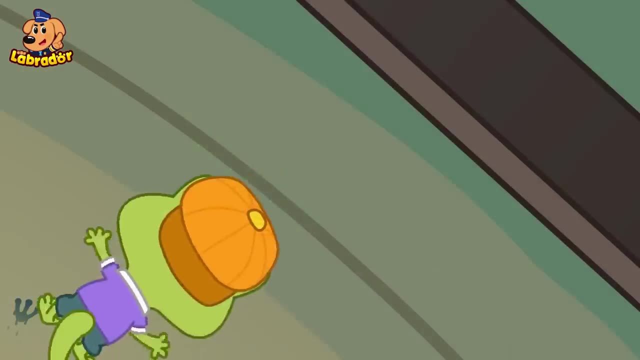 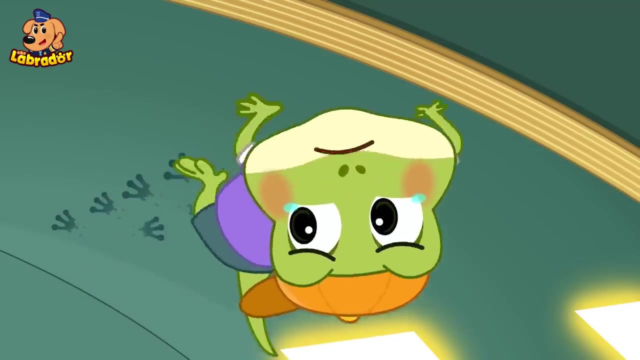 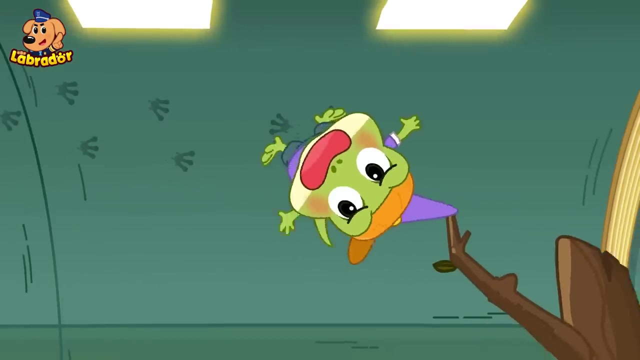 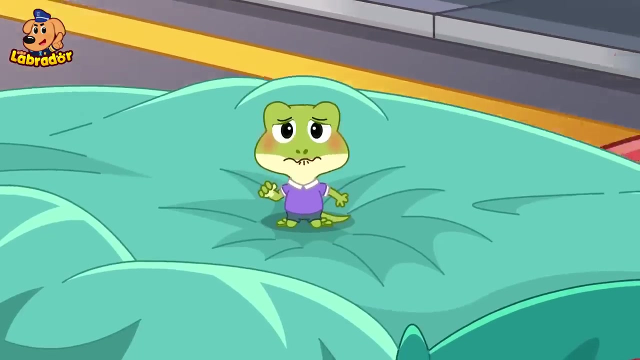 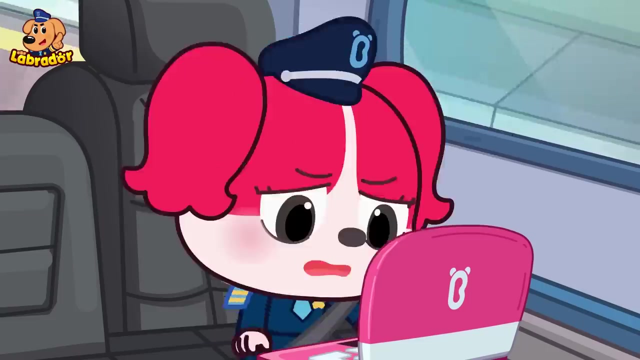 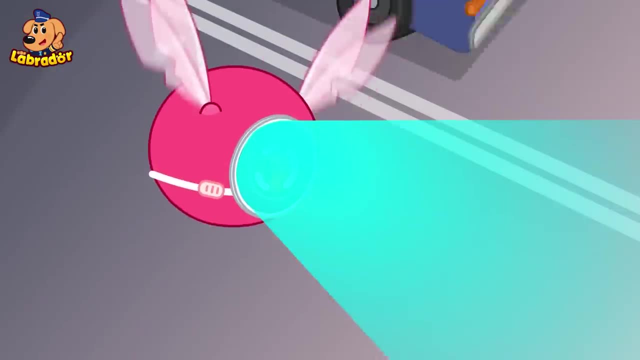 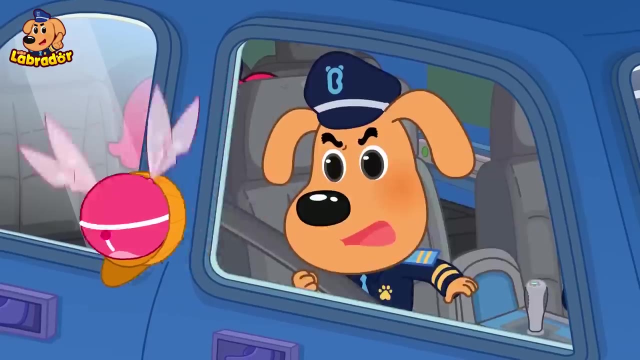 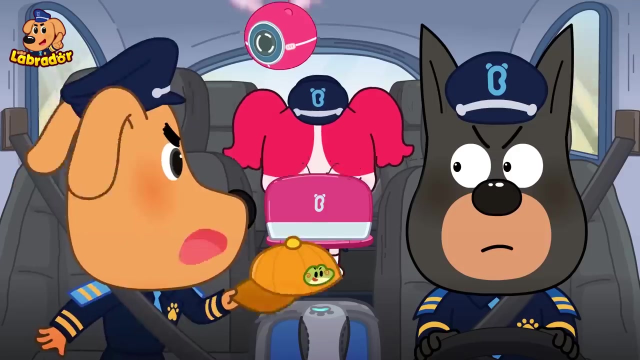 Let's see if he's nearby. Huh, What's that Error? Error Returning. now It's Little Gecko's hat. Oh no, He might have fallen. He might have fallen on that bannerhead. Hurry Doby. 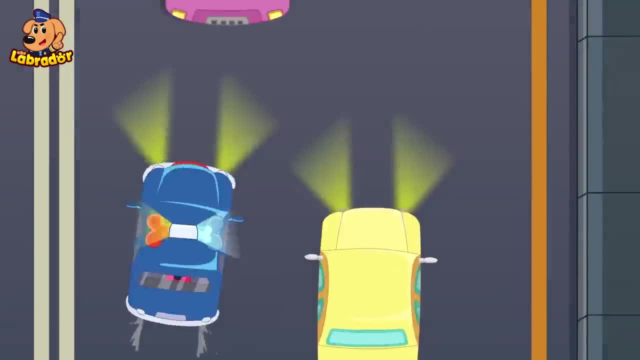 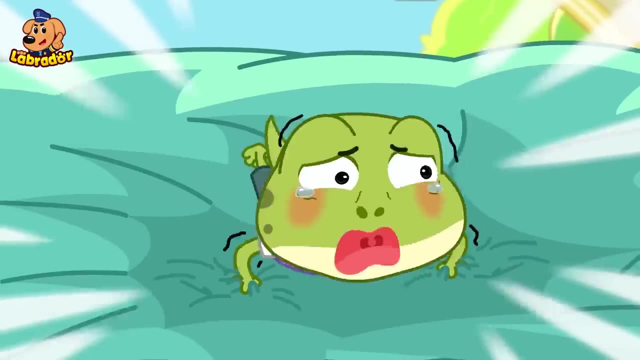 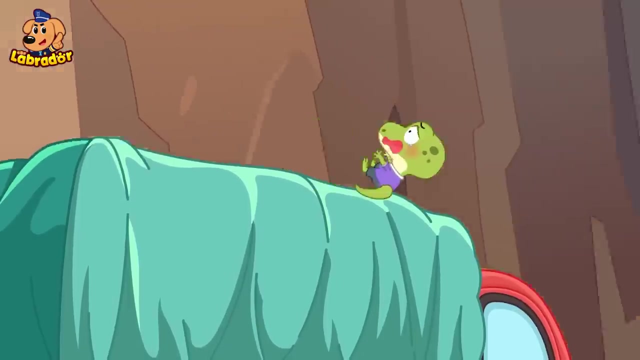 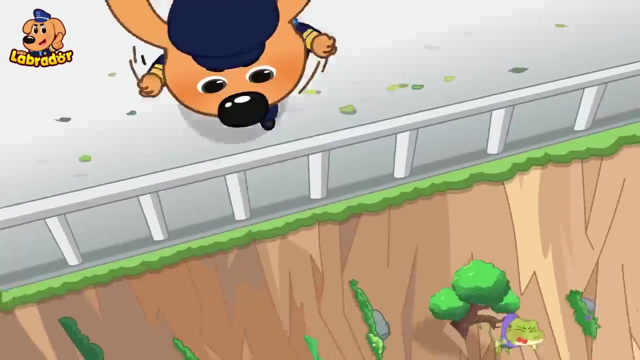 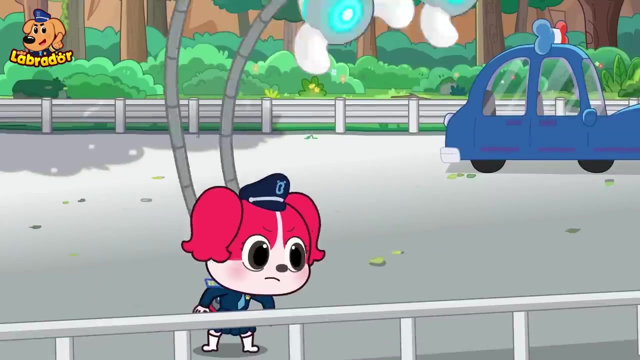 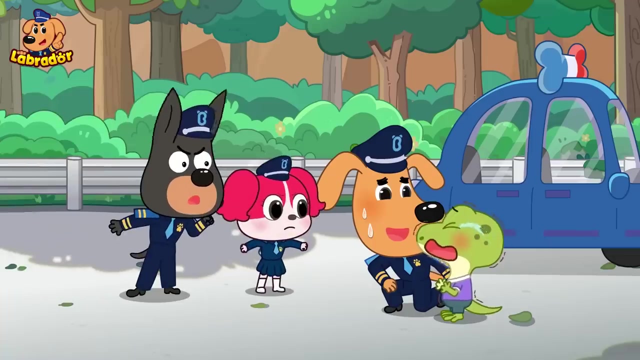 Leave it to me. Look, It's Little Gecko. Help, Help, Help, Help. Little Gekko, Little Gekko. Sheriff Labrador, Everything's fine now. Always sit in your car seat when riding in a car, okay? 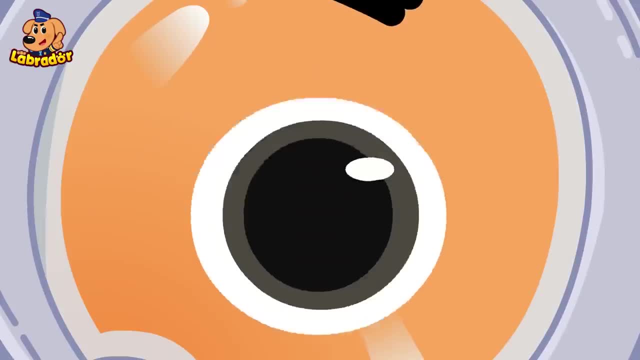 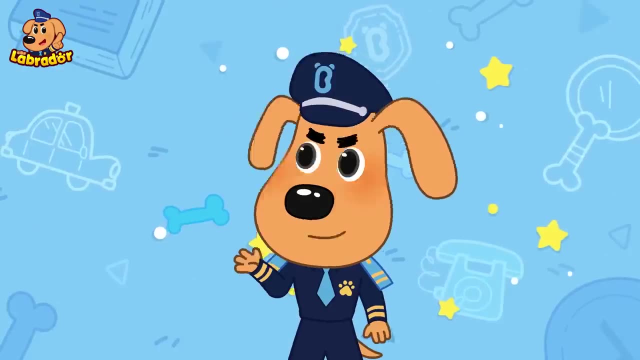 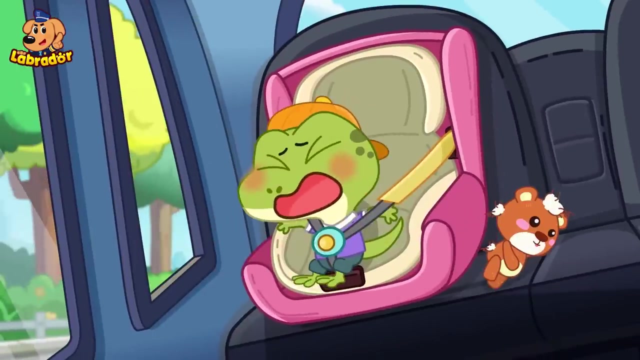 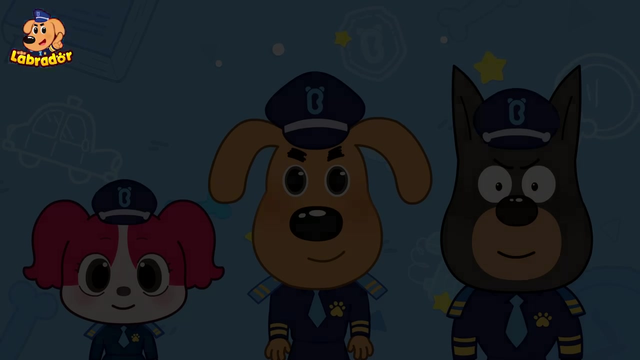 I got it, Sheriff Labrador's: Safety Talk. Kids, you should always sit in your car seat when riding in a car. Car seats can protect you when the car suddenly stops or when there is an accident. Can you remember that? Be careful when you walk. 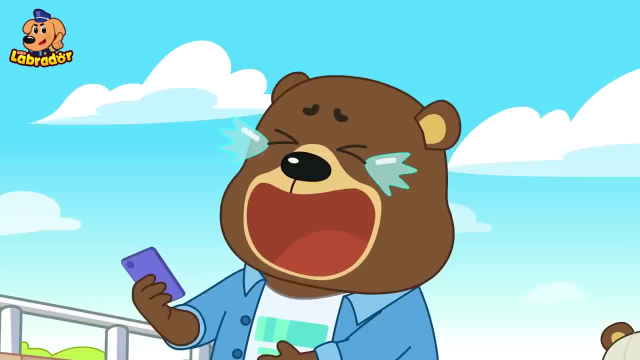 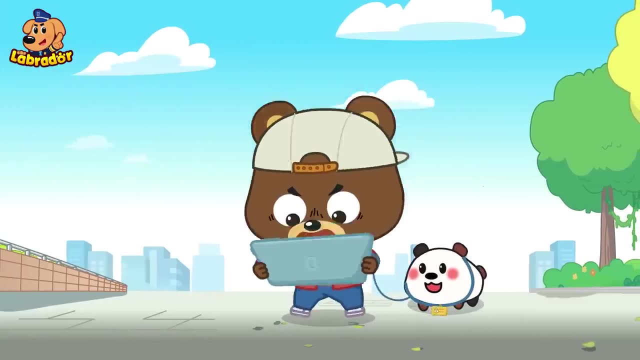 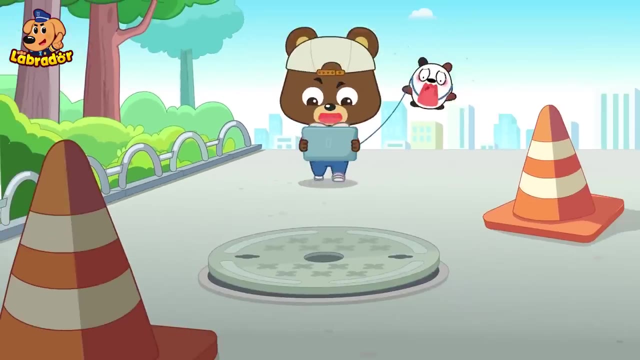 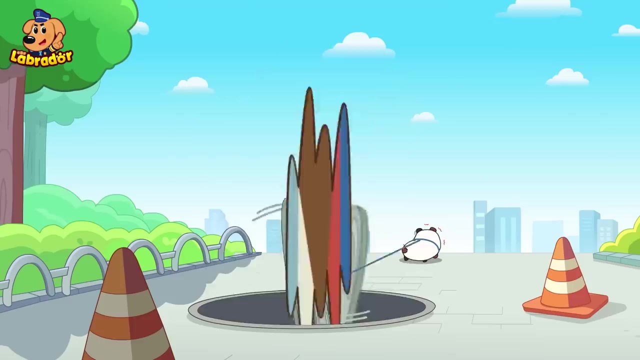 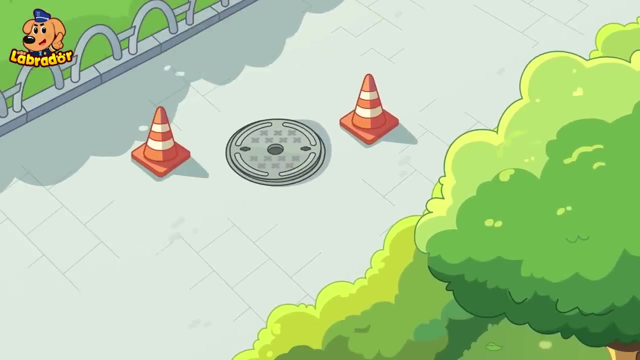 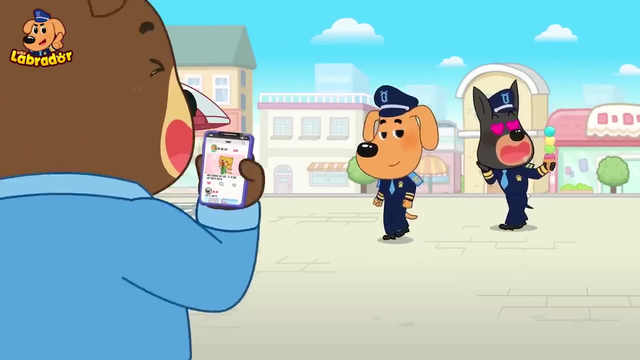 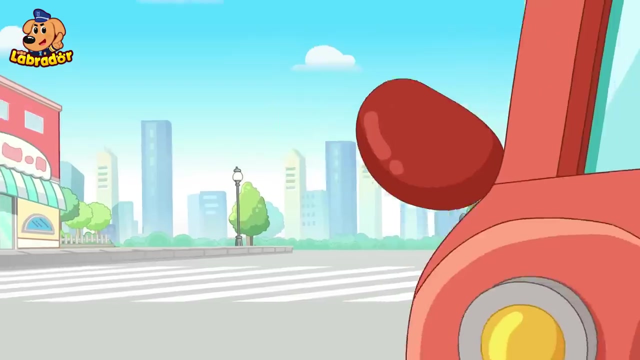 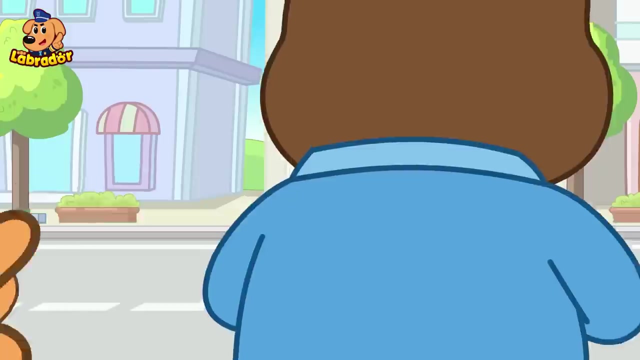 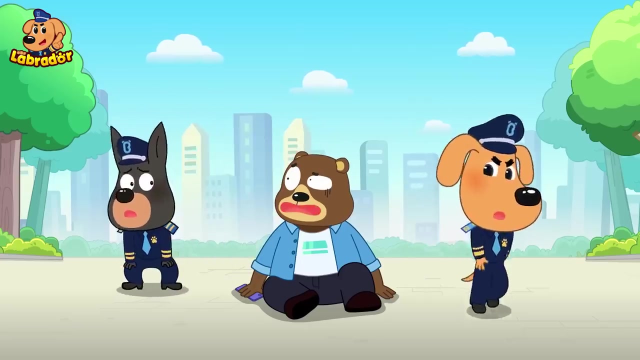 It's so much fun. That's so funny. Hey sweetie, stay close to daddy. I won Lulu. Watch out, Mr Bear. That was so scary. Mr Bear, you shouldn't look at your phone while walking. 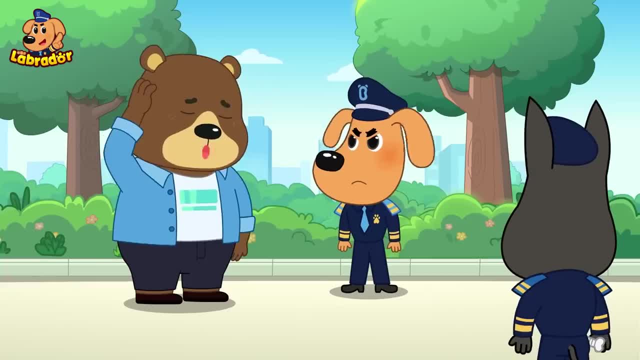 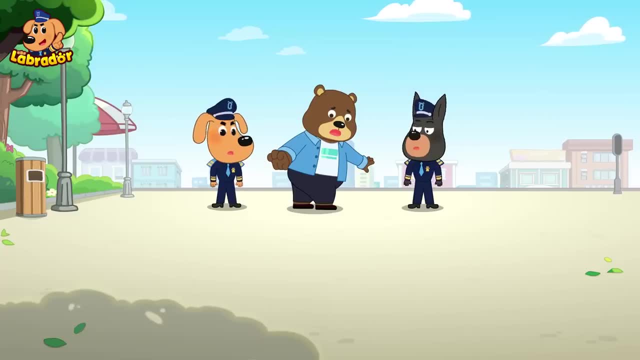 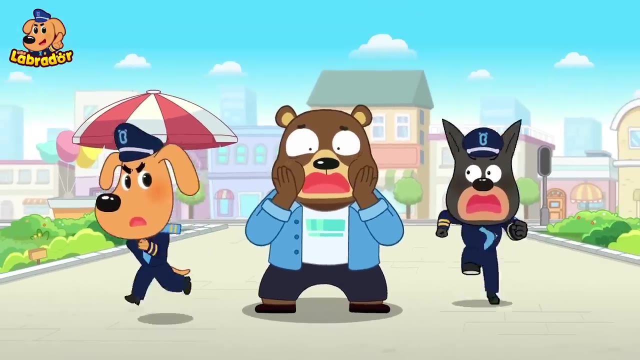 That was really close. Okay, I got it. Sweetie, give your tablet to daddy. Sweetie, Sweetie, Sweetie. My son is missing, Mr Bear, when did you last see him? I have just been looking at my phone. 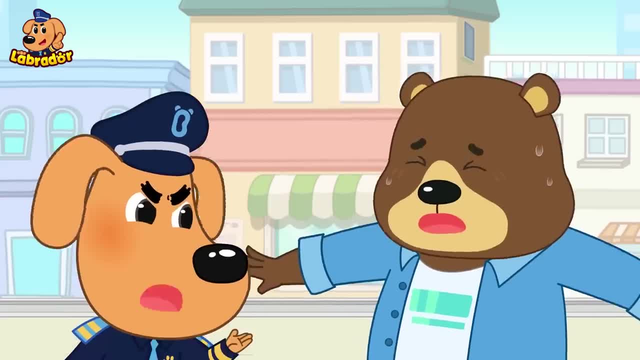 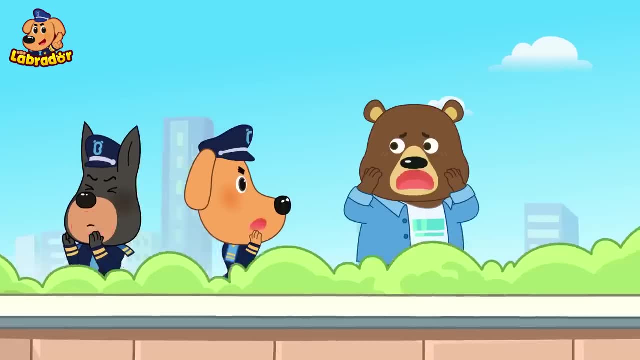 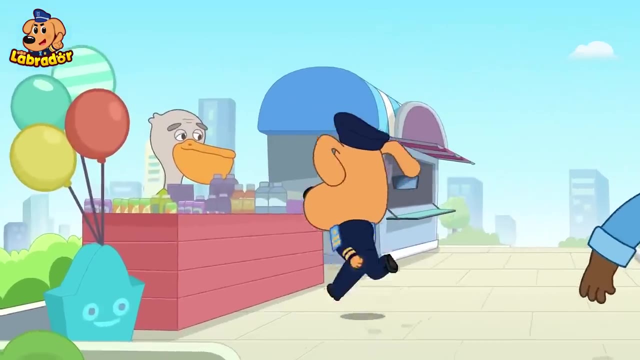 I don't know when he became missing. Let's go back the way you came and look for him. Little Bear, Little Bear, I'll go down and look. Mr Pelican, have you seen Little Bear around? No, I haven't. 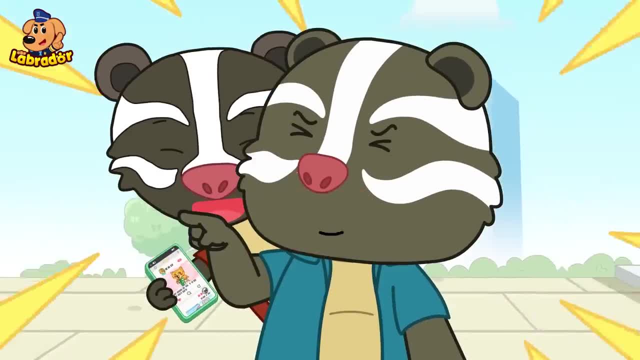 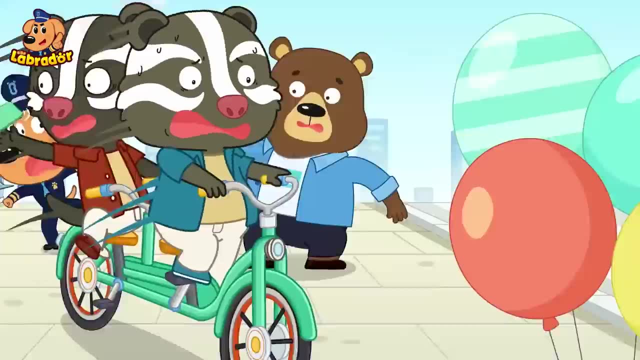 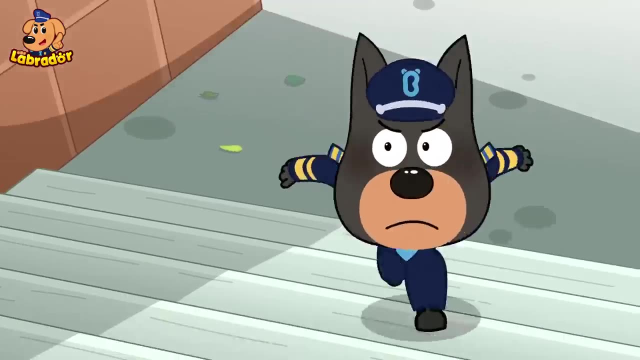 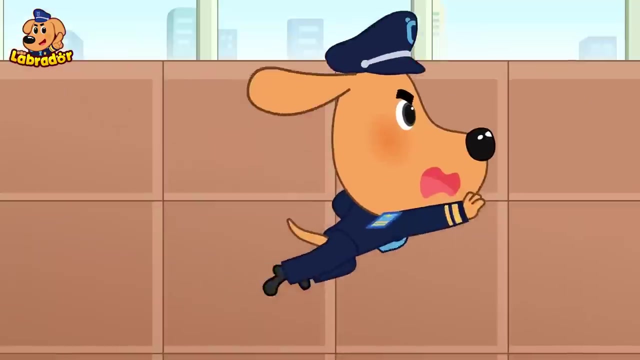 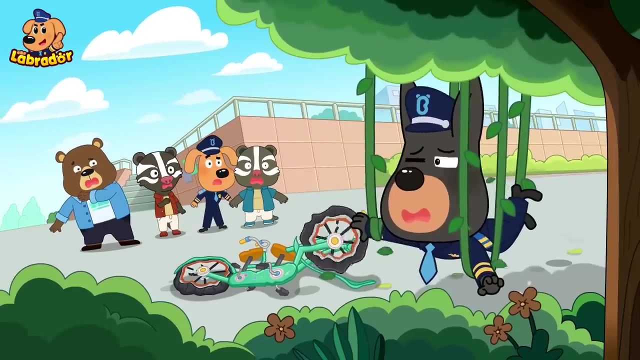 Look at this, It's so funny. Huh, It's so funny. Move aside, Oops, Watch out. There are stairs down there. I'll save you. Watch out. Gah, Ouch, Phew. Good thing that everyone's safe. 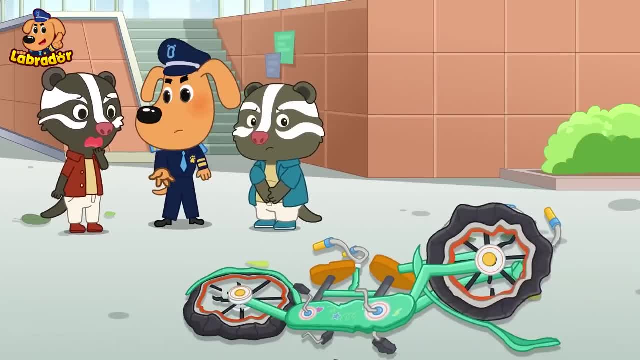 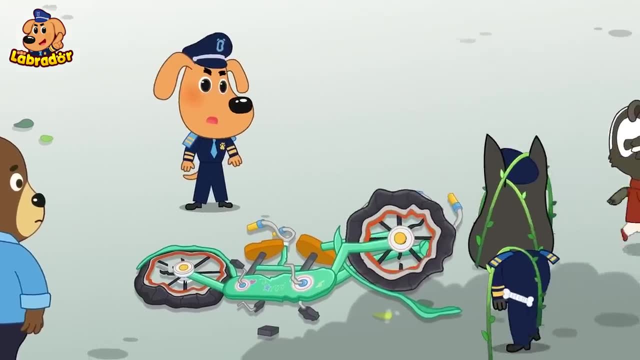 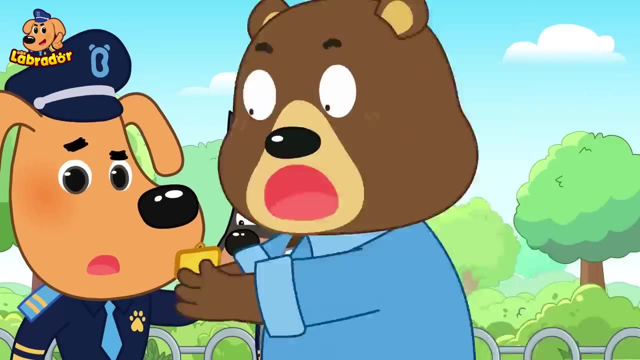 You should look straight ahead when riding a bike, or you might hurt yourself and others. I'm sorry, We'll be careful from now on. What's this? Oh, Ah, Huh, It's my pet Lulu's name tag. 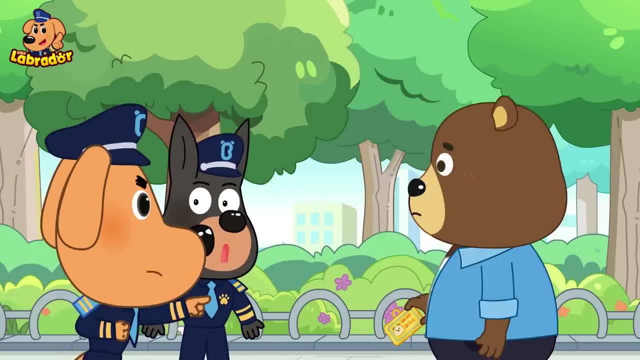 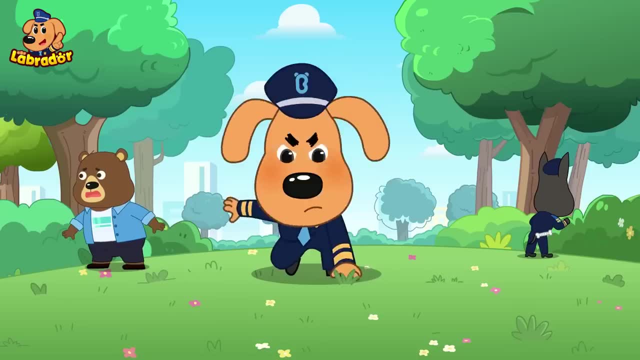 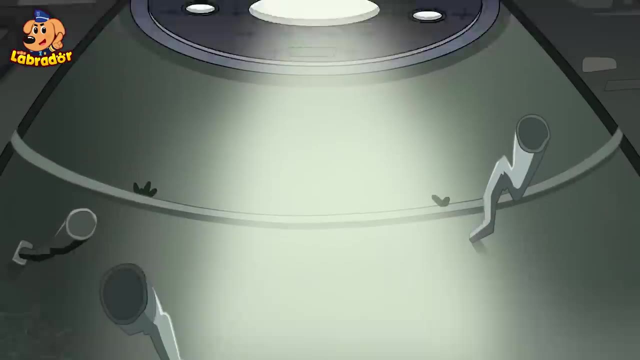 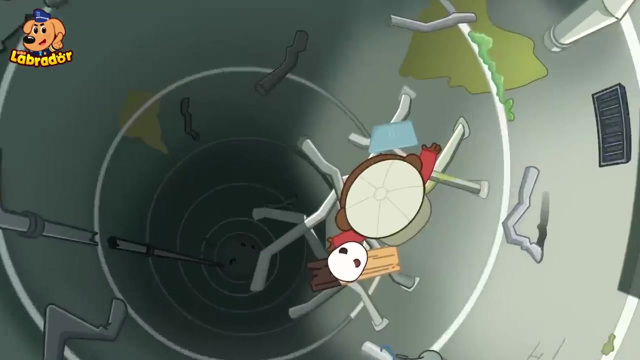 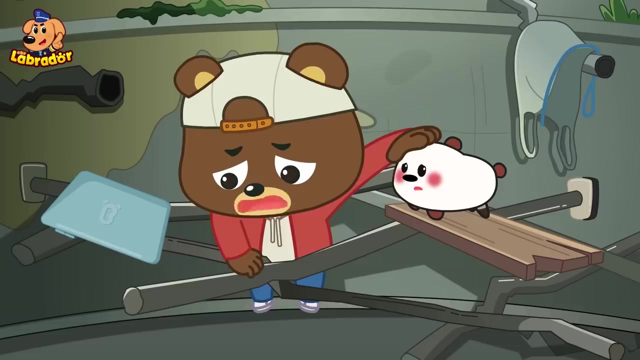 Lulu was with my son. There must be clues nearby. Let's go look for them. These are Lulu's footprints. They went that way, Lulu, Lulu. Sorry, Lulu, It's my fault, I shouldn't have looked at my tablet. 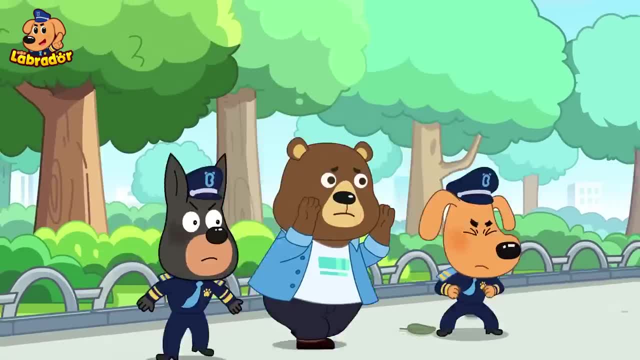 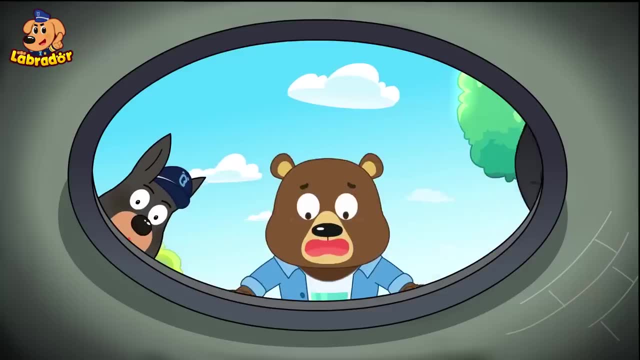 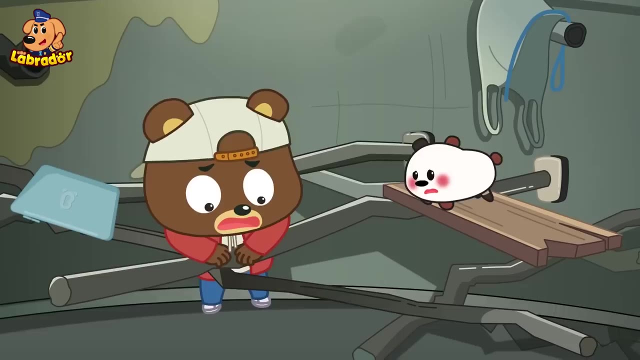 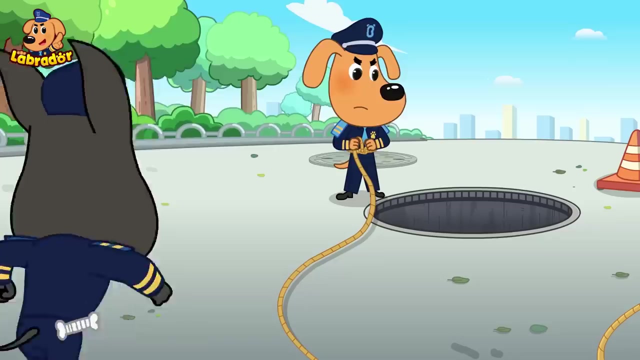 Help Little Bear, Little Bear Help. There's a sound over there. Oh, Sweetie Lulu, Help us. please Don't move. I'll come save you right now. Huh, Huh, Huh. 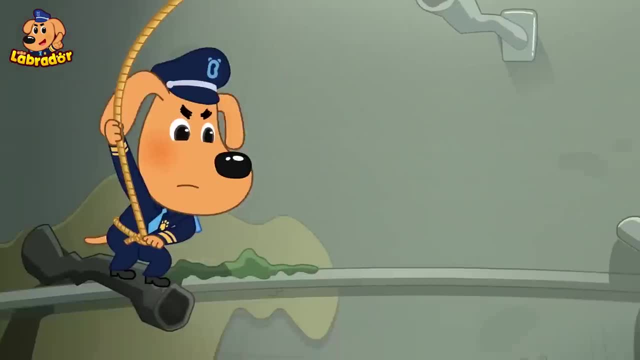 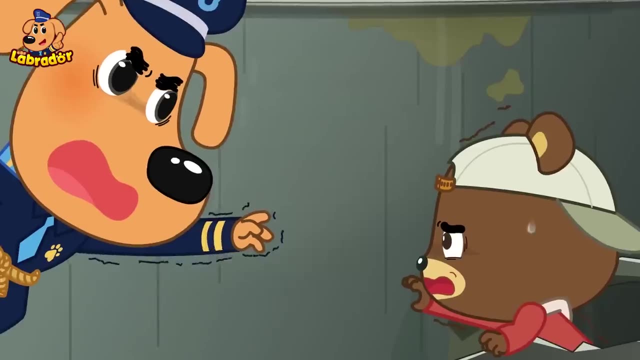 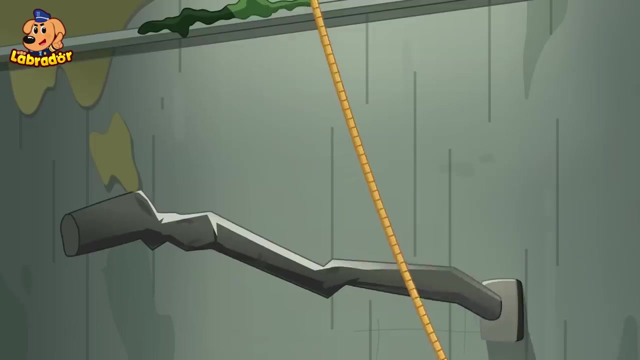 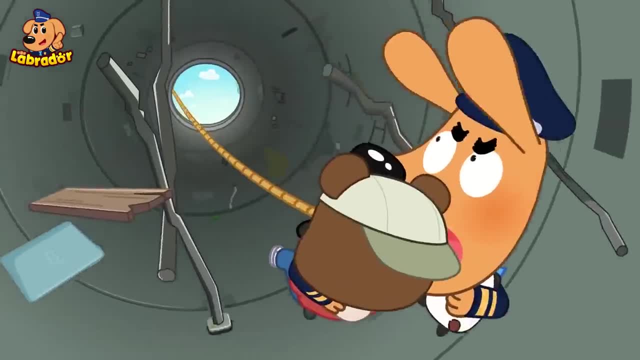 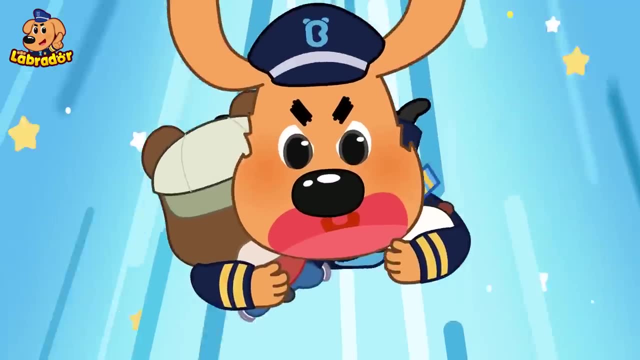 Huh, Huh, Huh, Little Bear, Huh, Hey Gobi, Pull us up, Gah, Gah, Gah, Gah, Gah, Gah Gah, I'll help too. 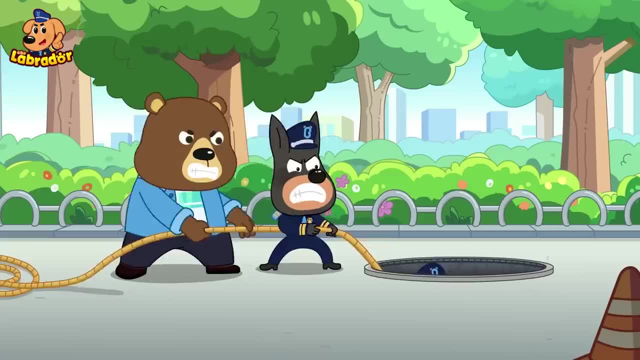 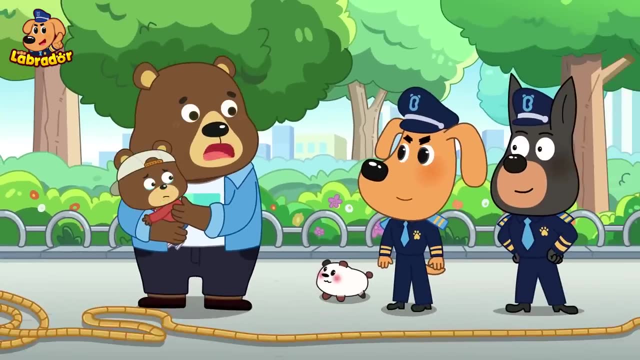 Ha, Gah, Phew, Gah, Gah, Gah, Gah, Gah Gah. That was so scary. Hmm, We'll watch the road while walking from now on. We'll watch the road while walking from now on. 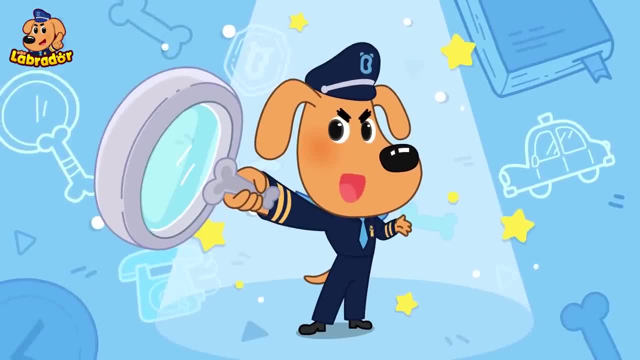 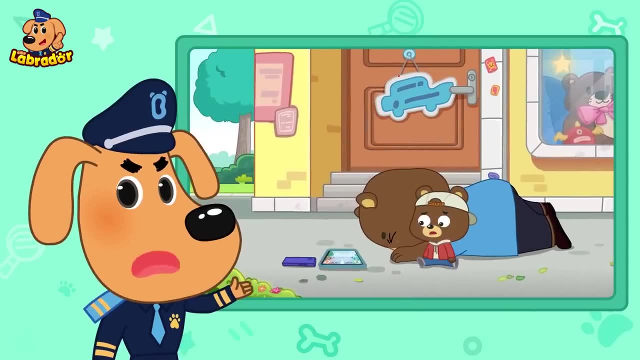 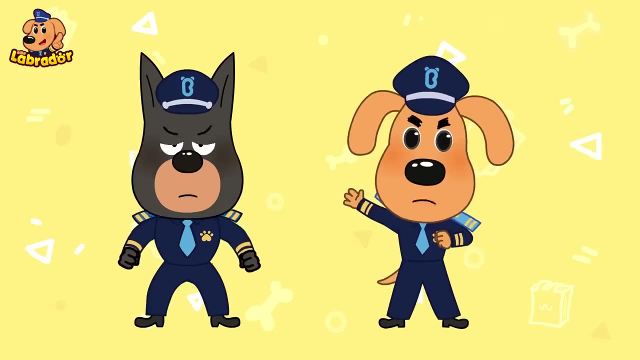 Sheriff Labrador's Safety Talk. Kids, you should always watch where you're going. Don't look at your phones or play games with them, or play games with tablets while walking. You'll lose your focus on the road and might cause accidents, hurting yourselves and even endangering your lives. 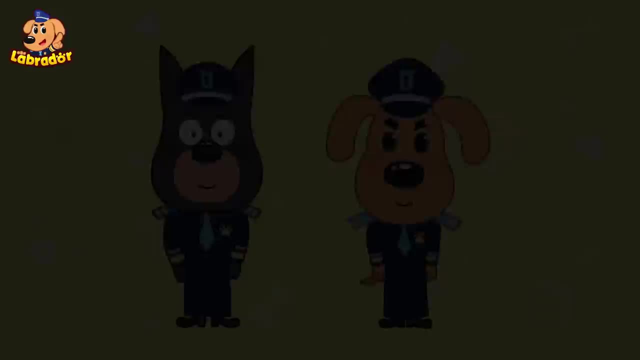 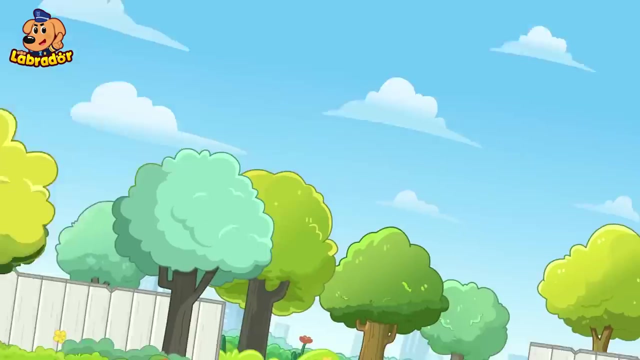 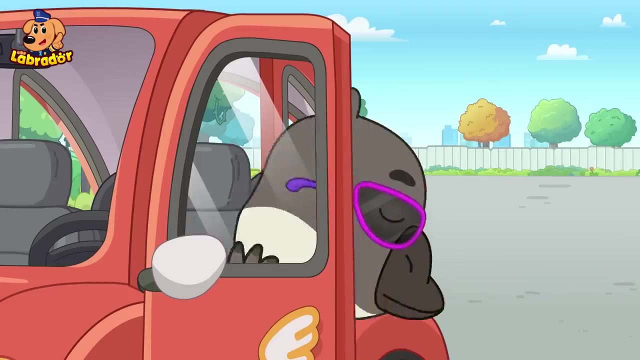 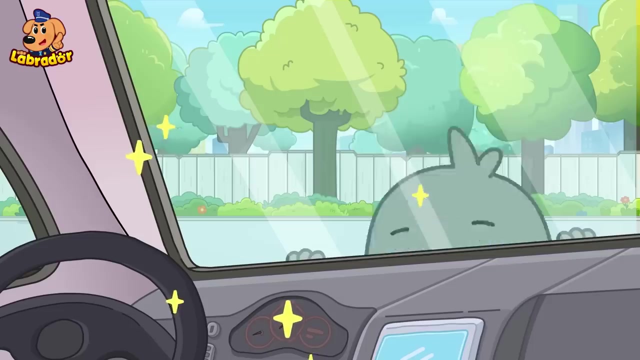 Please remember that Woof, Dangerous, overloaded car Daddy's back. Kids, look, Daddy's got a new car. Wow, It's awesome, Daddy, we want to go for a drive in the new car. All right, Line up everyone. 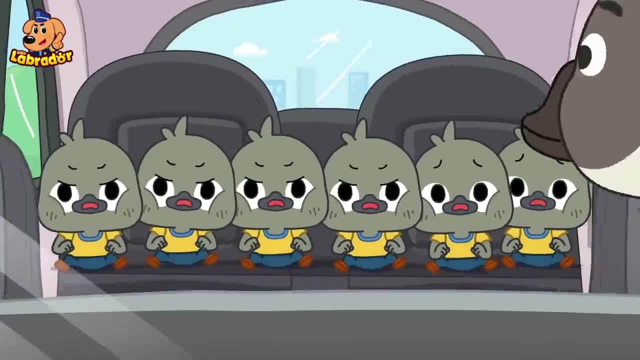 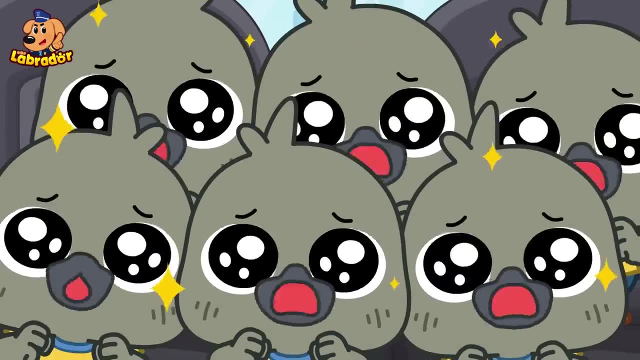 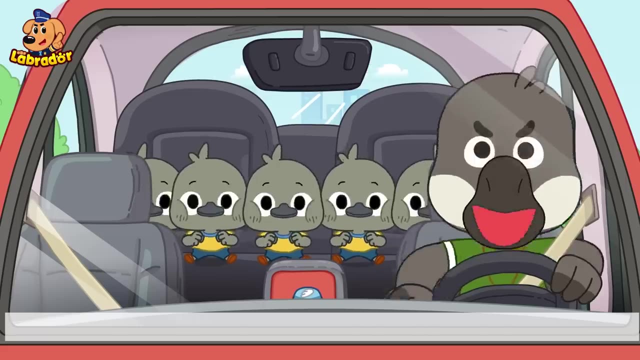 It's too crowded. No, it's not. Let's just stay home today. I'm going to the bathroom. Okay, Please, we really want to go. Then we'll just drive around for a bit, okay, Okay, Sit tight, Let's go. 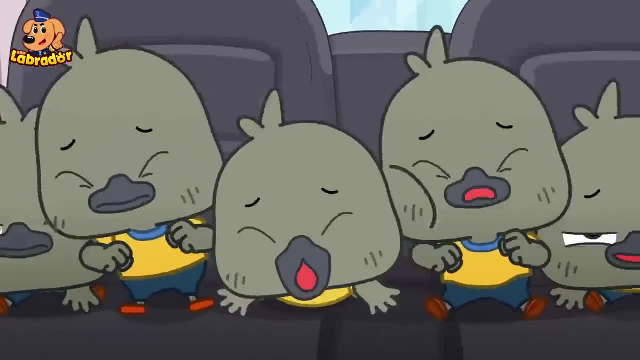 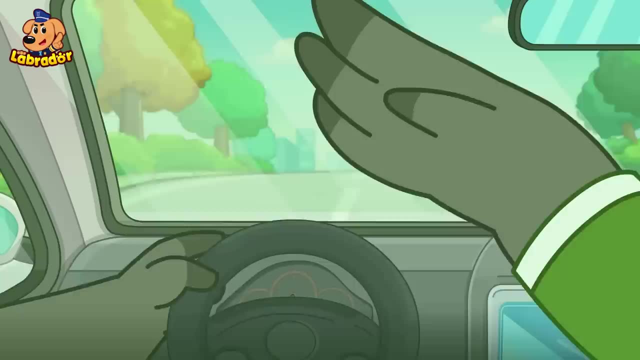 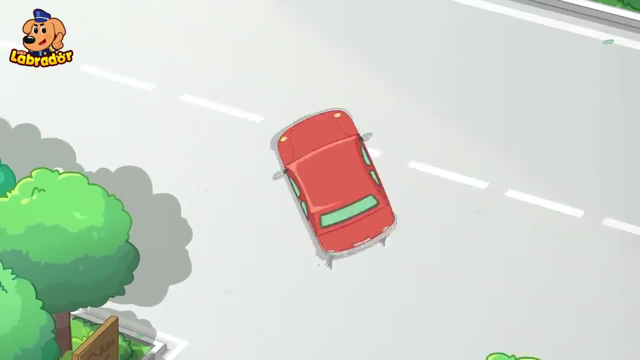 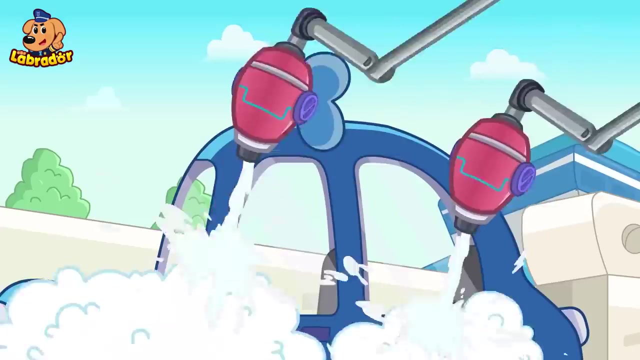 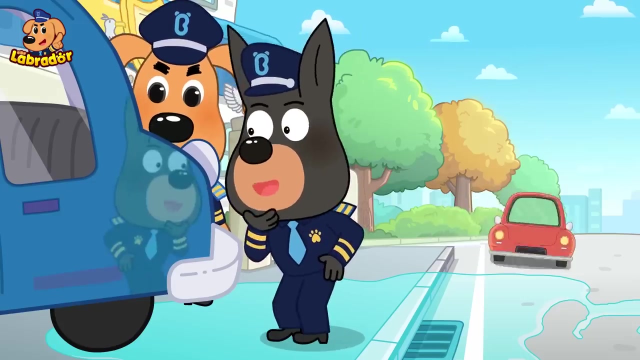 Ouch, I'm stuck. Don't touch me. What's that smell? Huh Huh, Huh, Huh, It stinks, It stinks, Huh. Hey, Watch me. Wow, It's so clean. 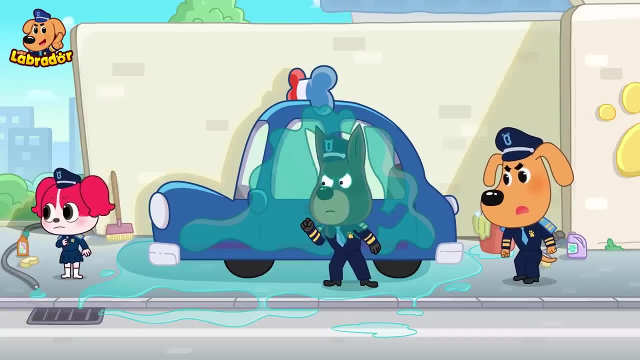 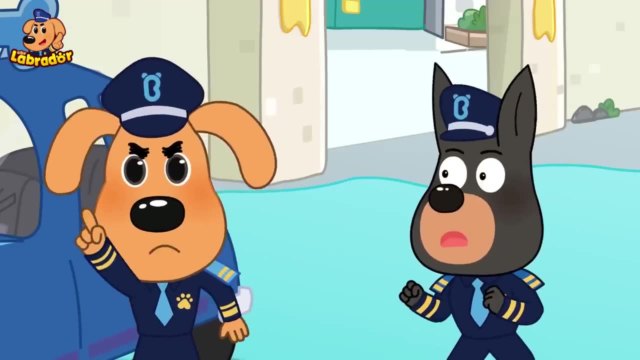 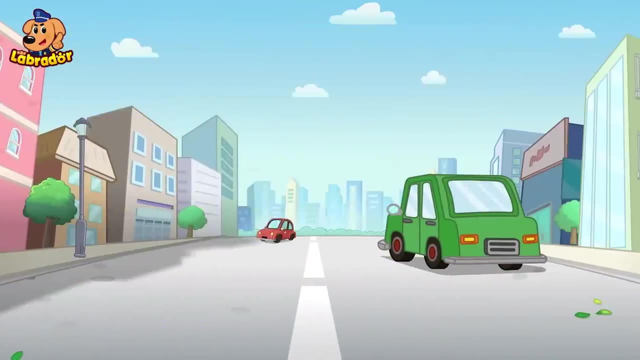 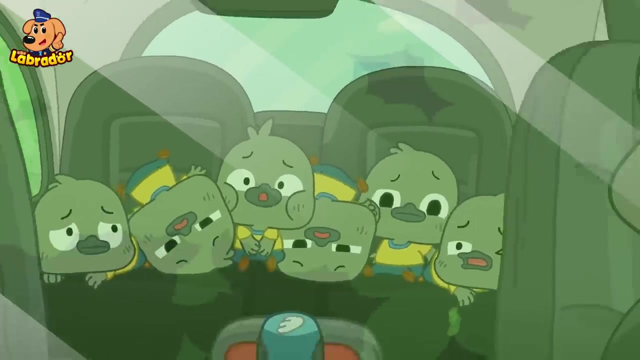 It's dirty again. Hey, You should drive safe with manners. Looks like something's wrong with that car. Dobby, let's follow it. Huh, Papillon ready for backup, Got it? Don't push me, I need to fart again. 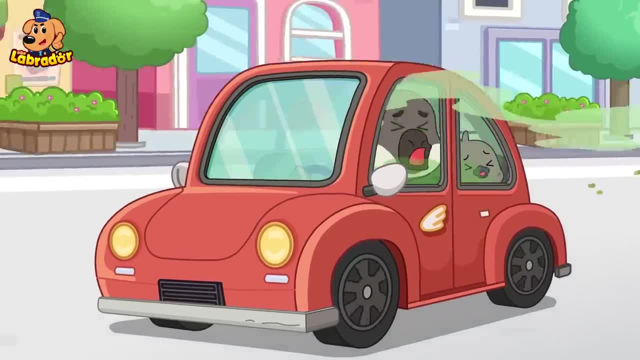 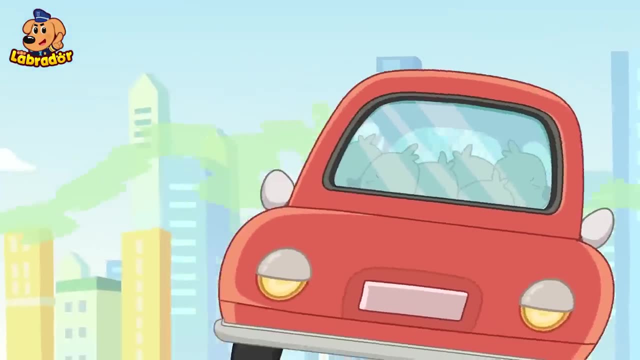 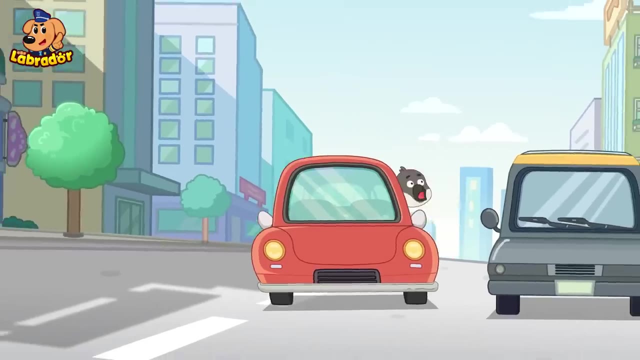 Let's open the window. Huh, Huh, Huh Huh. There are too many people in the car. That's so dangerous. We need to stop the car. Huh, Huh, Huh. Why am I on the main road? 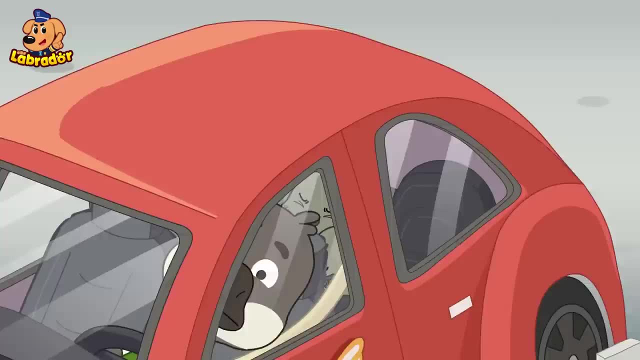 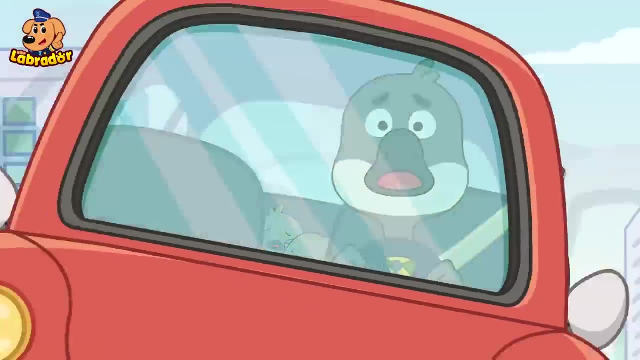 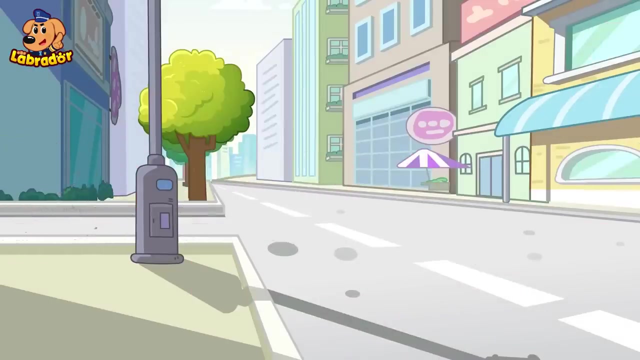 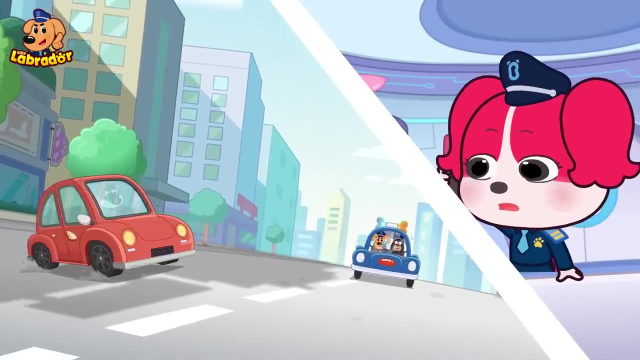 Huh, Oh, no, Watch out. Ah, Ah, Ah, Ah Ah, I can't control the car. Oh Ah, Whoa. Oh Ah, Watch out, Ah Ah, Papillon, Mr Wild Goose's car is out of control. 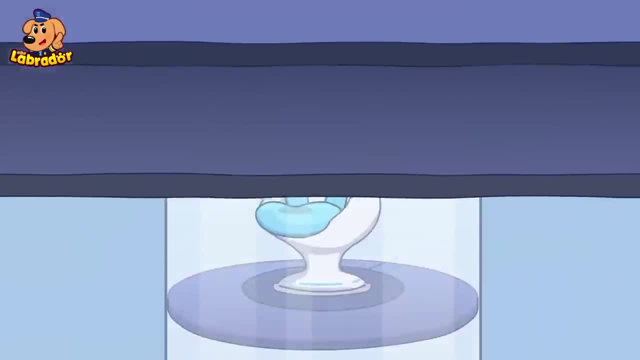 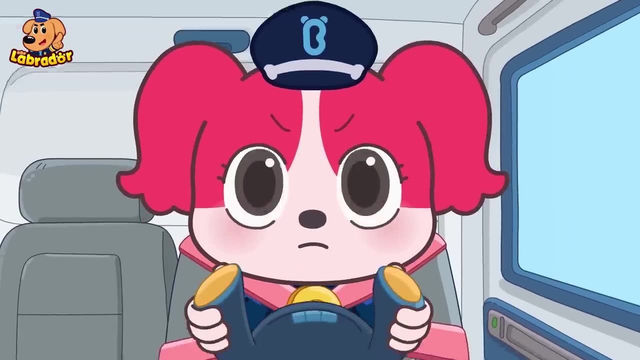 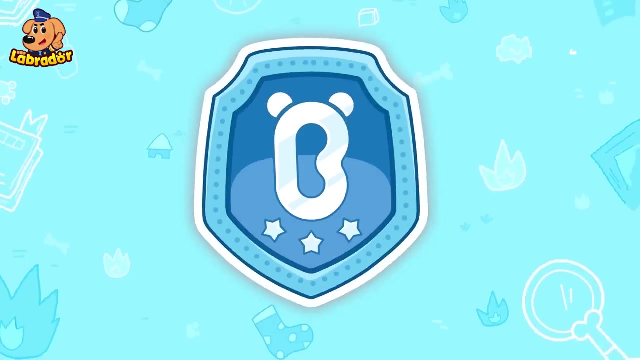 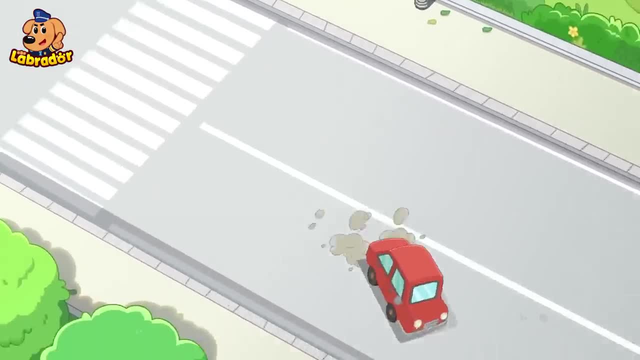 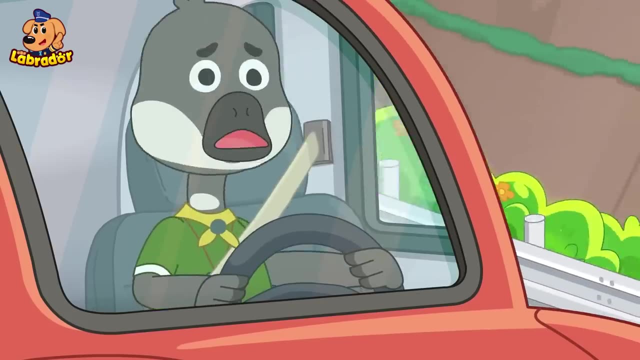 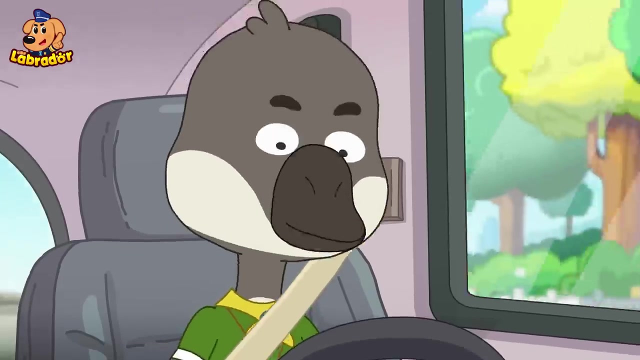 Ah, Ah, Ah, Ah, Ah Ah Ah. Oh, that was close, It was so scary. Huh, Huh, We're going downhill. I need to stop the car. Huh, The brake's not working. 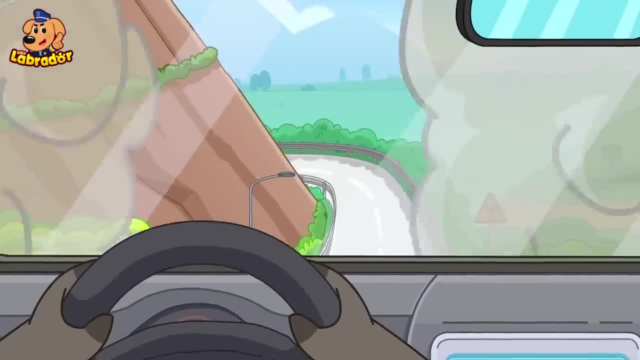 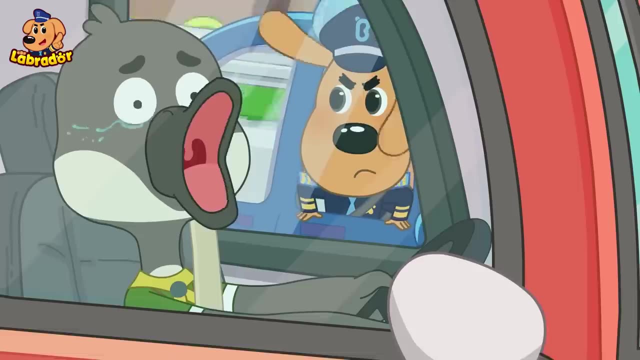 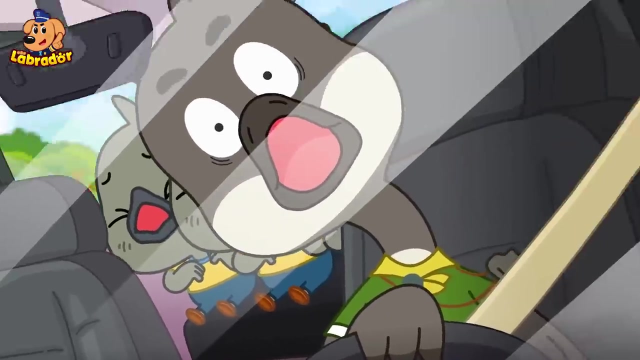 Ah, Huh, Ah. Why is there smoke coming out? Ah, Mr Wild Goose, stop the car. The brake's not working. Ah, It's so scary I want to go home. Ah, Huh, Oh. 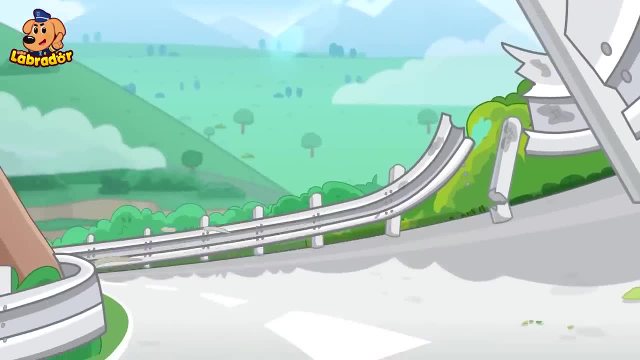 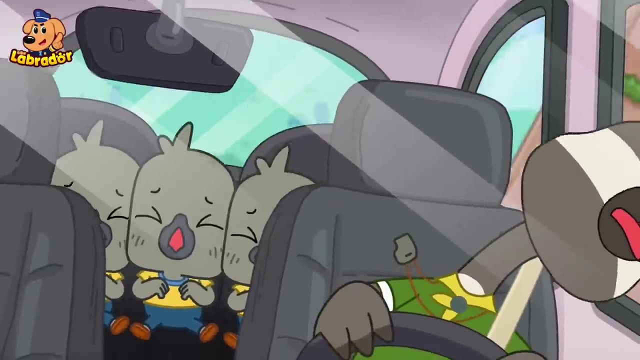 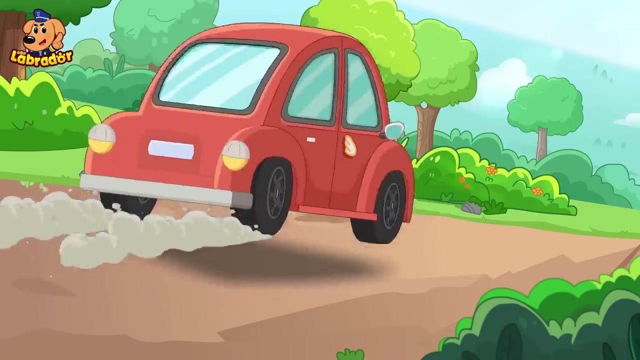 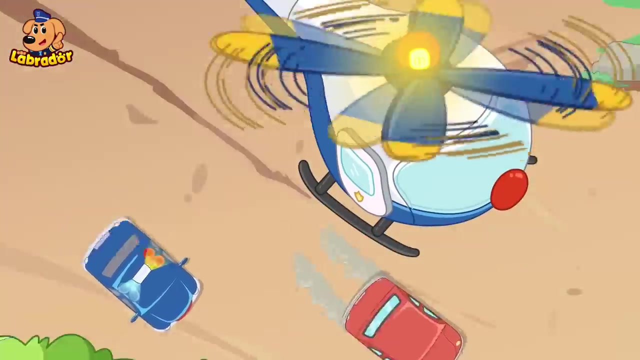 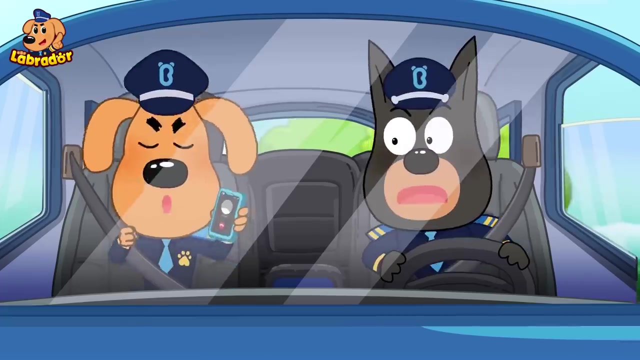 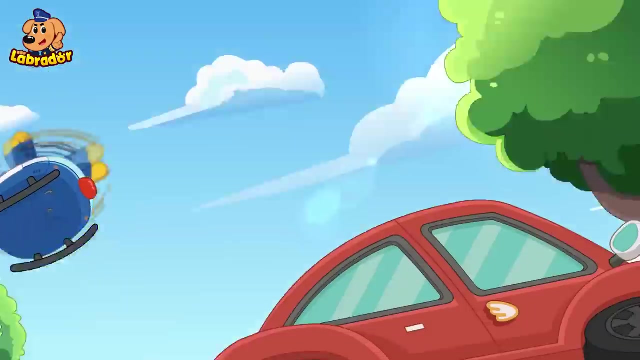 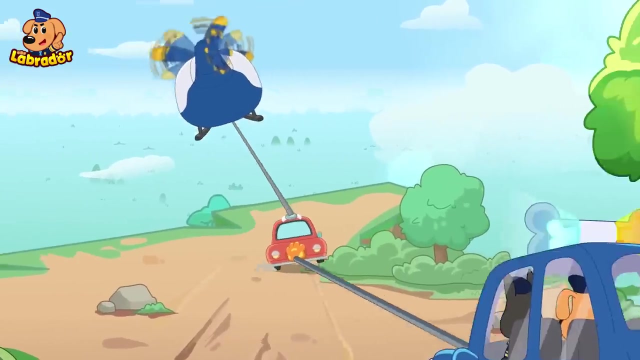 Ow, Help Papillon's here. Hihihi, Huh Huh. Sheriff Labrador, there's a cliff up ahead. What We need to stop the car right now Got it. Let's go. It's, it's a cliff. 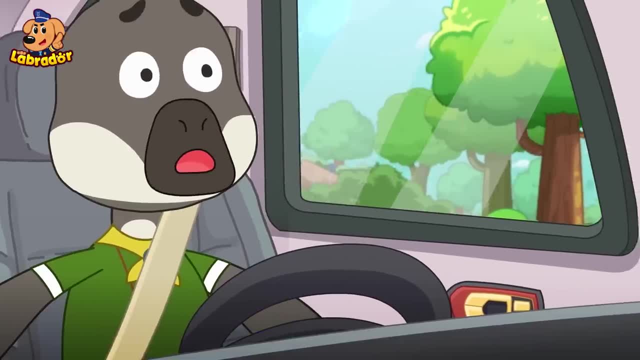 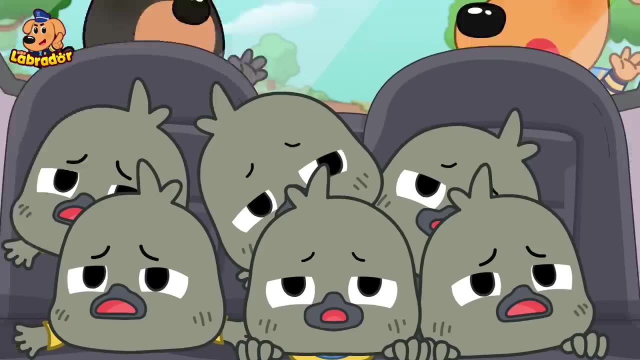 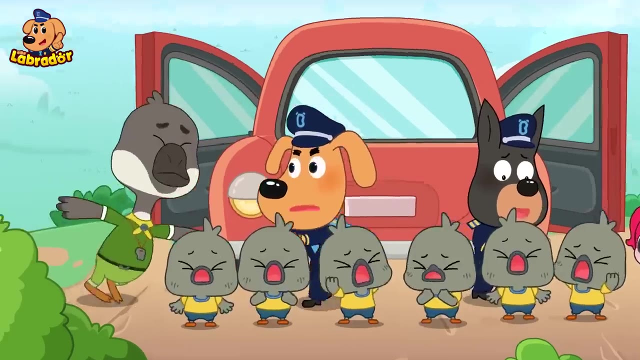 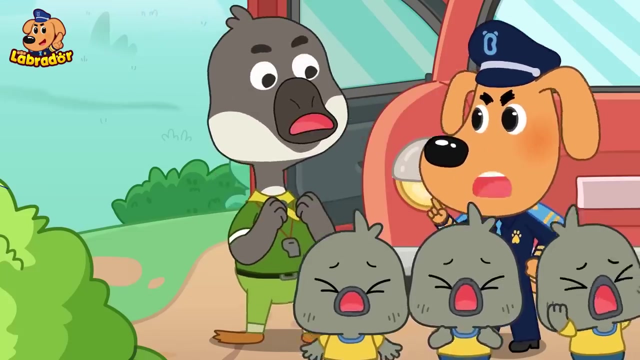 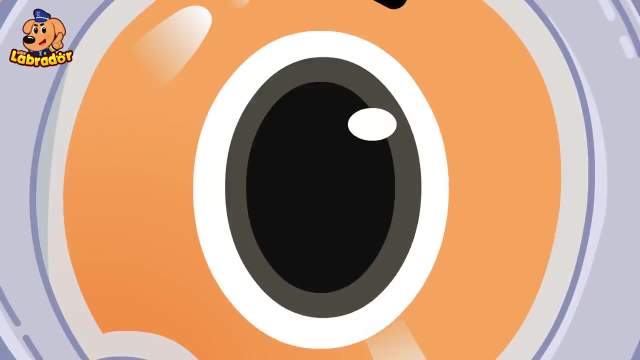 Phew, Everyone's safe. That was so scary. Thank you so much for saving us. Mr Wild Goose, you broke the traffic rules. You're coming with us to the police station. I'll never overload my car again. Sheriff Labrador's Safety Talk. 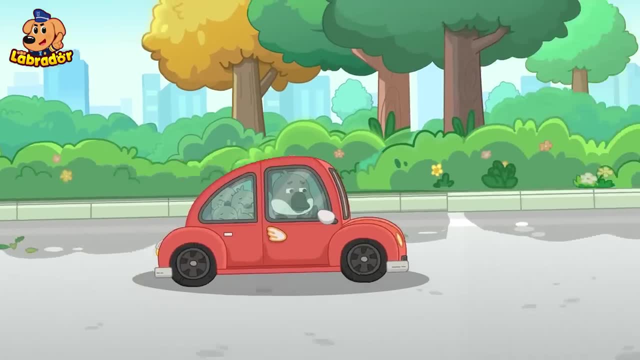 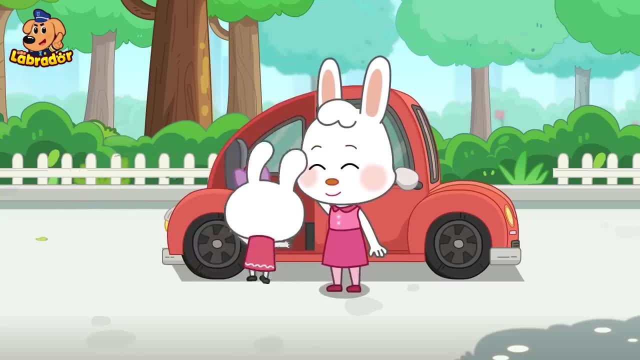 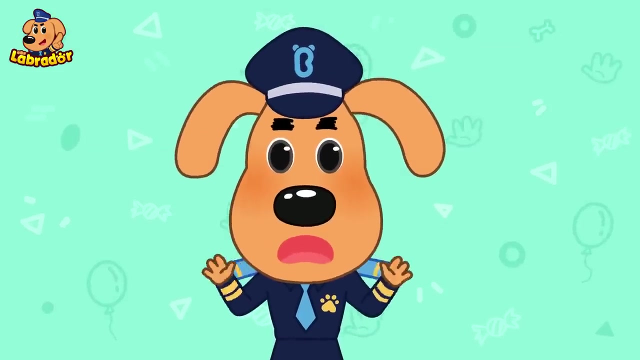 Kids. it's very dangerous to ride in a car that has more people than it was designed to seat. When riding in a car, kids should sit in safety seats in the back and fasten their seatbelts, And while riding, you should remain seated and keep your heads and arms inside the car. 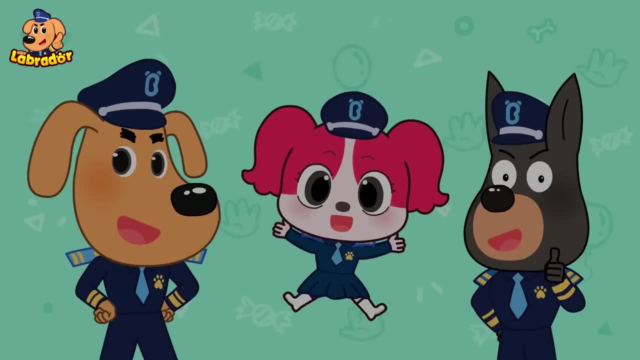 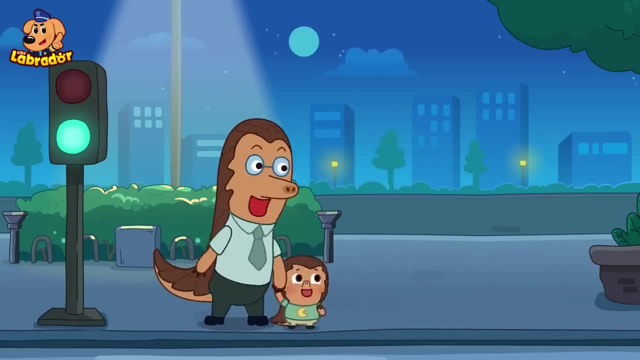 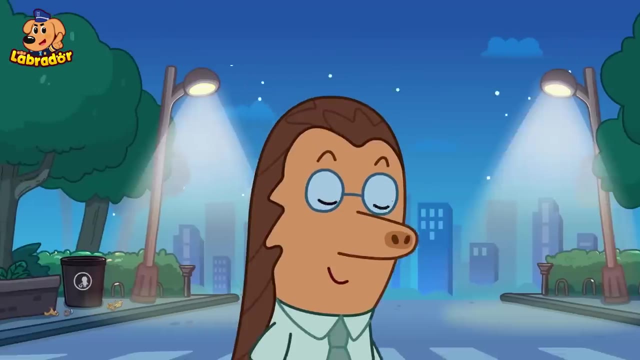 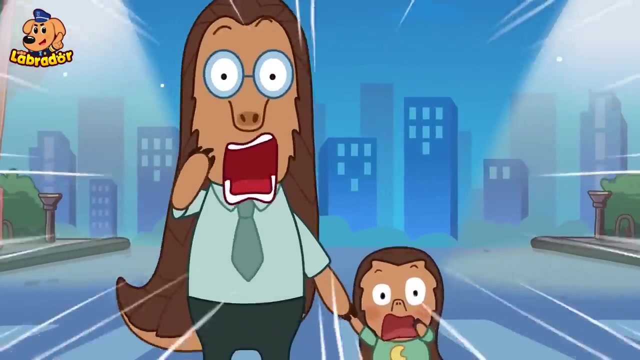 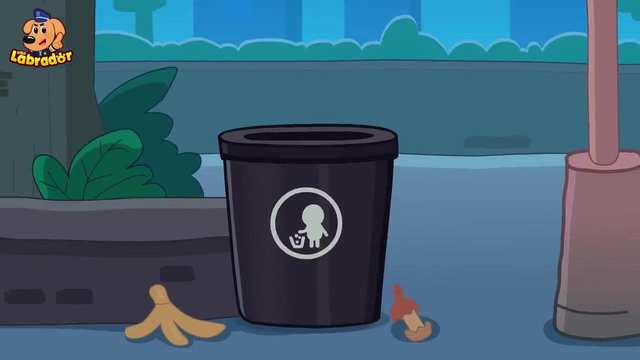 Please remember that Woof The Ghost Motorbike Green light. Stop at red, go at green. What's that? There's no one driving it. Ah Ow, Ah. I'm sorry, I didn't mean to hit you. 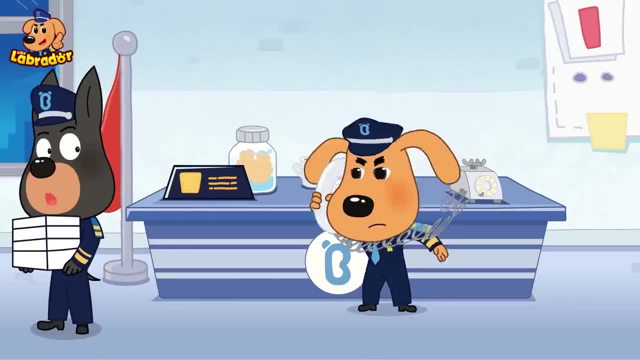 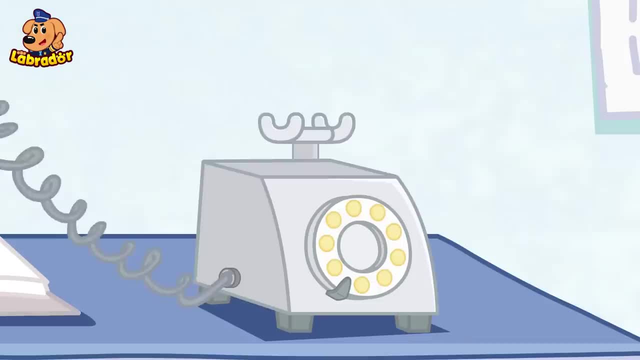 I'm sorry, I didn't mean to hit you. Woof, Hi, I'm Sheriff Labrador. Sheriff Labrador, I got hit by a Ghost Motorbike when I crossed the street just now. What A Ghost Motorbike. We'll be right there. 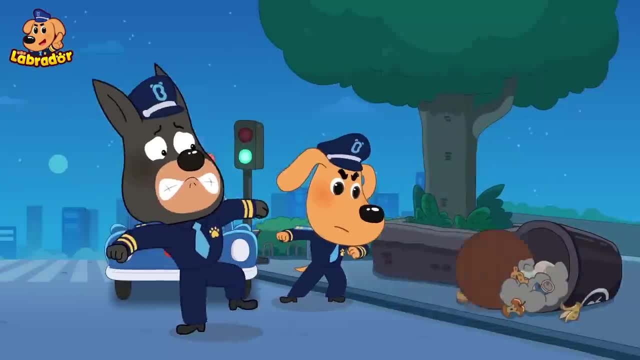 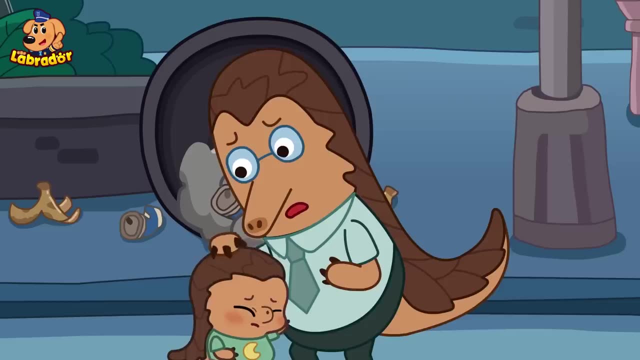 Where is he? I'm here, I'm here, I'm here. What? Ah? Ah, That was close. That was close. We're lucky to have hard scales. Mr Pangolin, you called the police, right? Oh yes. 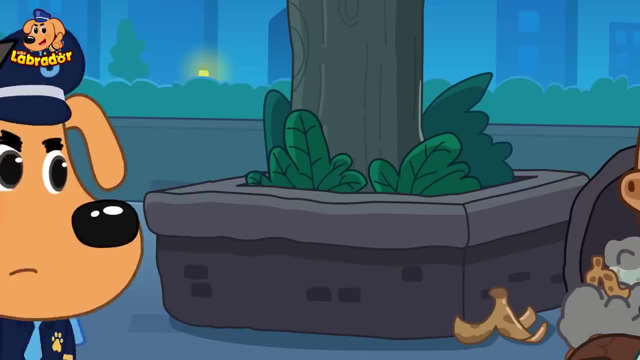 I got hit by a motorbike running a red light And you know what? There was no driver. It must have been a Ghost Motorbike. Ah, I'm so scared, I'm so scared, Oh no, I'm so scared. 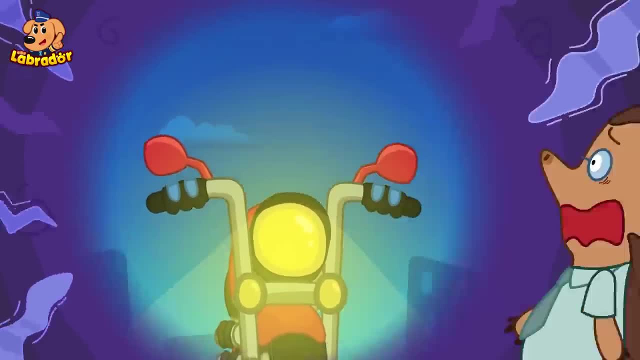 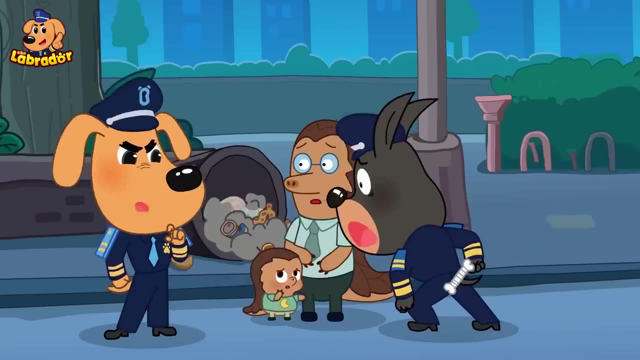 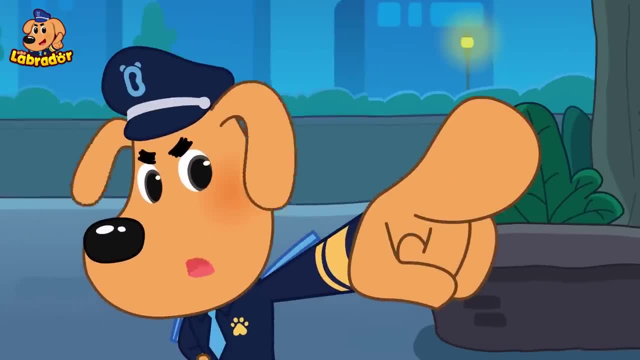 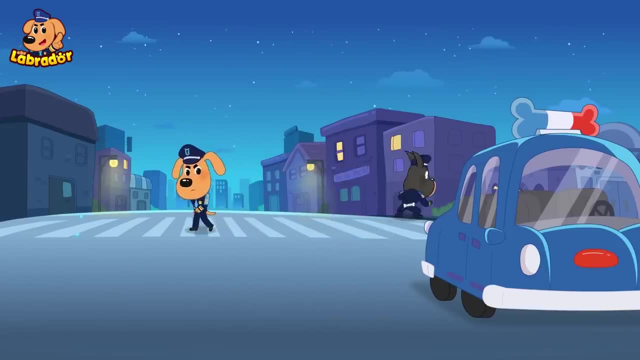 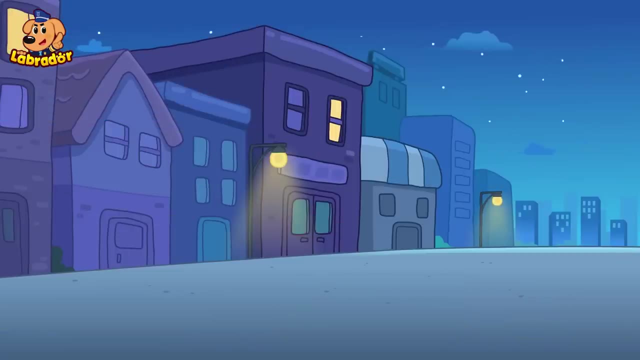 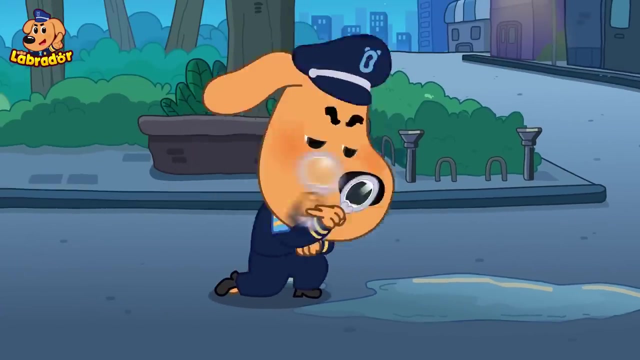 Don't worry, There's no case that I can't solve Now. let's find the motorbike first. Got it? Every vehicle leaves a mark when it passes by. It's a puddle. Hmm, Hmm. these are cars' tire tracks. 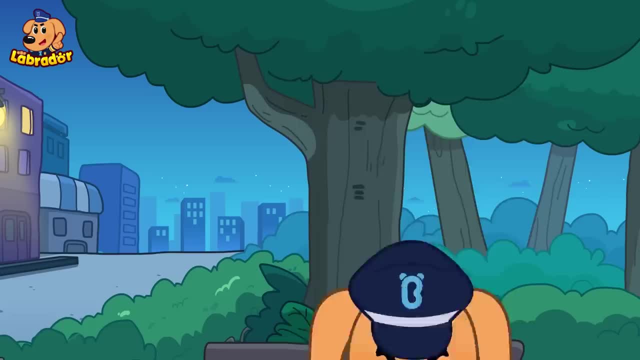 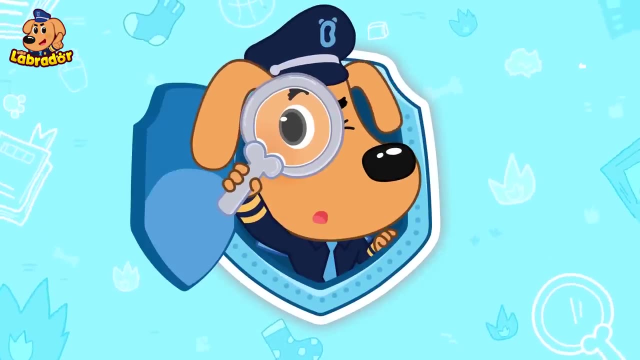 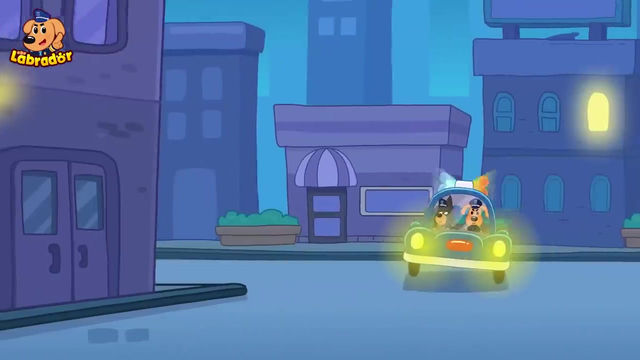 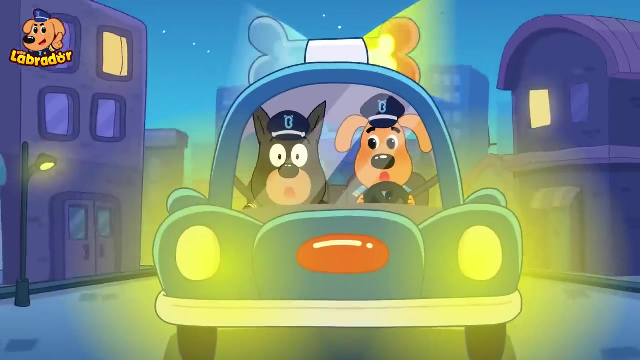 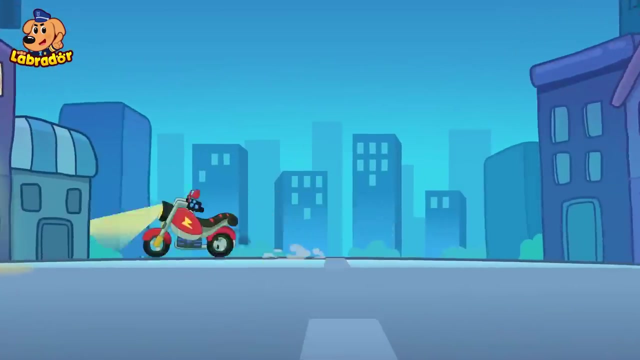 And these are motorbikes' tire tracks. I found the clue. It must have gone this way. Woof, Let's go Look over there. It can't be. Is it a real ghost? There's no such thing as a ghost. 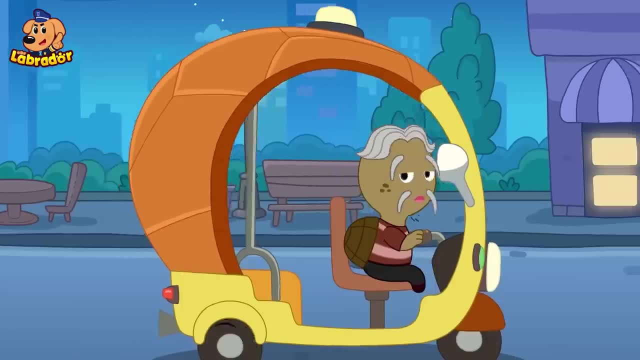 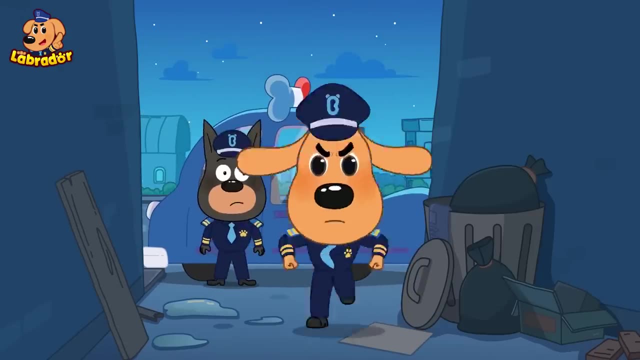 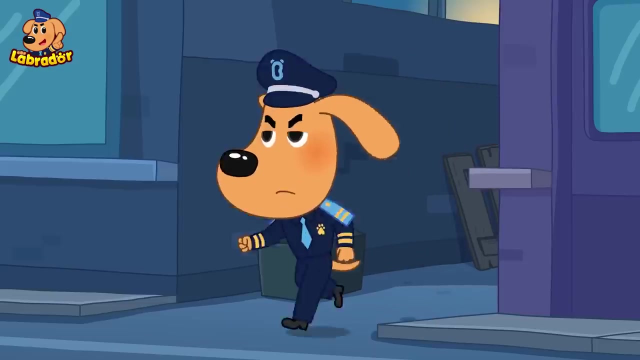 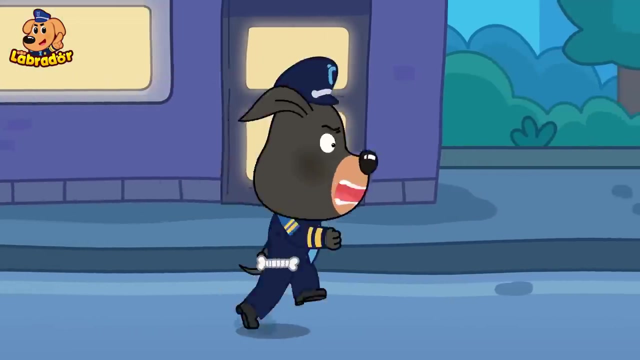 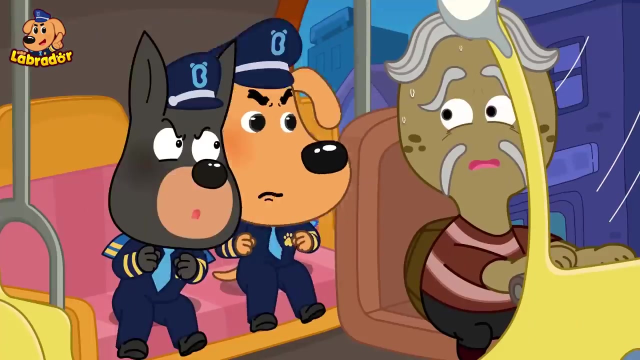 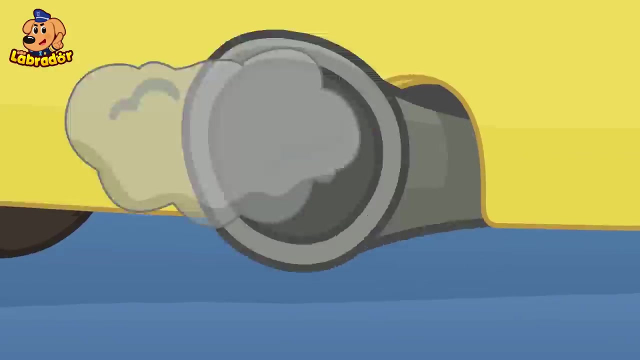 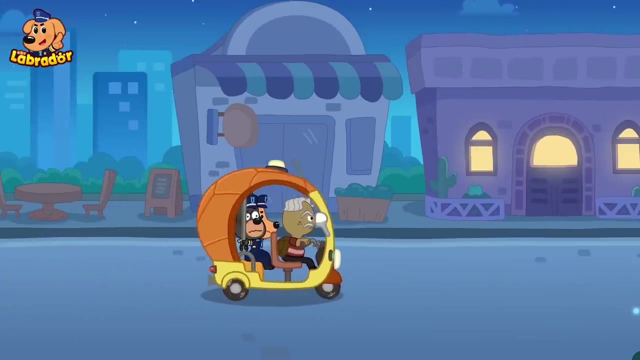 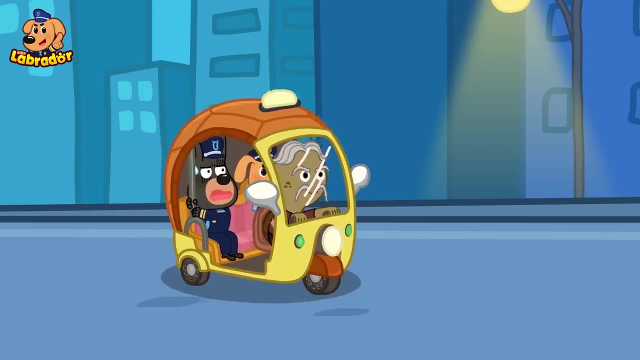 There Into the alley, Hurry up, Huh, Oh no, It won't go far. Police, Mr Turtle, Can you help us follow the motorbike over there? Sure, Hold on tight, Mr Turtle, Are you sure you can catch it? 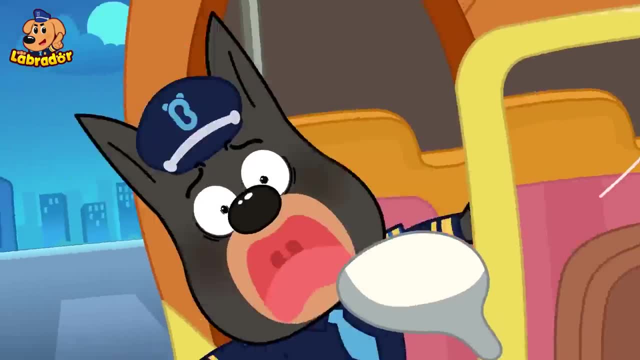 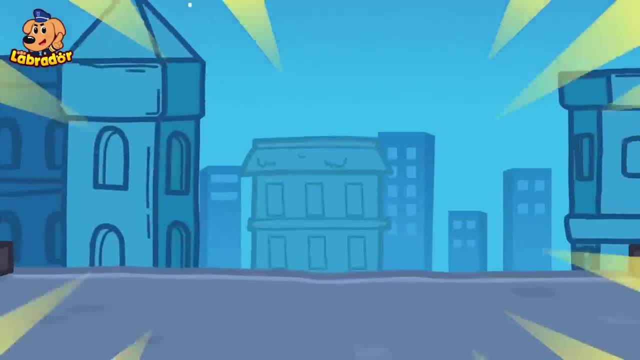 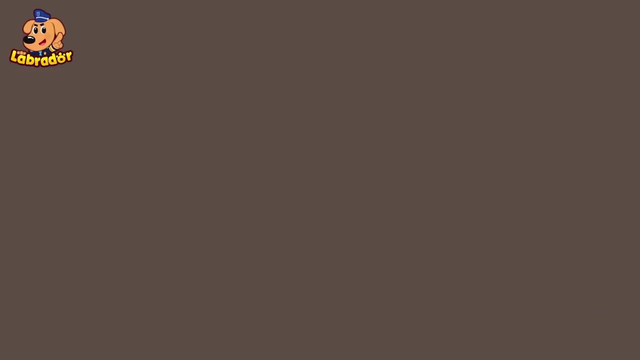 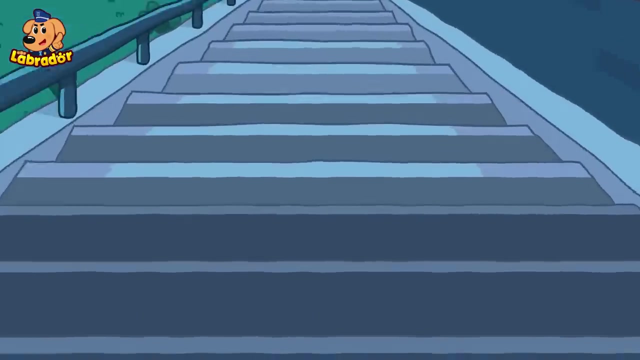 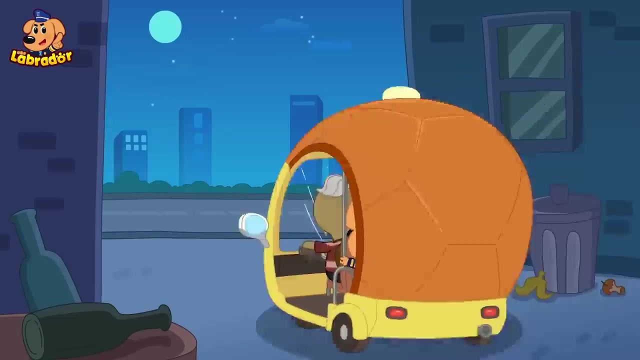 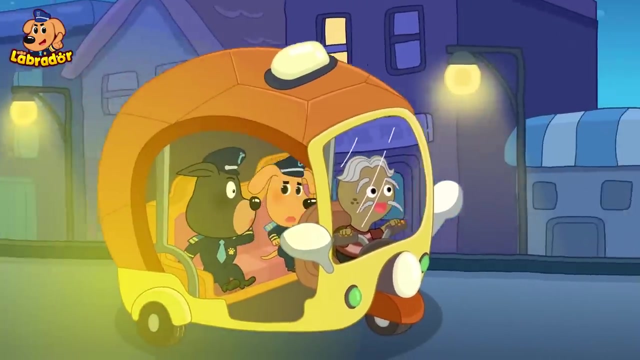 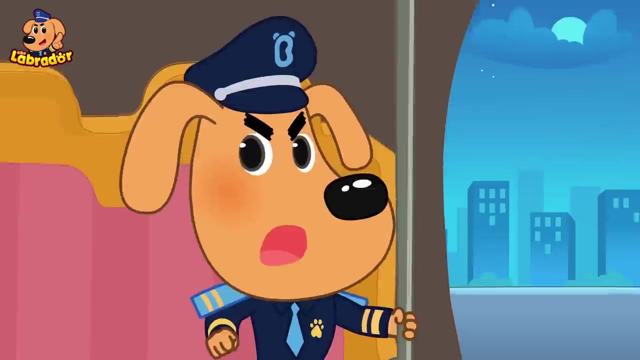 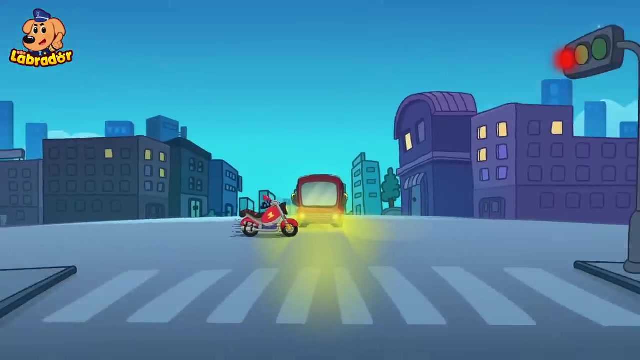 Of course Go, Let's go. Ah, Ah, Ah, Ah, Ah, My bottom really hurts Huh. Where are we? Huh? Ah, The ghost motorbike, Huh, Stop, Huh, Ah. 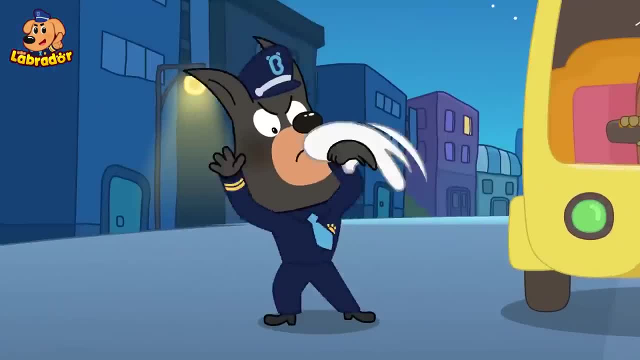 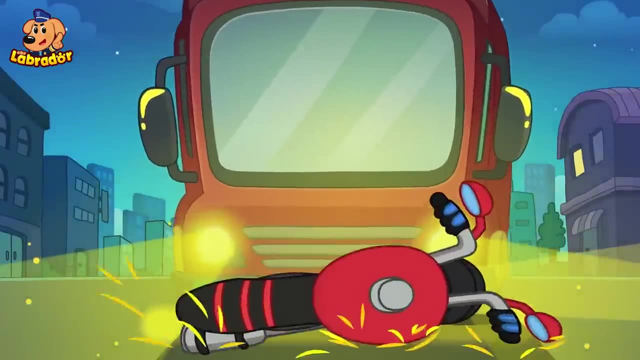 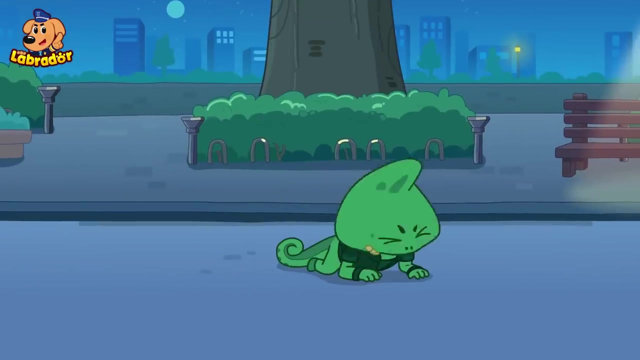 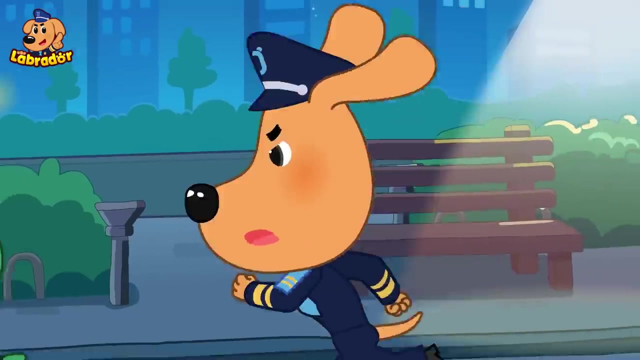 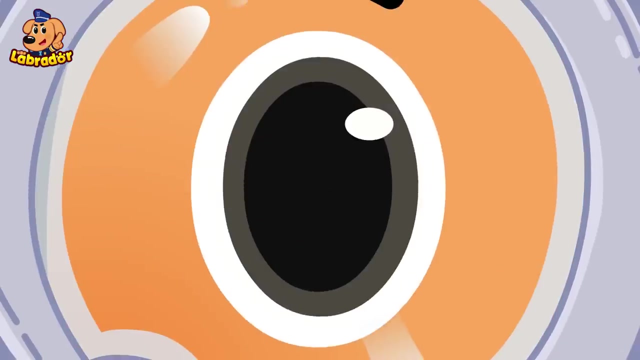 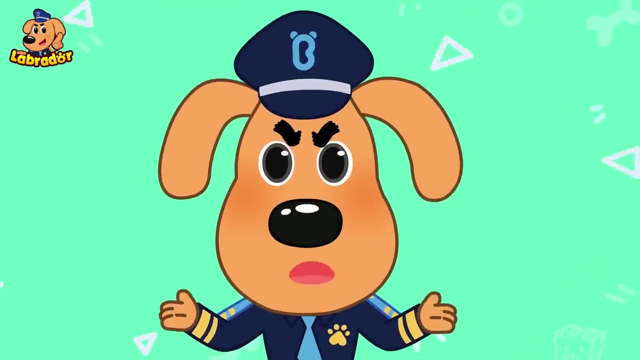 It's a chameleon. Watch out, Ah Ah Ah. I was really scared, Chameleon. You broke the traffic rules. You're under arrest. Sheriff Labrador's Safety Talk Kids. Traffic lights are the signals to control traffic. 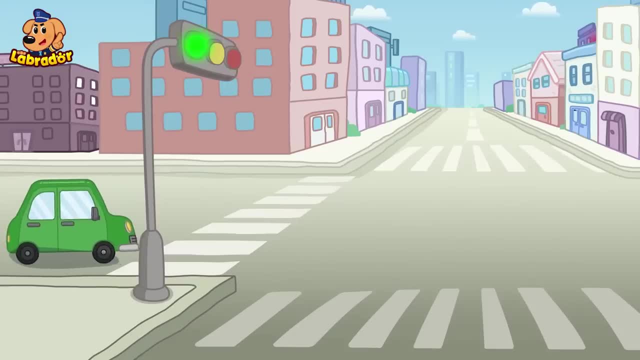 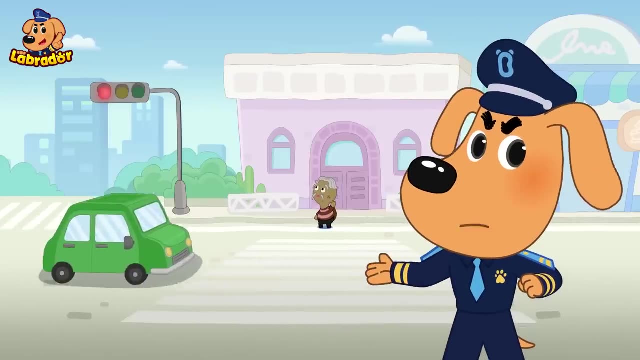 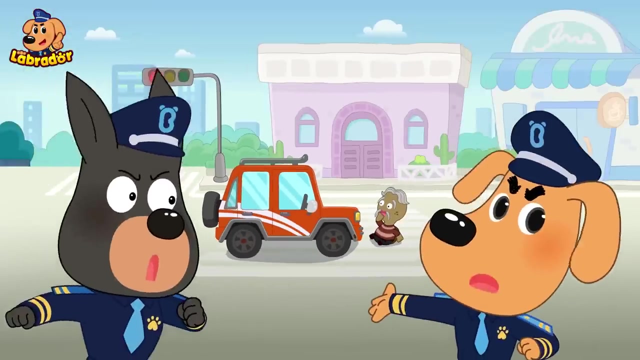 The red light means stop, The green light means go And the yellow light means be careful. Whether you're a driver or a pedestrian, you should always follow the traffic lights. If you don't, you might get in a traffic accident. Please keep that in mind. 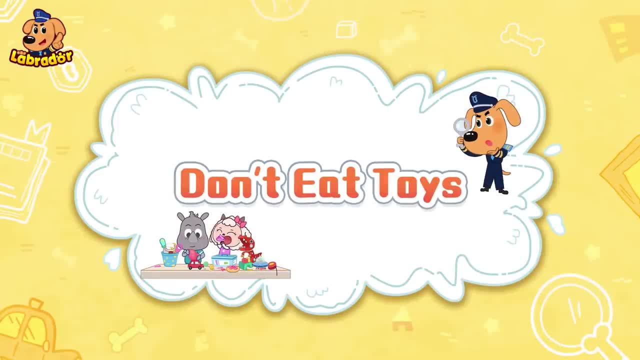 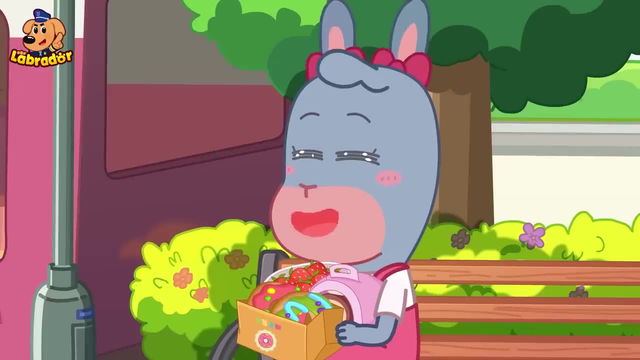 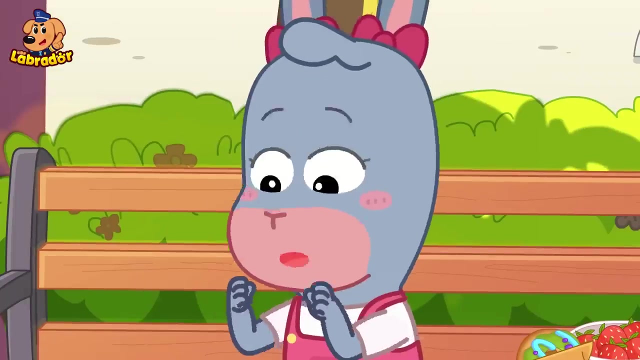 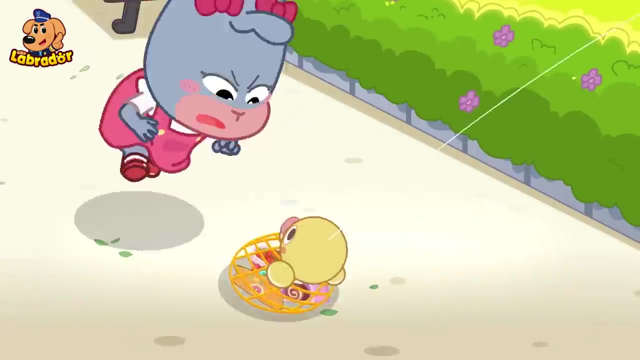 Woof, Don't eat toys. I bought a lot of yummy food. Wow, Where's my doughnut? Oh no, My strawberries and cake. Ouch, It's so yummy. It was you. Hey, Give it back, Ouch. 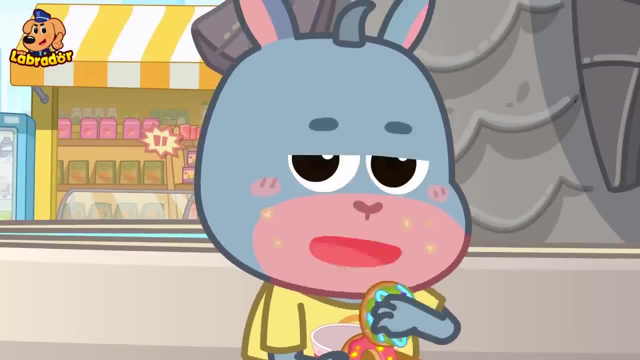 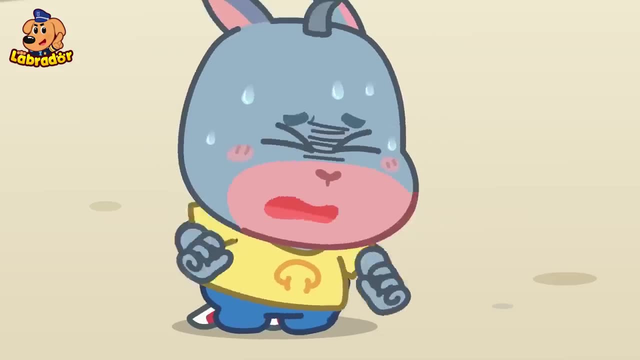 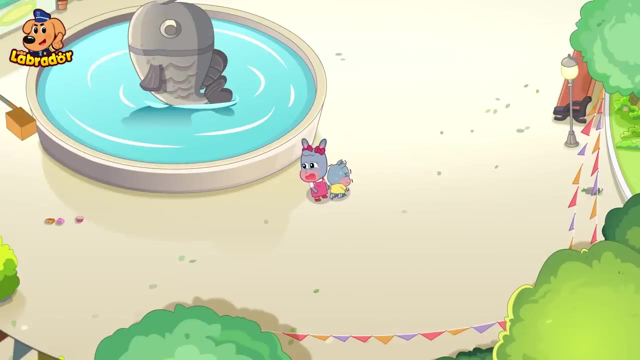 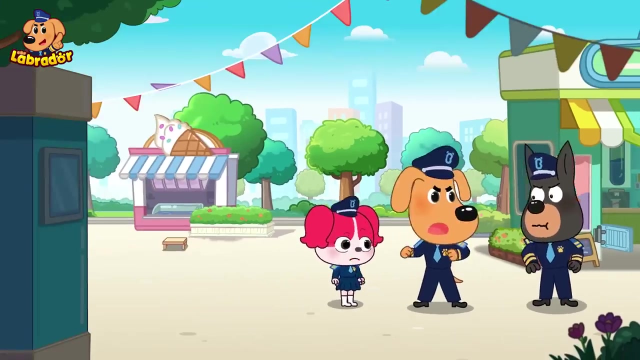 My tummy hurts. What's wrong? Get your tantrums, Ah Ah, Not again, Are you OK? What's wrong? Help Somebody, help us. Something's wrong over there. Let's have a look. What's wrong, little donkey. 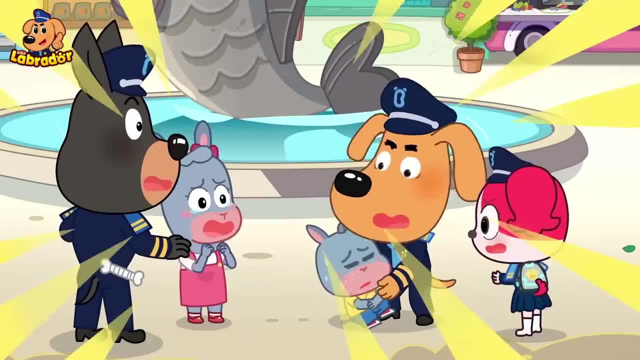 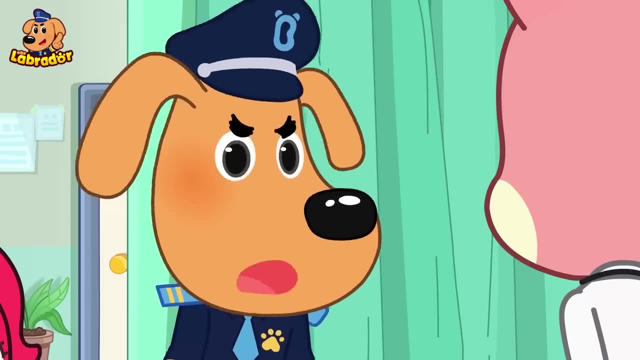 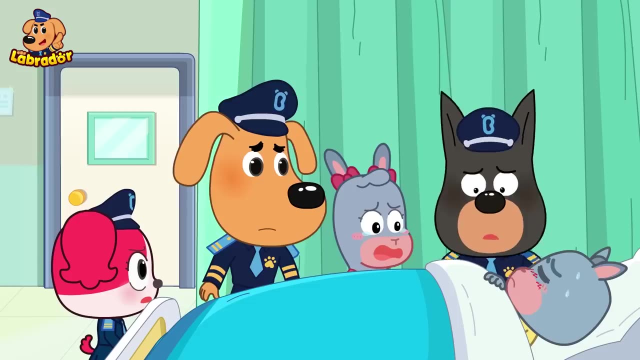 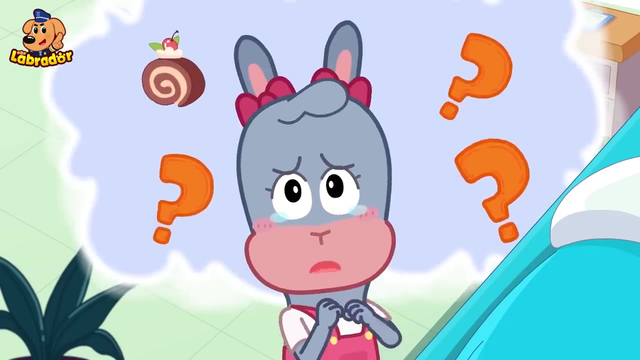 My tummy hurts. Hurry, take him to the hospital. Got it, Doctor Deer? why does he have a stomach ache? Seems like he ate something poisonous. What, Sister Donkey? what did your brother just eat? Um, he ate what I bought: A cake, strawberries and donuts. 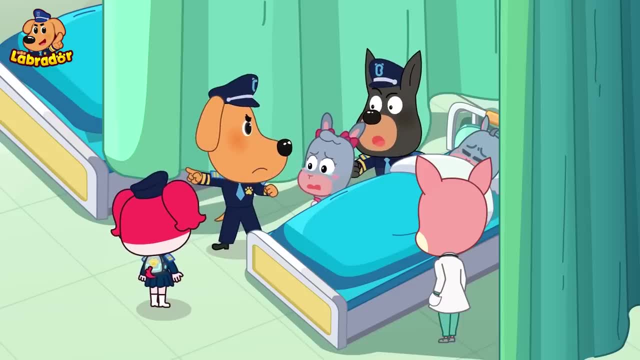 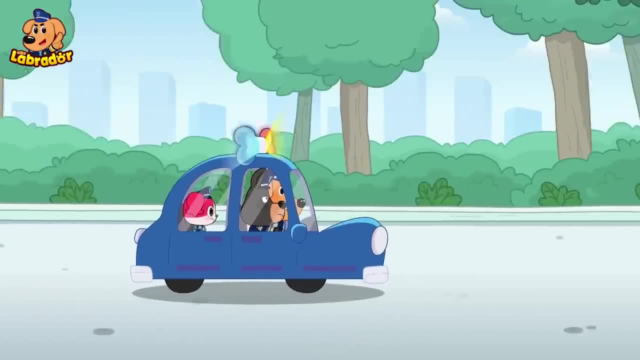 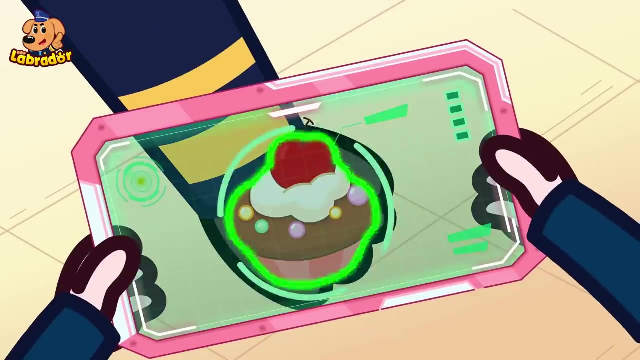 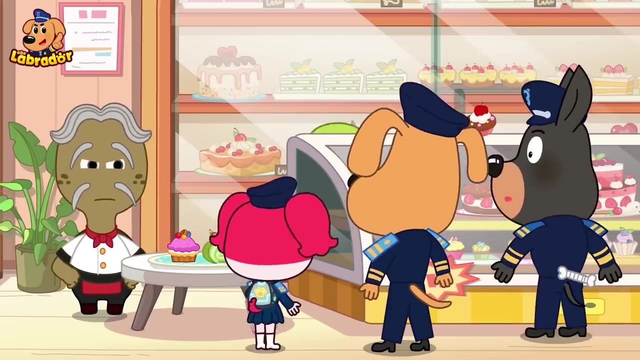 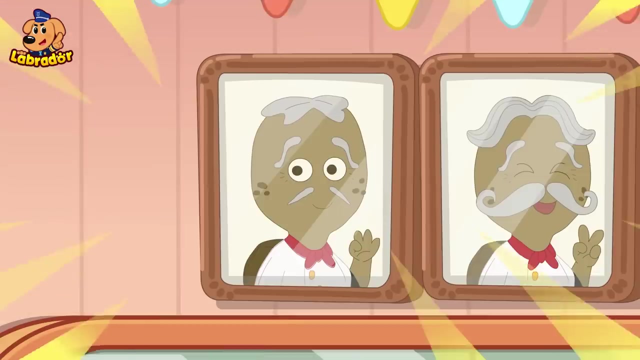 Papio Dobby, let's investigate these shops. Got it? The cake is fine. I told you my cake is fine. Our cake shop is a hundred years old. Since my grandpa's grandpa's grandpa's time there has not been a problem. 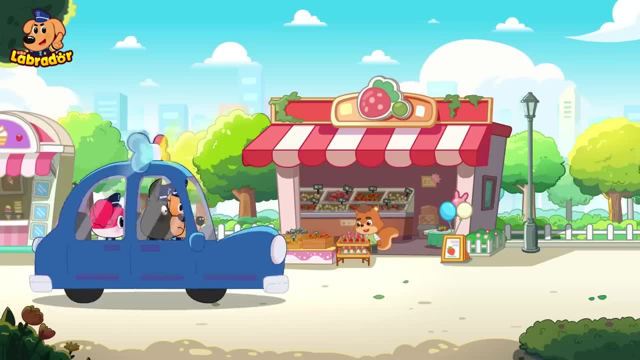 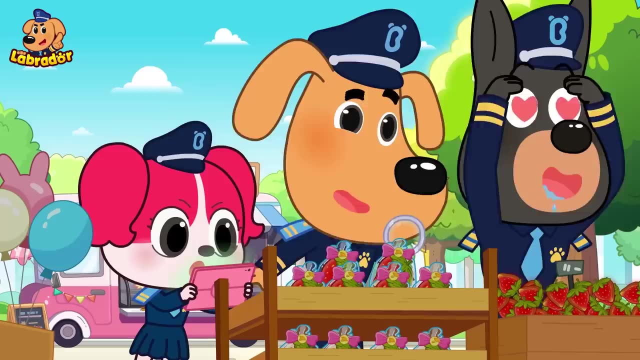 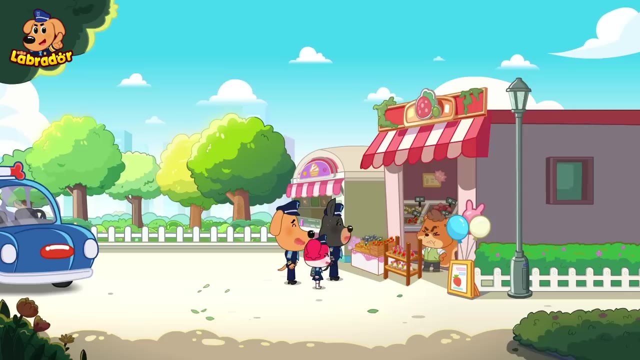 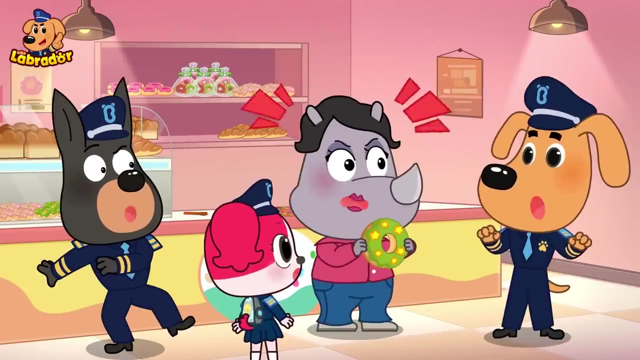 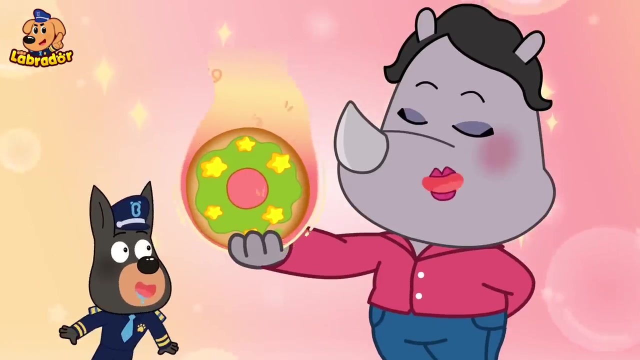 Sorry for bothering you. Uh, My strawberries are freshly picked. They're all fine, Even my own child is eating them. Sorry for bothering you. Oh, how could there be a problem with my donuts? Look The vibrant colors. Ah, smell the tempting fragrance. 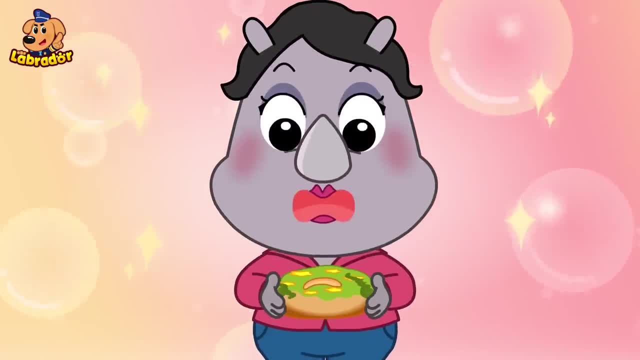 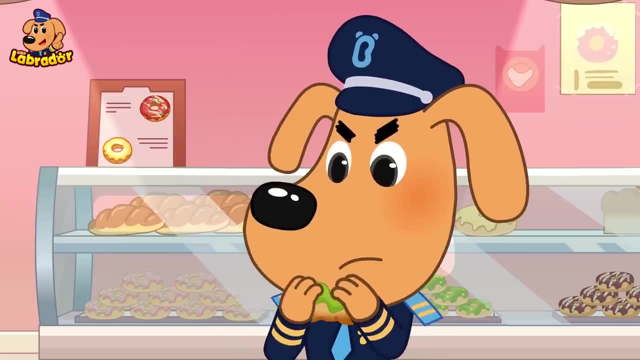 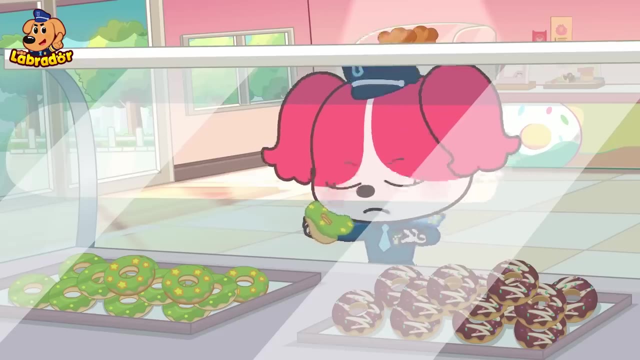 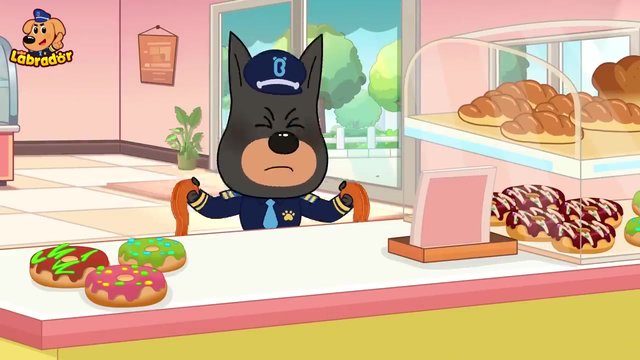 And touch the soft texture. Oh aww, strange. This is not a donut I made, It's clay Clay. The donuts here are made of clay too. Same here: Even the bread tongs are made of clay. 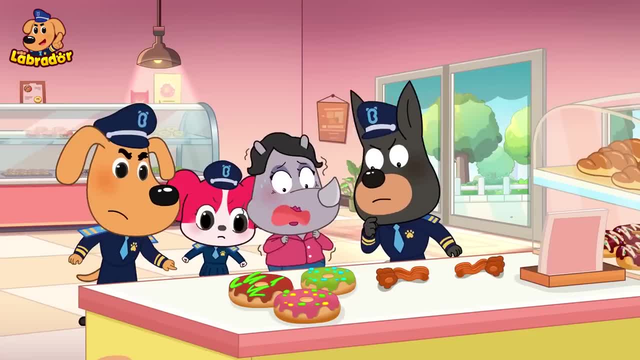 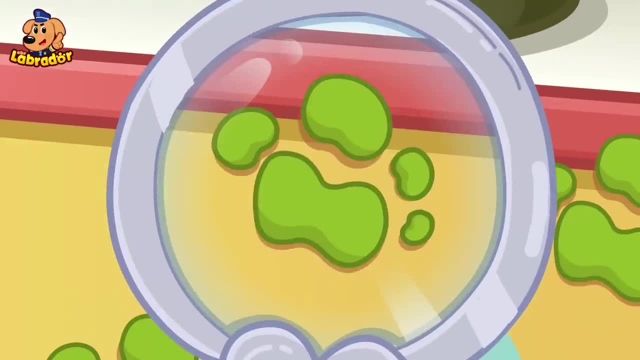 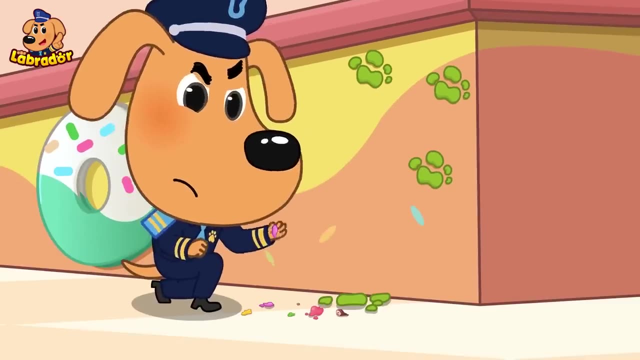 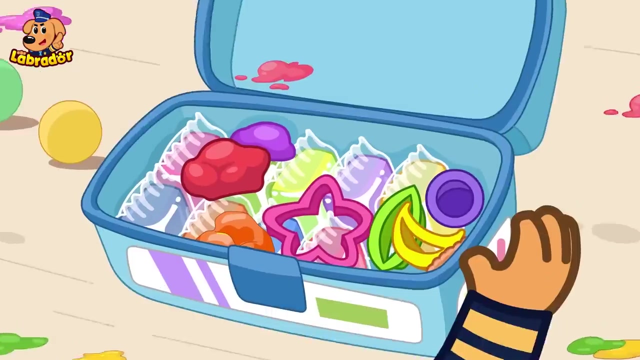 It seems that little donkey ate donuts made of clay. How could this happen? Uh-huh, It's a child's handprint. Uh No, this is my son's table. Why is there so much clay? It seems that little rhino made those clay donuts. 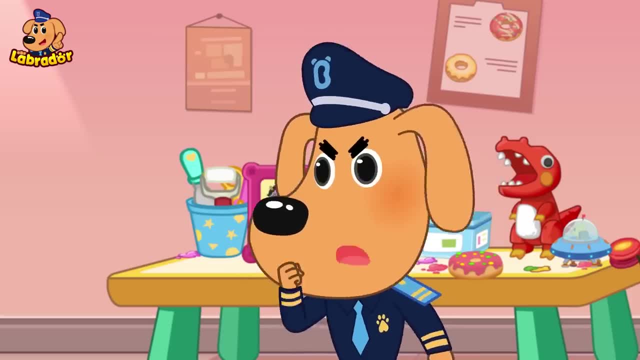 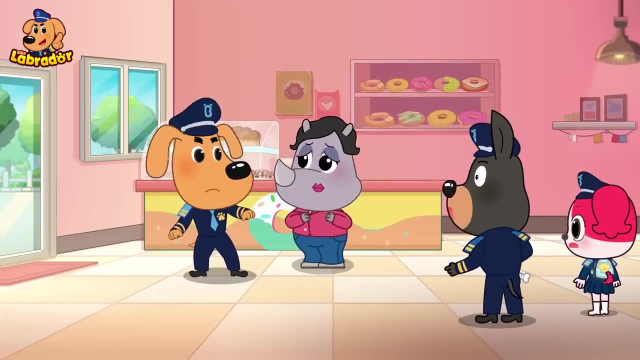 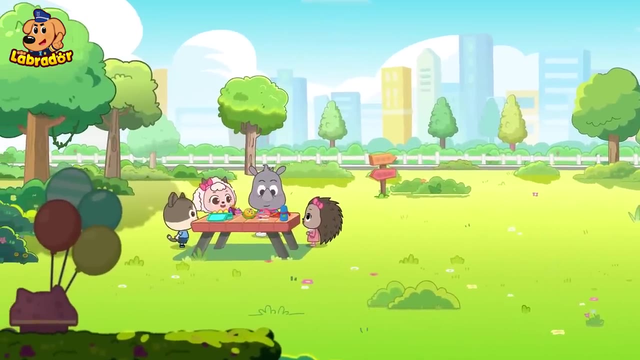 What, Miss Rhino? Do you know where he is? He went to the park. He said he was going to share some food with his friends. Share some food? Oh no, Oh no, Let's go find him All done. 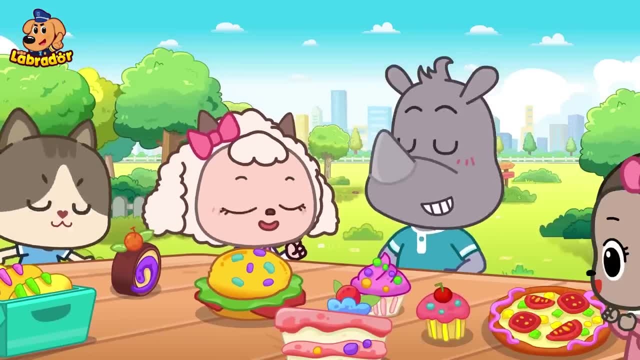 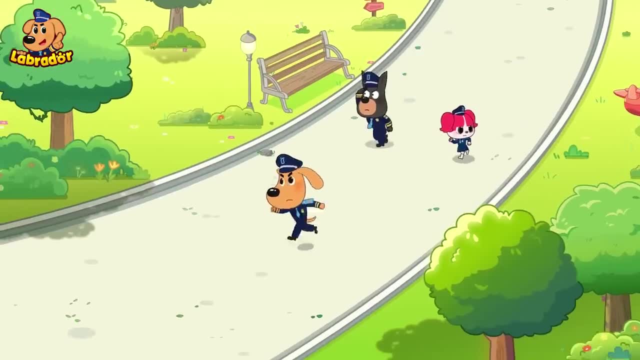 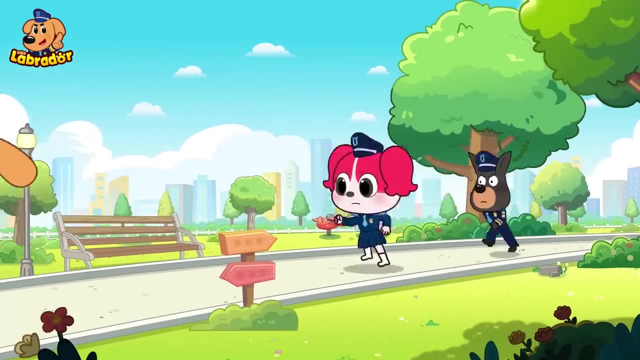 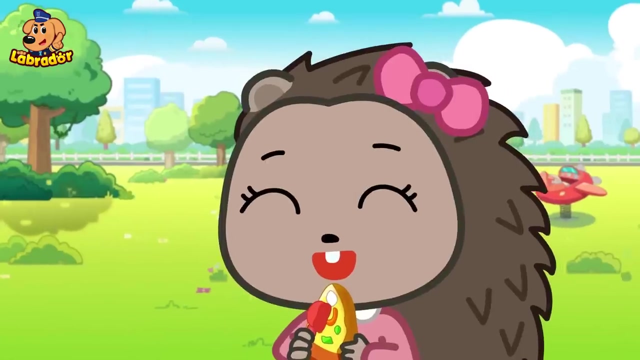 Wow, It looks real Little Rhino. this is awesome. It looks so yummy I want to try it. He's not here. Not here either. Wow, Let's start eating. Just one bite, Just a little. Don't eat it. 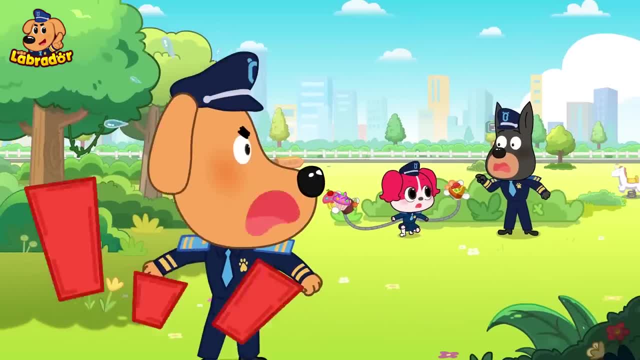 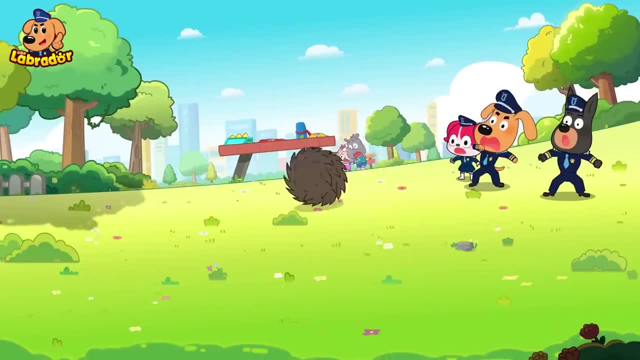 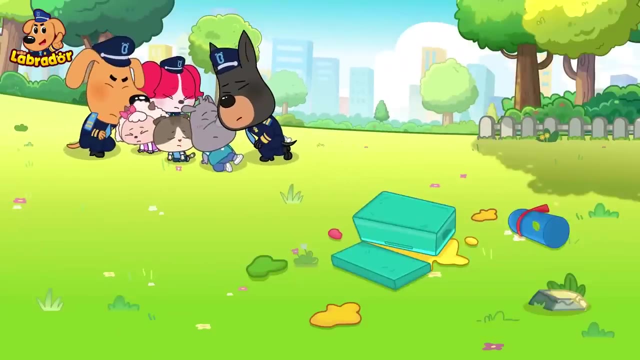 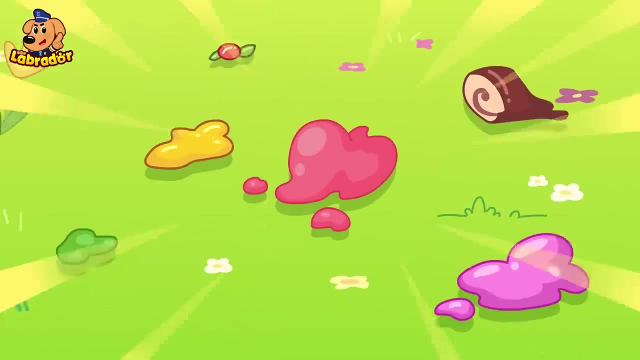 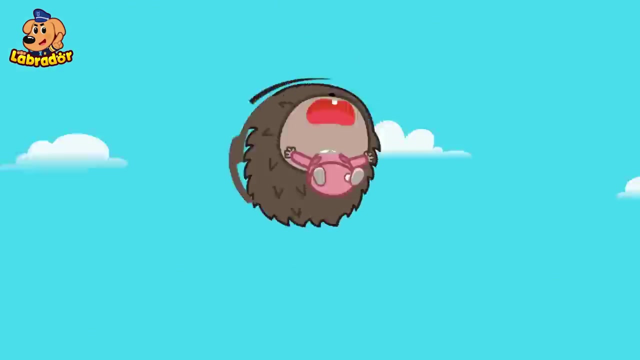 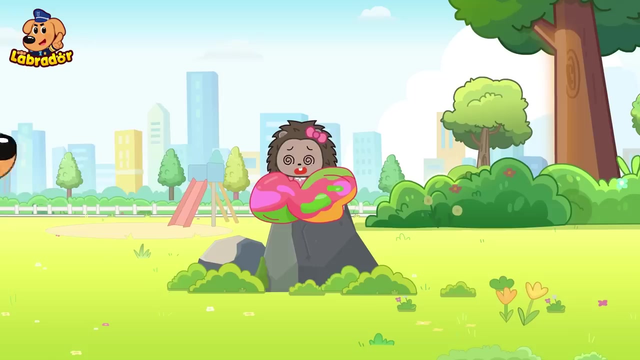 This one has a bite mark. Oh no, My tummy hurts. Little Hunchhunk, ate the clay. My tummy hurts so much. Watch out. Hey, Oh no, Hey, Hey, Oh no, Oh no. 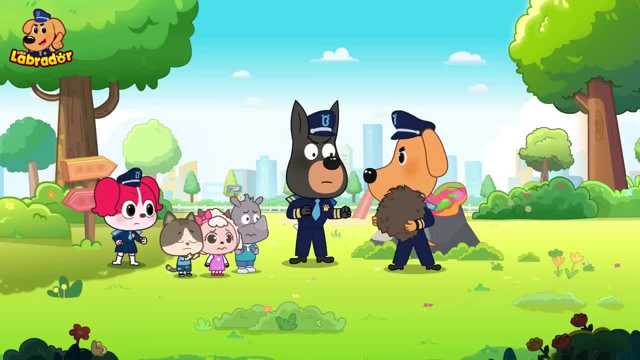 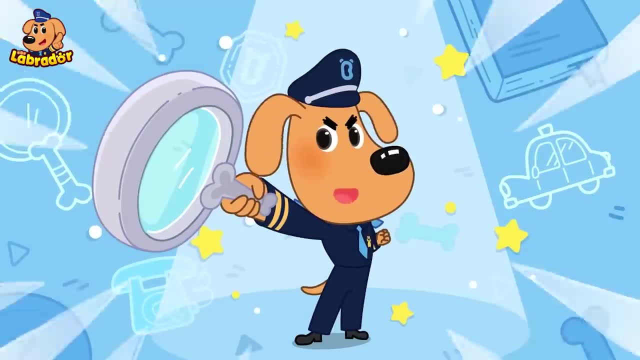 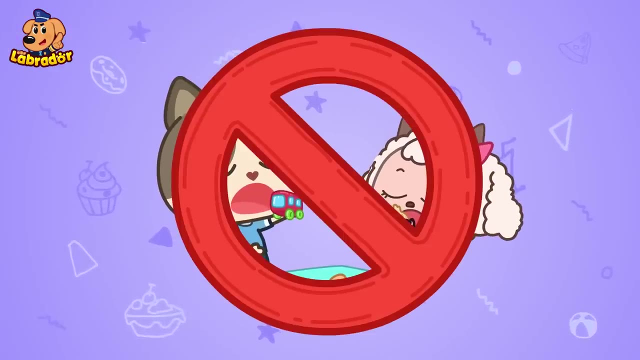 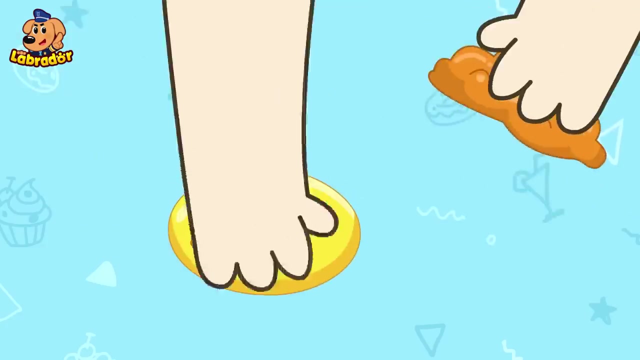 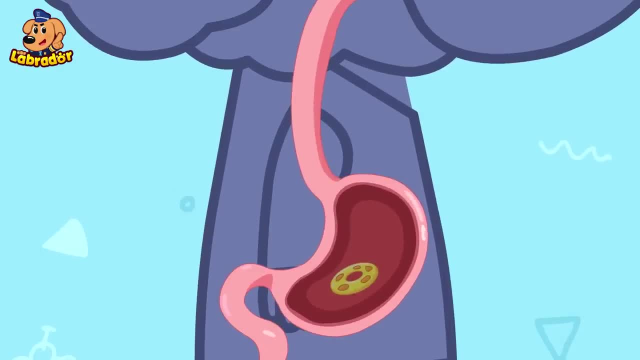 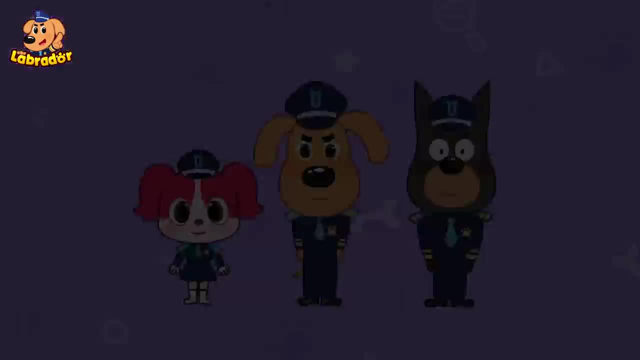 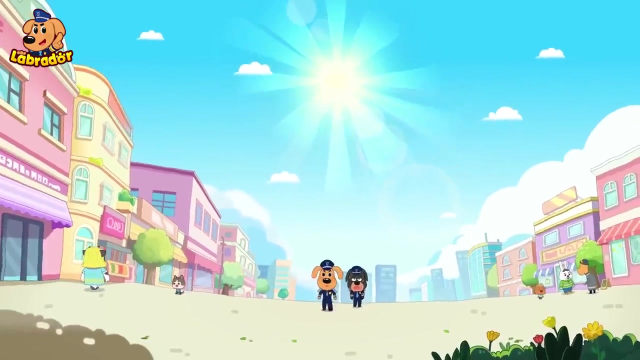 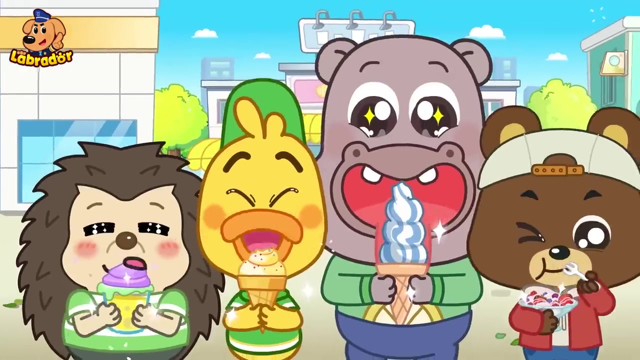 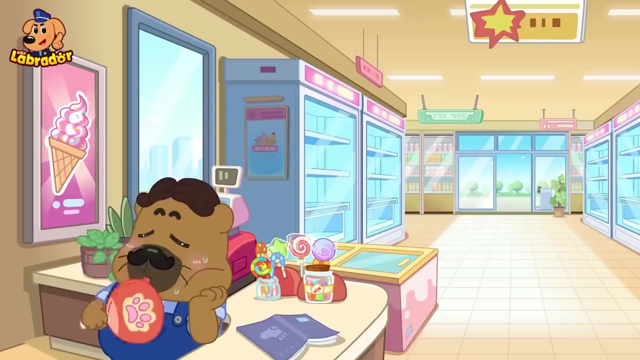 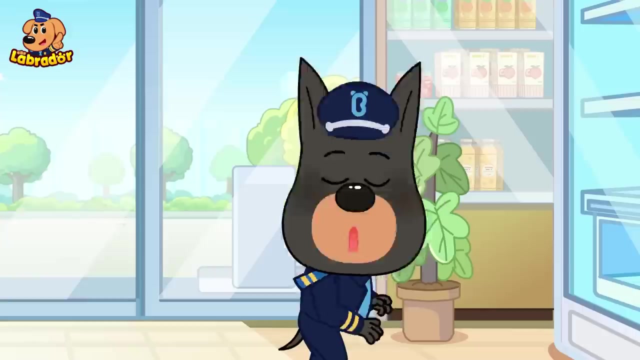 and some smell nice. eating them can cause stomach aches or even poisoning. Can you remember that? Don't eat too many cold treats. It's so hot. Wow, Ice cream, Ha, Hey, It's empty, Empty, Empty. 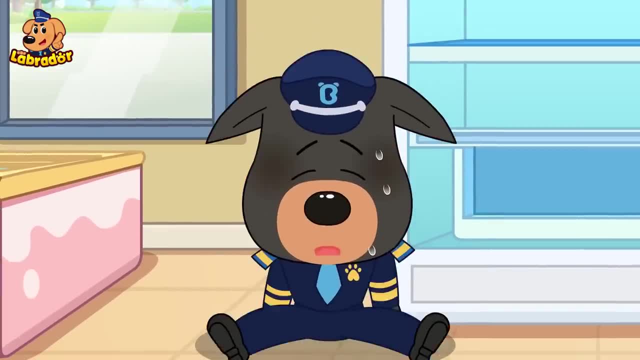 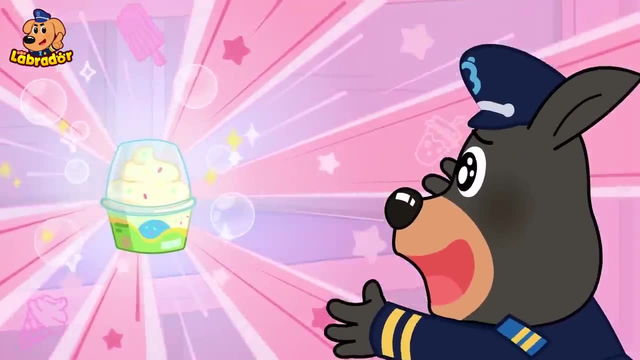 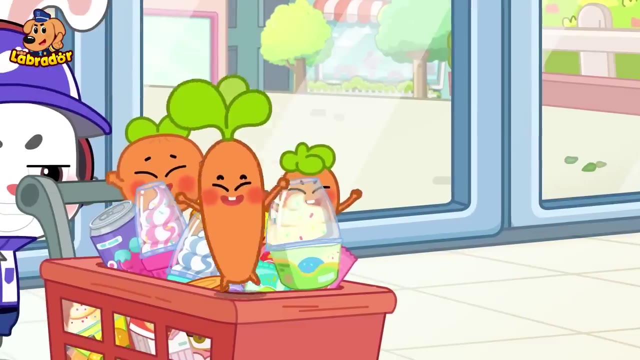 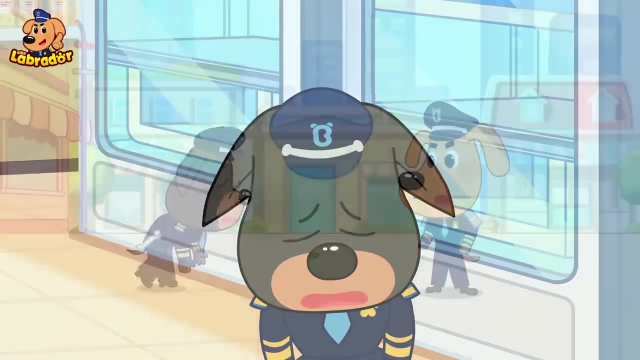 And empty. They're all empty. There's one left. Ha ha, ha, Ha ha ha. Buy them all. Buy them all. Ha ha ha, Sir, all of them please. Whoa, Oh, I couldn't even buy one. 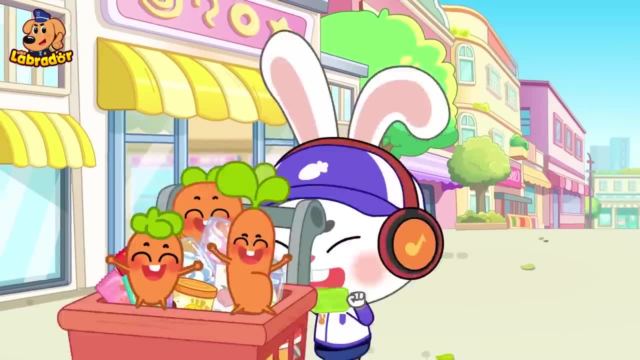 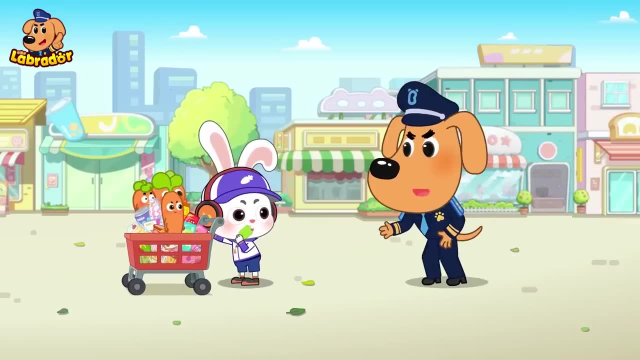 Peepy Rabbit bought all of them. Oh, Ha, ha, Fantastic, I'm going to eat them all. Peepy Rabbit, eating too much ice cream will make your tummy hurt. No, it won't. Ah, Bye-bye. 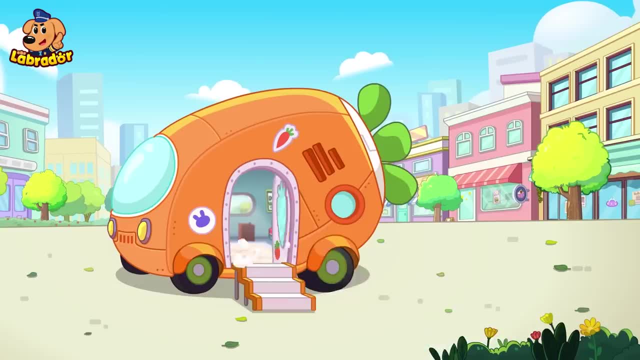 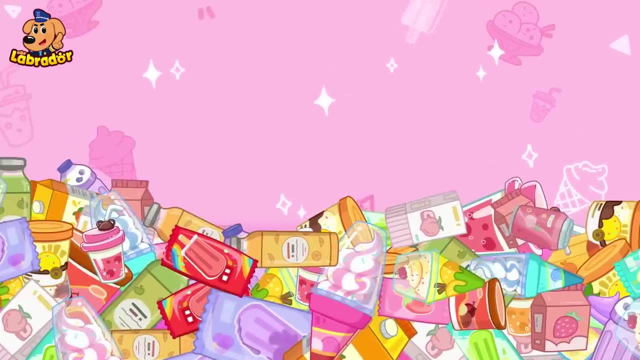 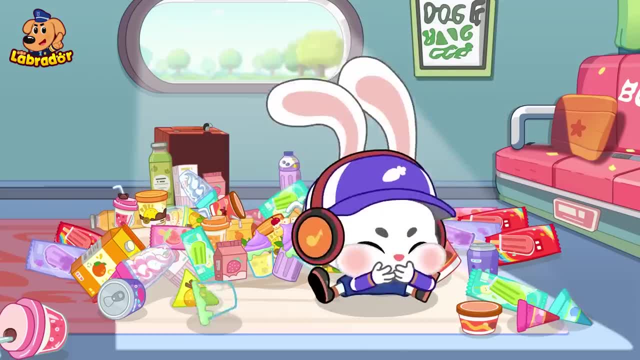 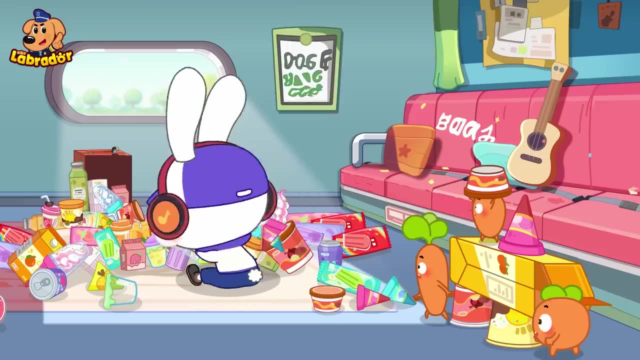 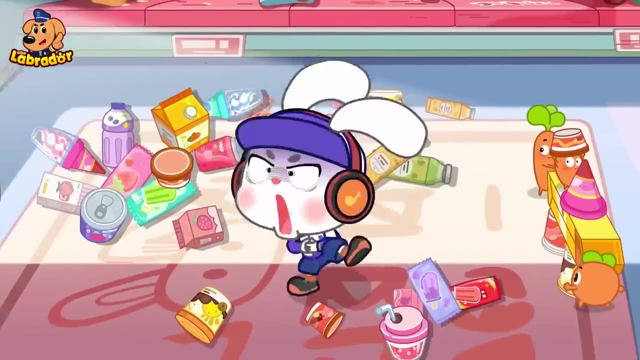 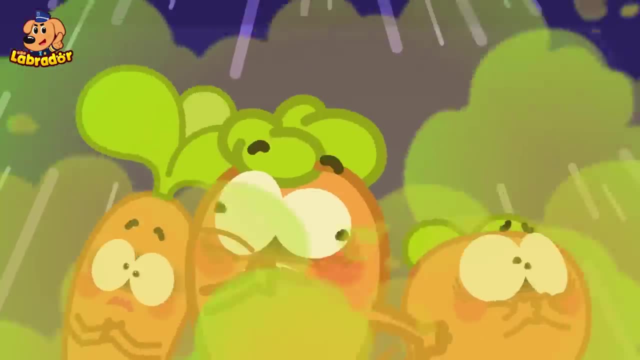 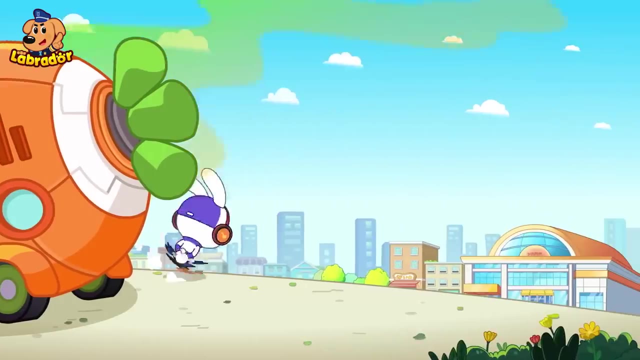 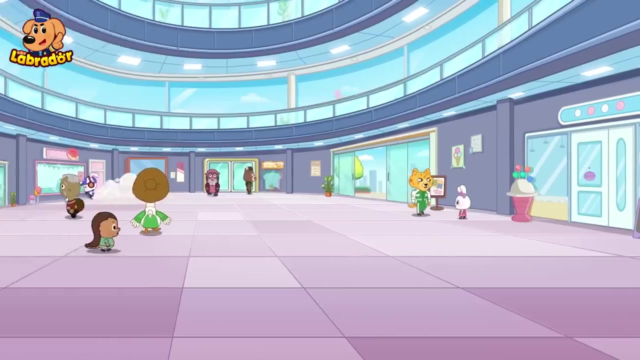 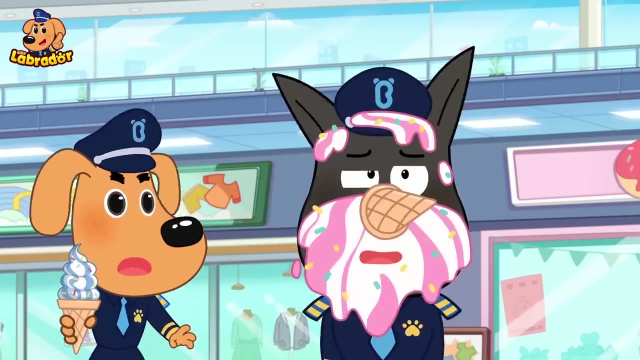 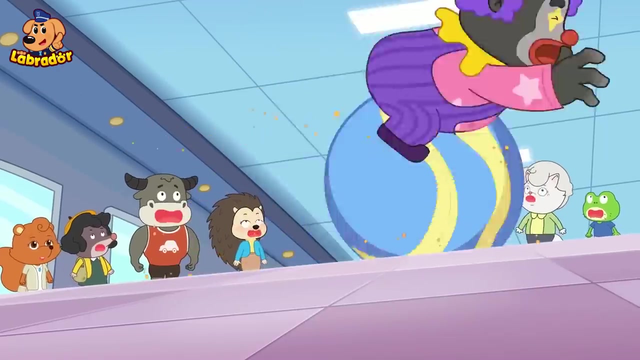 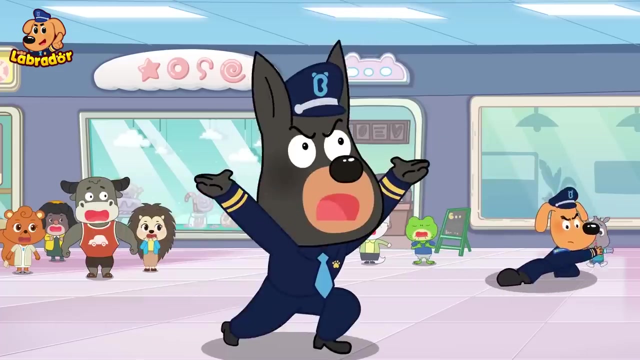 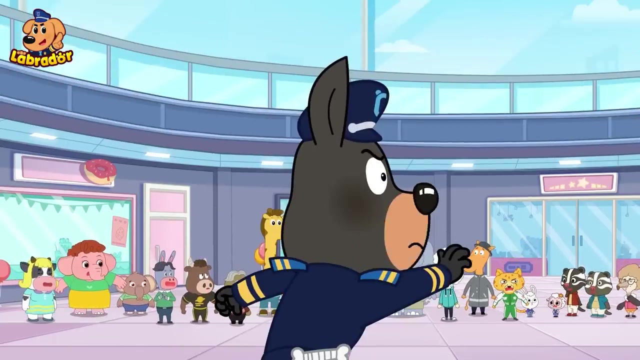 Ah, My tummy hurts. I need to go to the bathroom. Wow, Finally got one. Move aside. Move aside, Ah Ouch, Ah, Ah Ouch. Watch out, Hey, pee-pee rabbit, You shouldn't run around like that. 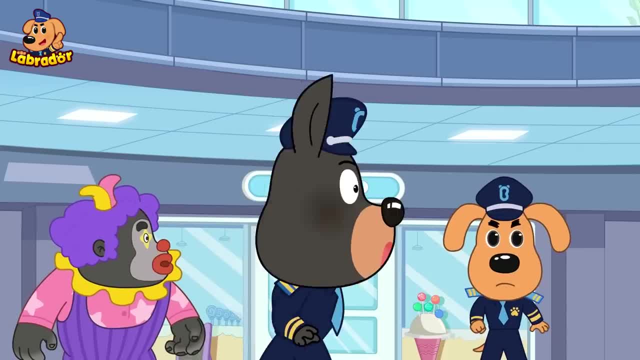 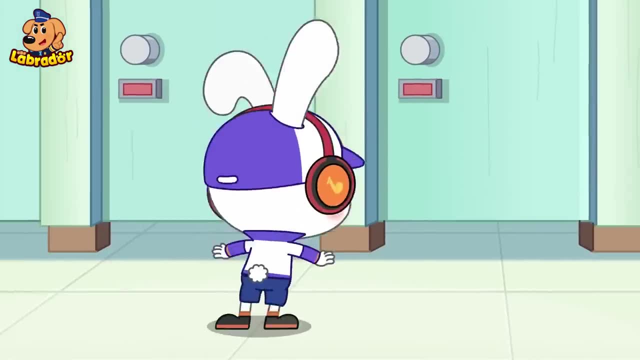 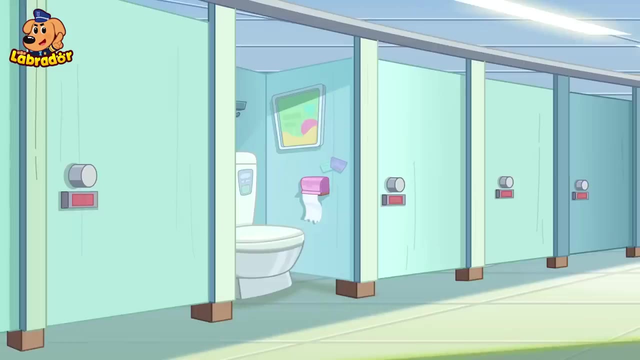 Dobby, I think he's looking for a bathroom because he has a tummy ache. The bathroom. Where is the bathroom Occupied? There's another one over there. Ah, Under repair. Ah, There it is, Ah, Oh. 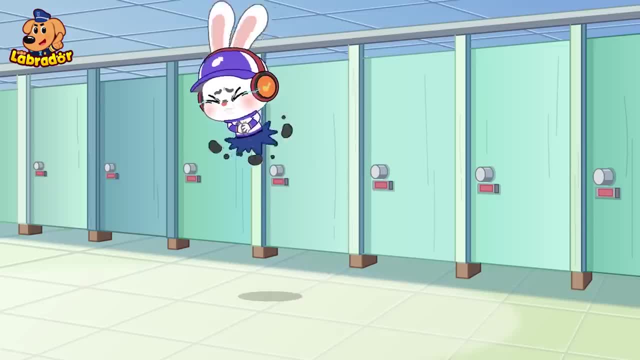 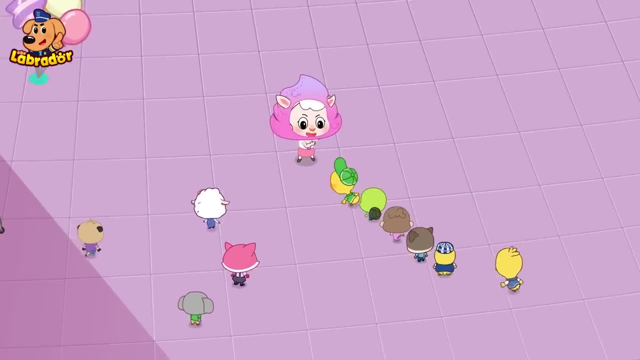 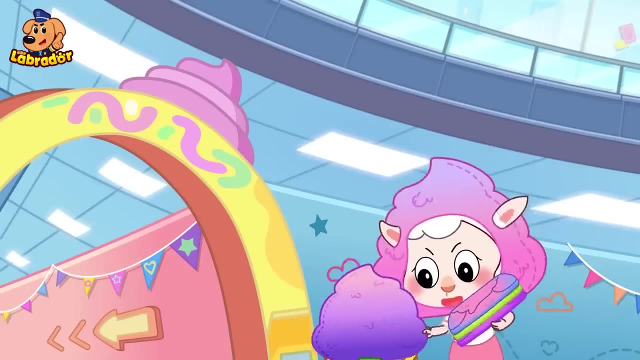 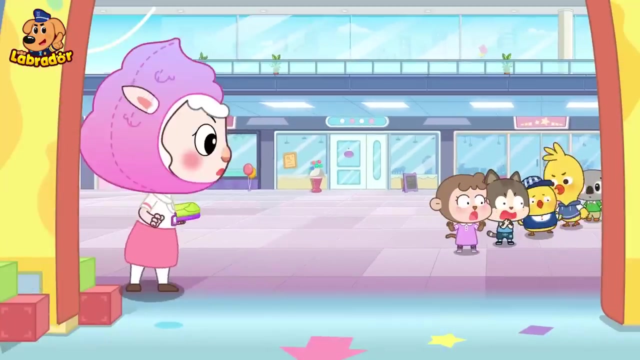 Come on, Seriously, I gotta find another bathroom now. Oh, Welcome to Poop May's Adventure. Oh, It's a bathroom. I wanna try. Here you go. Next, Here you go. Oh, Watch out, Wasn't he looking for a bathroom? 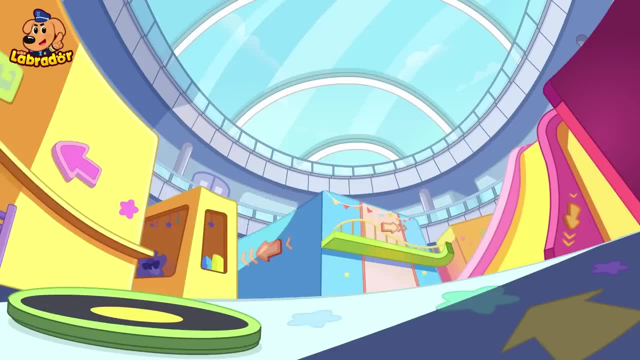 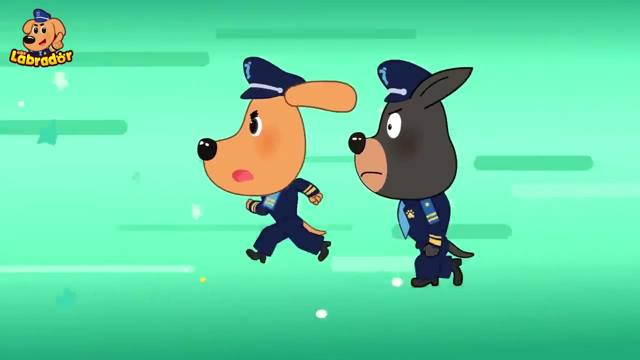 Why did he enter the maze? Ah? Why am I back here again? Ah Ah, Why is going to the bathroom this hard? Help me. Oh no, Pee-pee rabbit needs help. Ah, Ah, Ah. Sorry, There's an emergency. 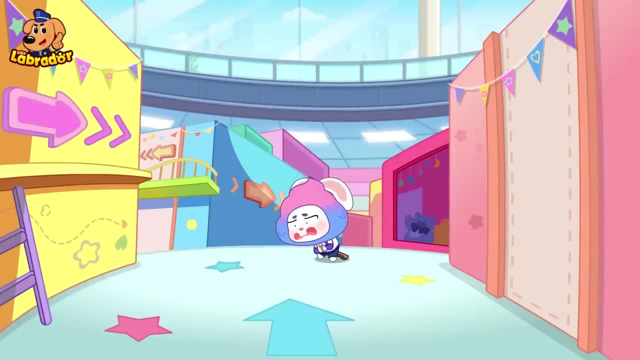 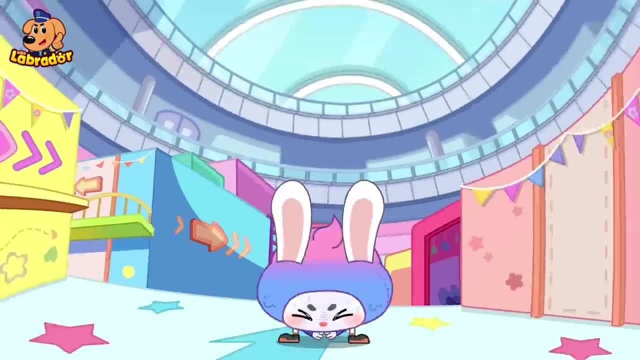 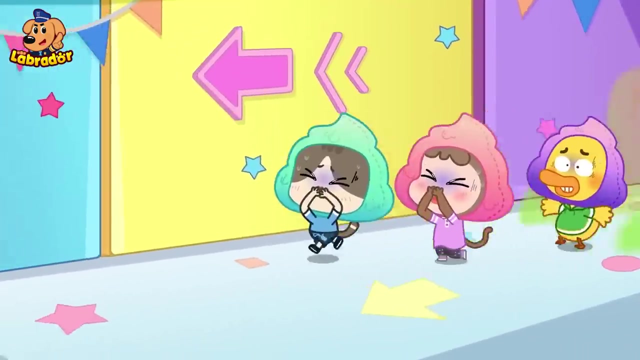 Huh Ah, My tummy hurts so much. Ah, Ahaha, Ah, Ah, Ah, Ah, Ah, Hahaha, Ah, Ah Auch. Ugh, Where's Pee-pee rabbit? Huh Ah. 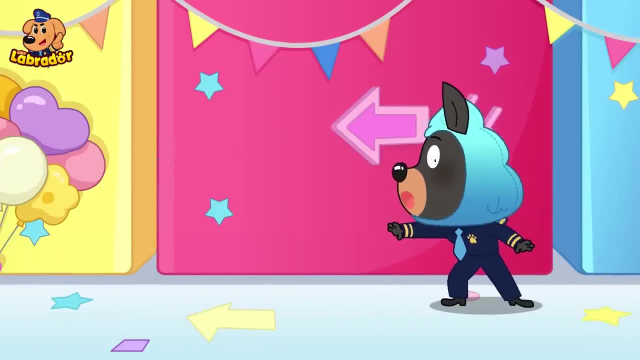 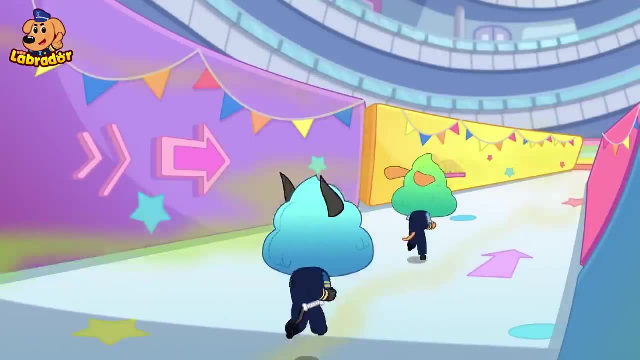 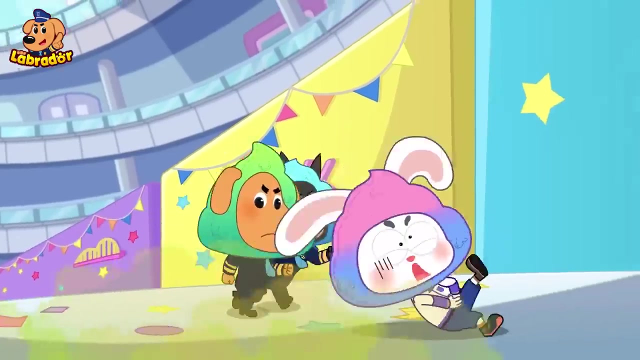 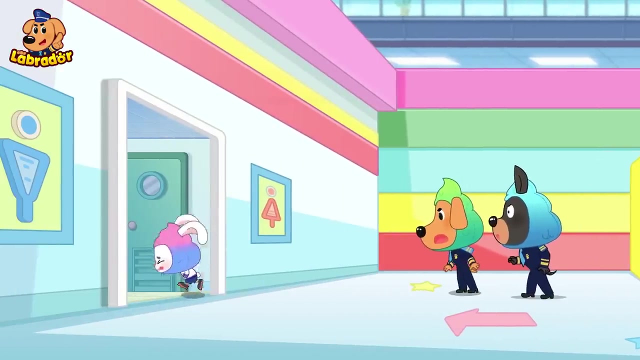 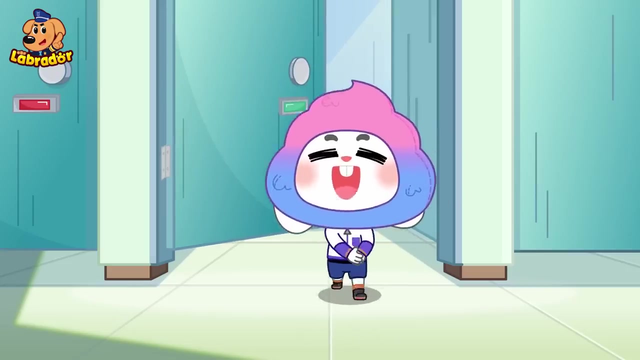 What's going on? Someone farted. It stinks. It must be Peepy Rabbit Over there. My tummy It hurts so much. Peepy Rabbit, Come on, We'll get you out of here, Hurry. Phew, I feel much better. 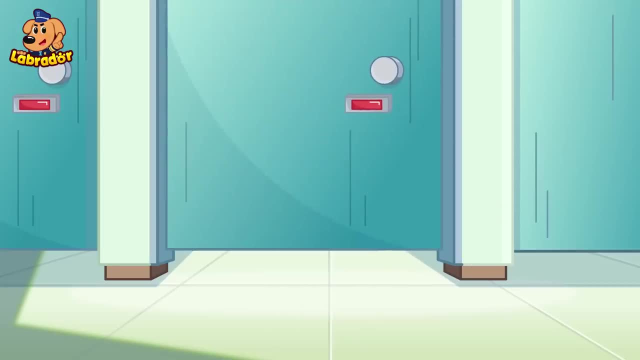 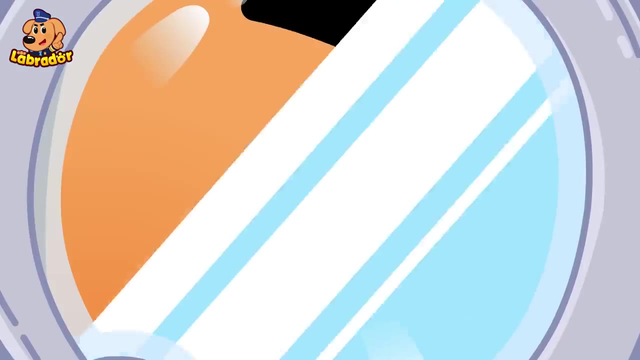 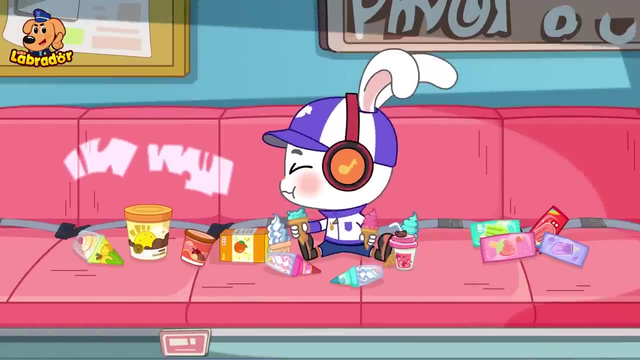 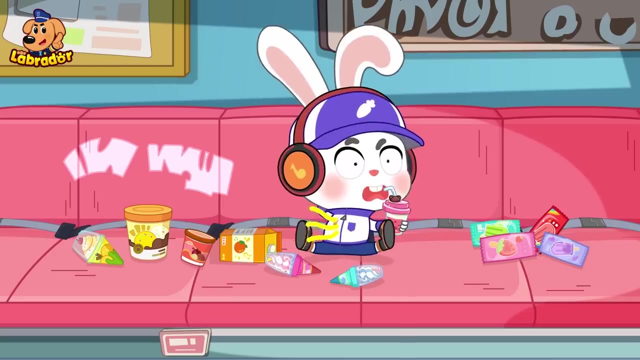 Oh no, I have to go again. I'll never eat so much ice cream again. Sheriff Labrador's Safety Talk: Kids. cold treats are delicious, but you shouldn't eat too much at once. If you eat too much of them, you might get a tummy ache or diarrhea. 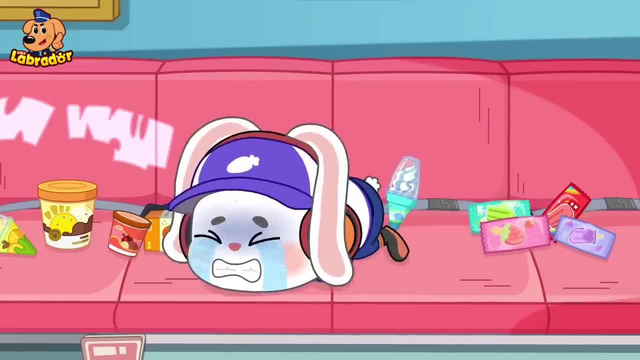 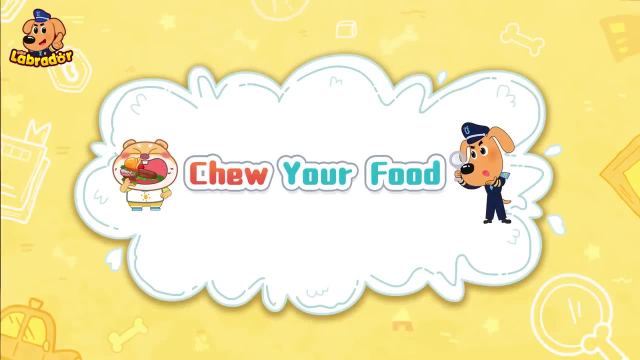 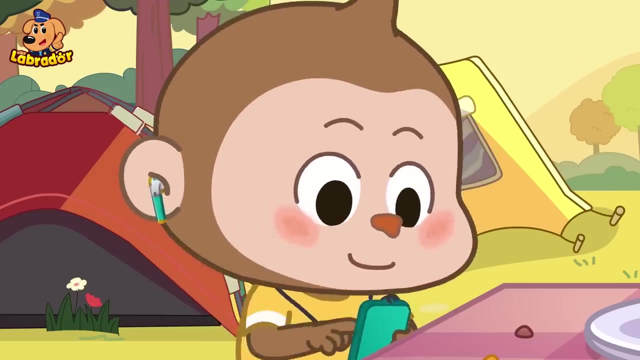 You might even vomit or get a fever, which is not good for your health. Remember, don't eat too many cold treats. Woof Chew your food. A long, long time ago there was a monster who loved to play hide and seek. 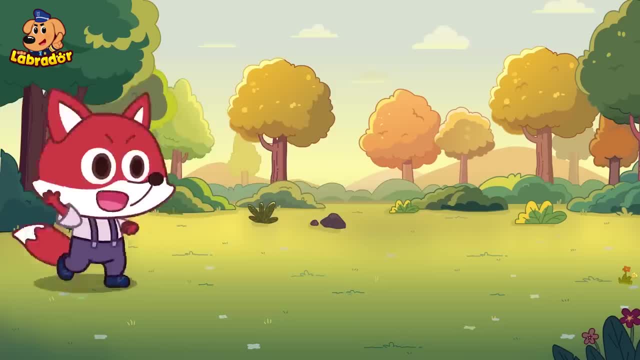 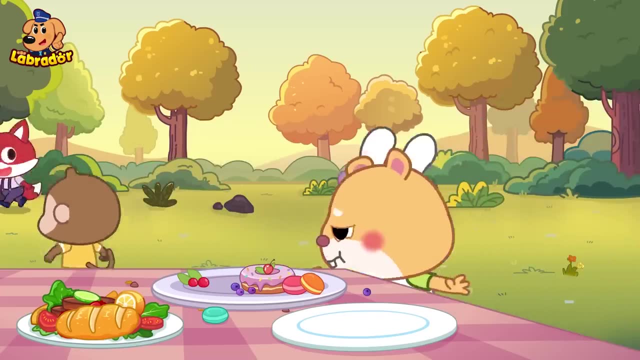 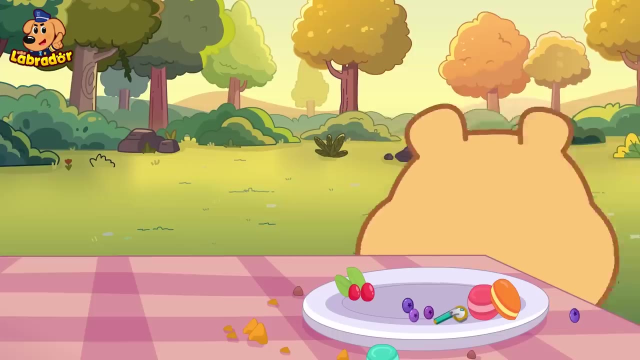 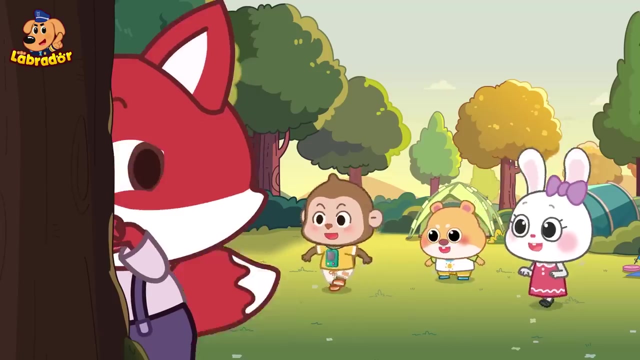 You should eat slowly, you little hamster. Come on, guys, Let's play Red Light, Green Light, I'm coming. Oh, Wait for me, Are you ready? Green Light, Red Light. Someone left, Come out now. 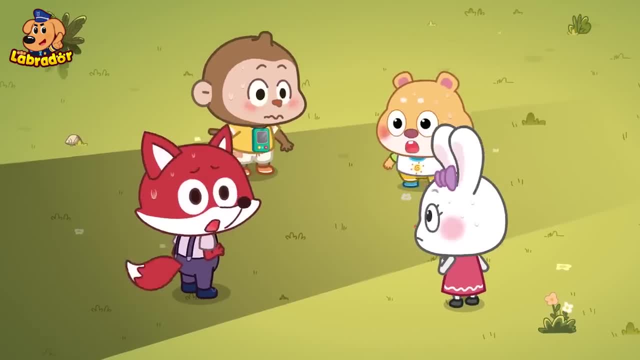 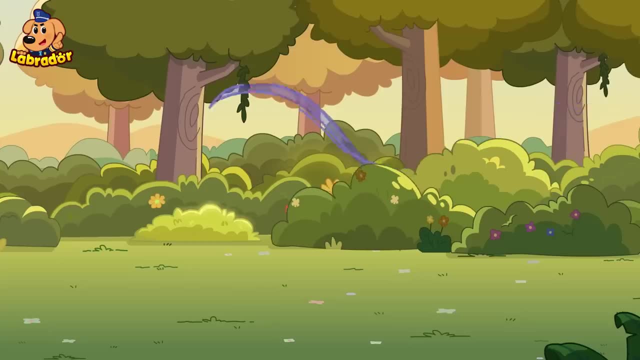 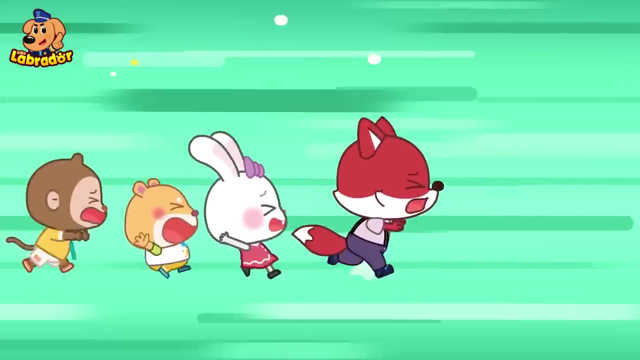 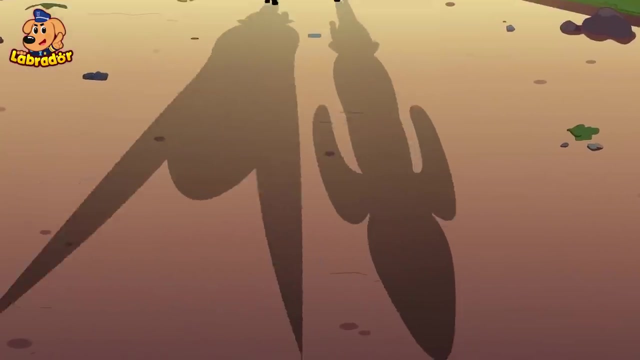 It wasn't us. Come and play with me. Who's talking? I'm coming for you. It's so scary. Aaaaaah, Aaaaaah, Aaaaaah. The monster's chasing us. Aaaaaah, Huh. 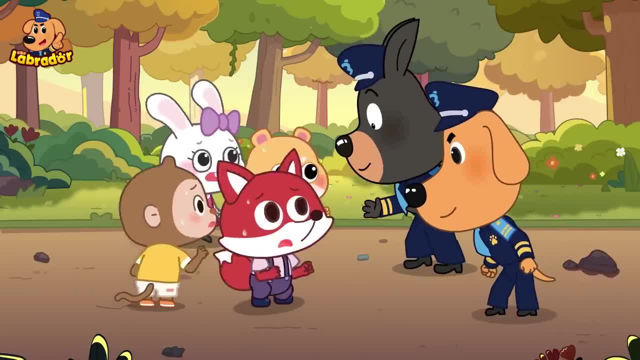 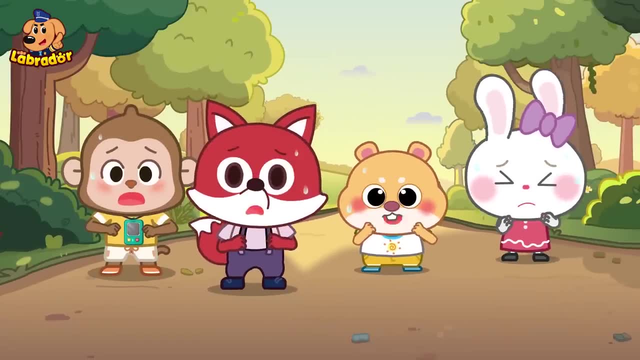 Don't be afraid, kids, It's us. Phew, What's going on? There was an invisible monster and it told us to play with it. It was so scary. Oh, An invisible monster, It's right over there. 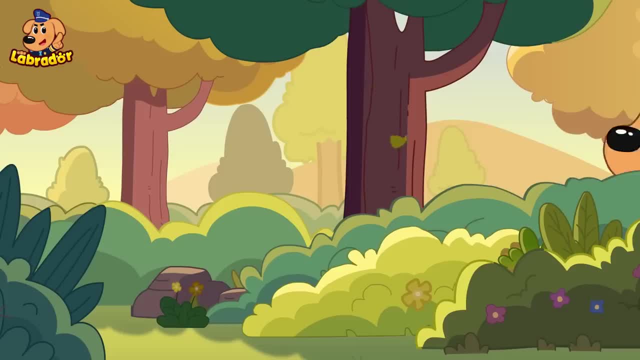 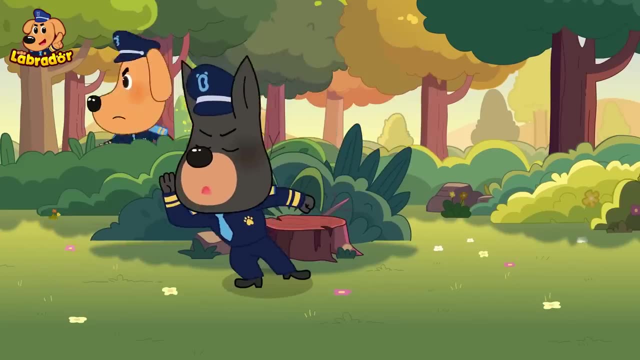 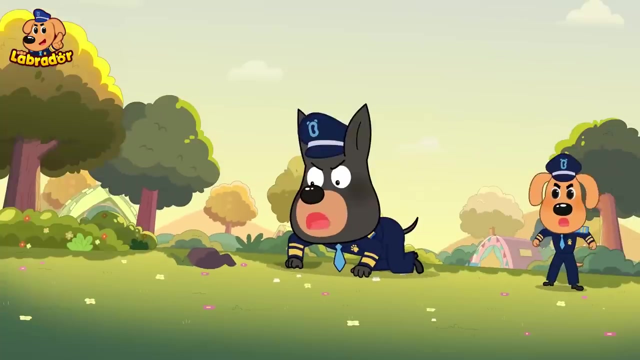 Let's go have a look. There's no invisible monster. It's probably just hiding somewhere. Huh, What's that sound? Huh, Huh, Huh, Huh, Huh, Right here, Huh Huh. 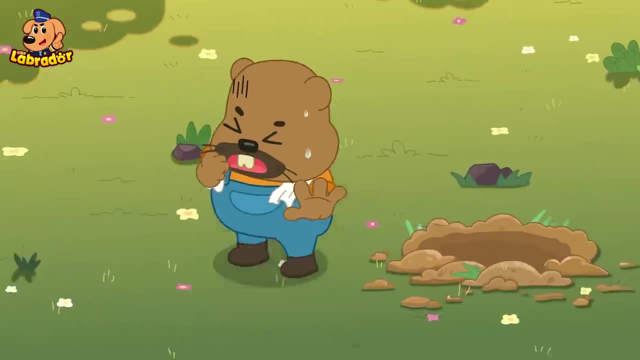 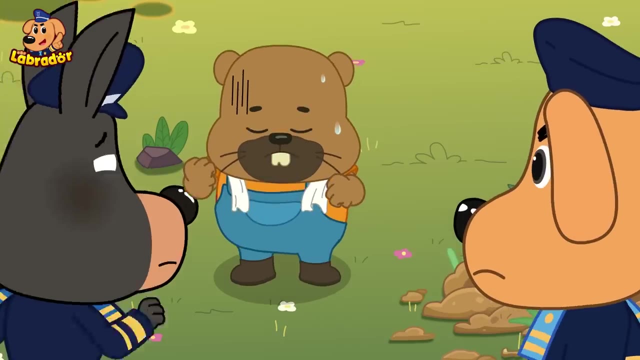 Huh, Huh, Huh, Huh, Go away, monster, Huh. Mr Marmot, I'm Officer Doby, not a monster, Phew, But I heard a strange sound coming from the tent. It was so scary. 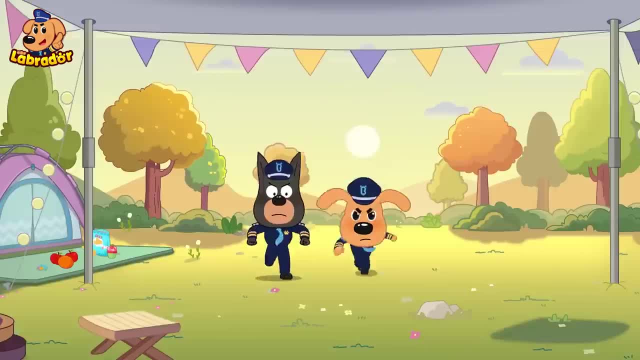 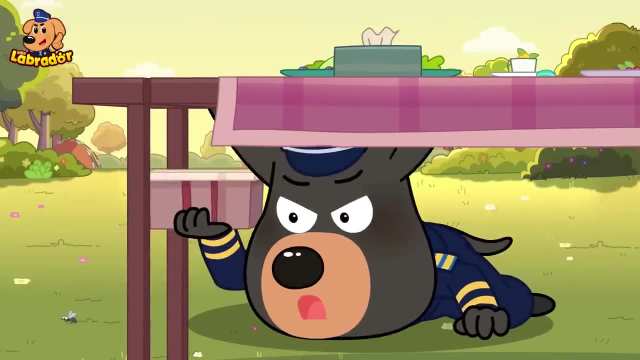 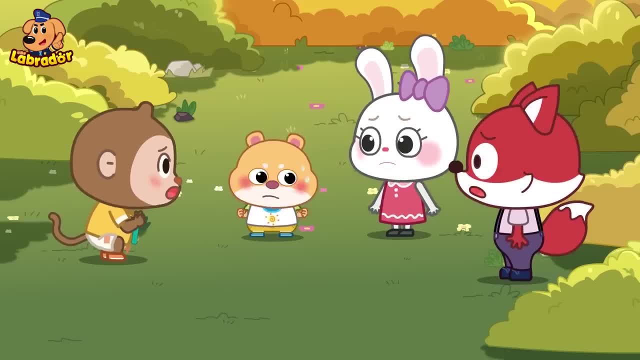 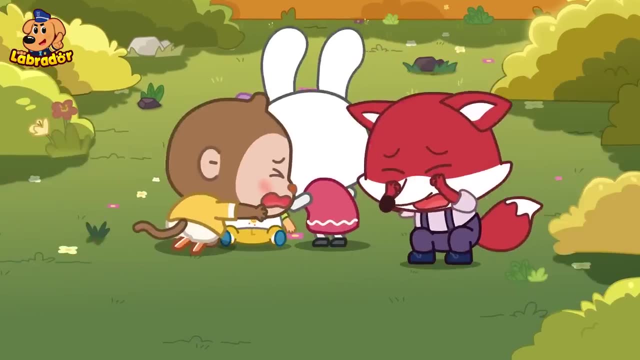 Hmm, Why is this earphone on the plate? Don't be afraid, guys, Sheriff Labrador will catch the monster. Ha-ha-ha, You will find me. I'm hiding right here. Ah, The sound is coming from Little Hamster's tent. 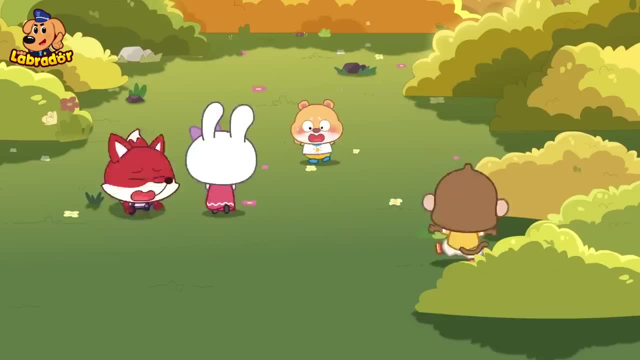 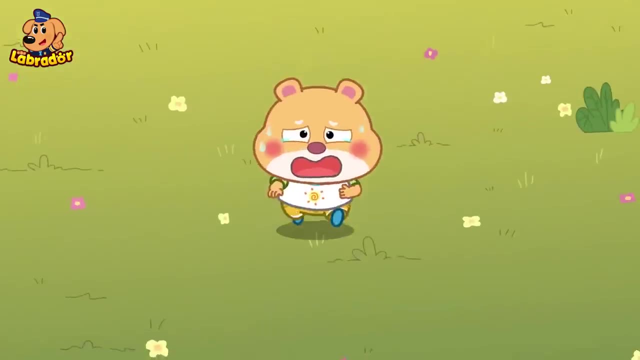 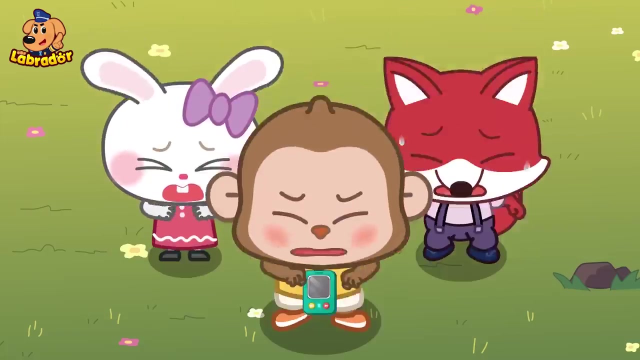 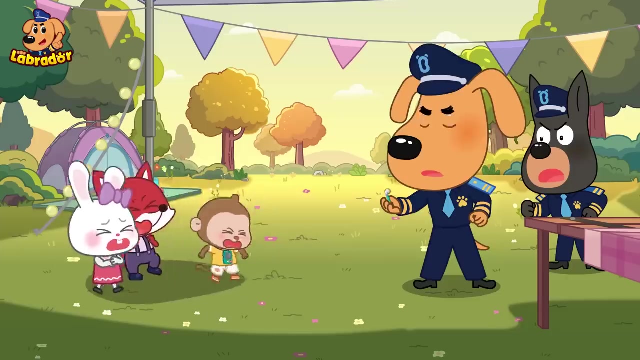 from Little Hamster's tummy. How did it get into my tummy? Oh my tummy, Sheriff Labrador The monster, It's inside Little Hamster's tummy. What, Uh, what's that? Ah, That's the monster's voice. 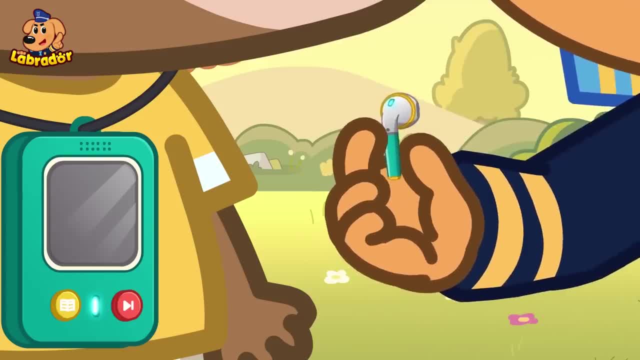 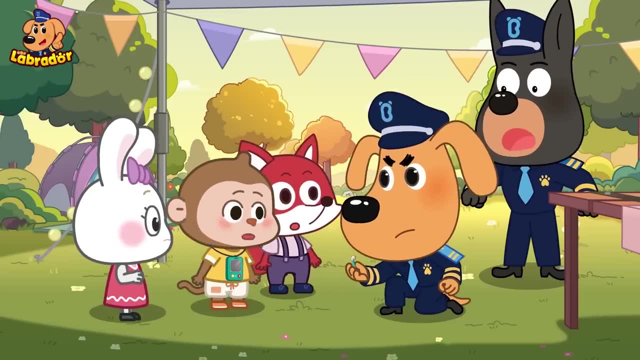 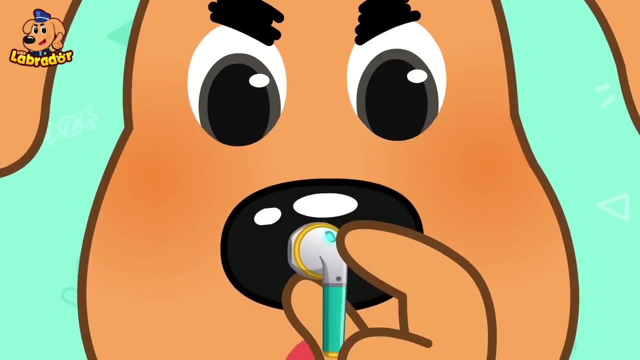 Don't be afraid, The sound just came from the earphone. Uh Little Monkey, is this yours? Yes, I put it on the table, But where's the other one? Hmm, the earphone on the plate and the monster's voice coming from Little Hamster's tummy. 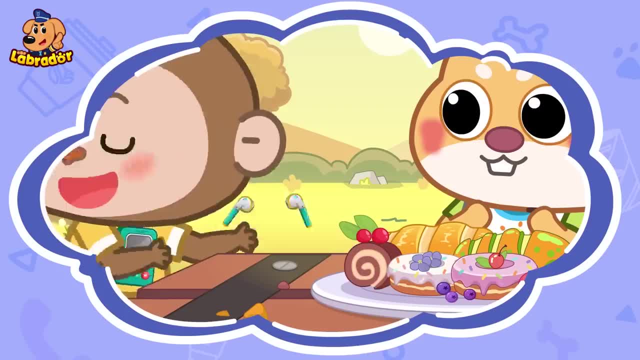 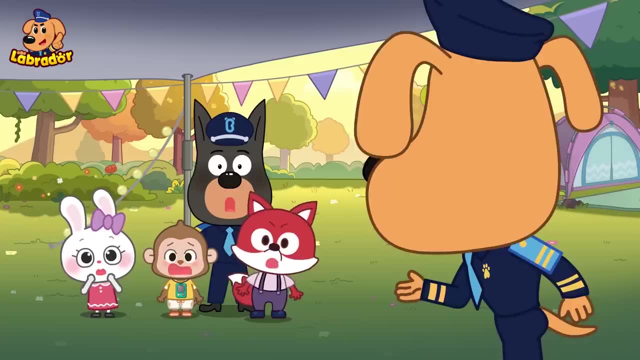 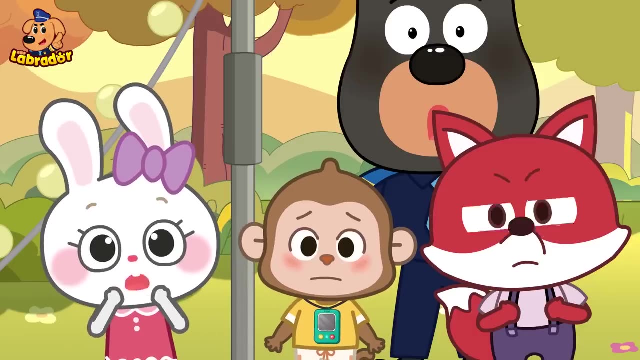 I got it. Little Monkey's earphones fell on the plate And Little Hamster ate one of them. Oh, that's why the sound was coming from his tummy. Oh, I remember. now Little Hamster gobbled up the food. 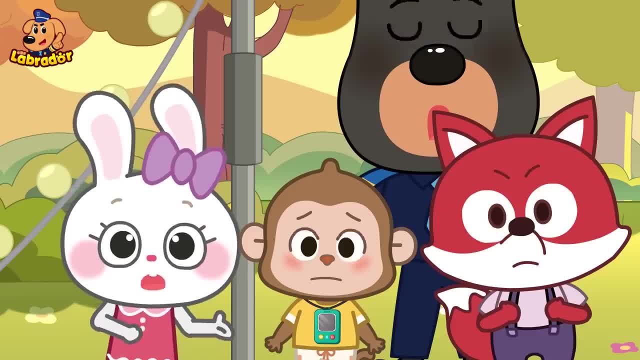 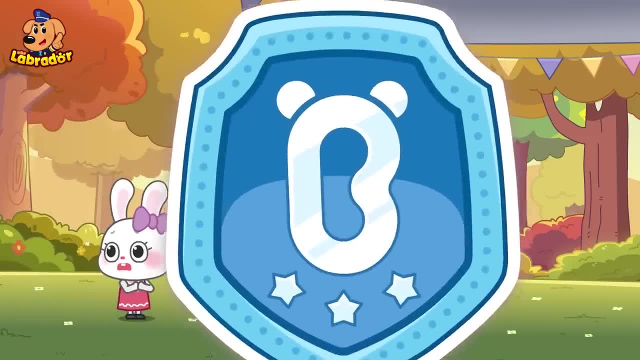 and I told him to take his time and chew his food. Where is he now? We need to take him to the hospital. He went that way. Toby, let's go. Little Hamster, Little Hamster, Little Hamster, Oh. 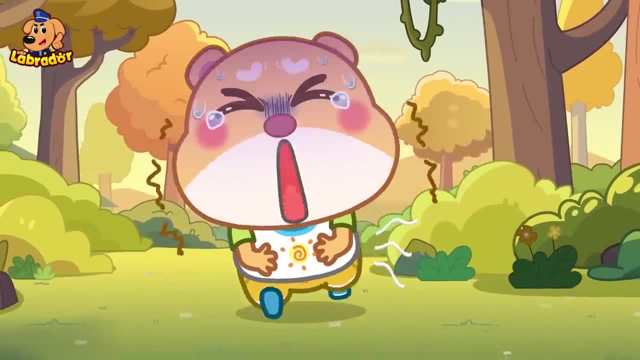 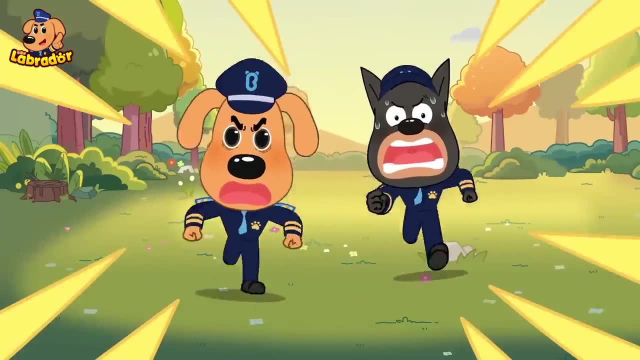 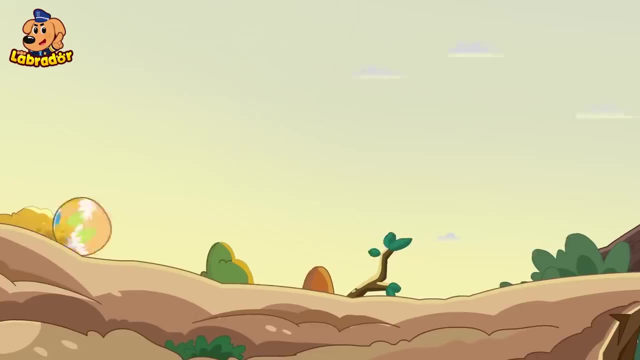 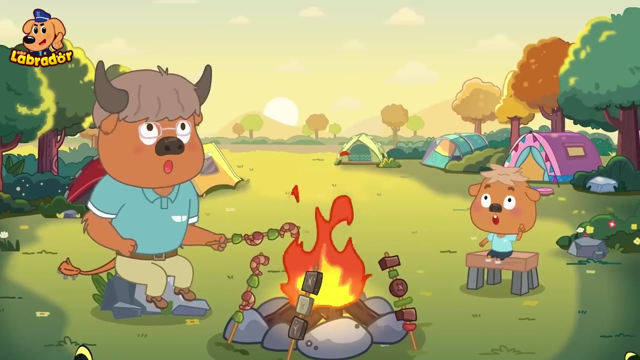 It hurts so much. Please come out of my tummy, Ow, Ow, Ow, Ow, Watch out, Whoa, Whoa, Whoa, Whoa, Whoa. Ow Daddy look. Ah, Whoa, Oh. no, The road is blocked. 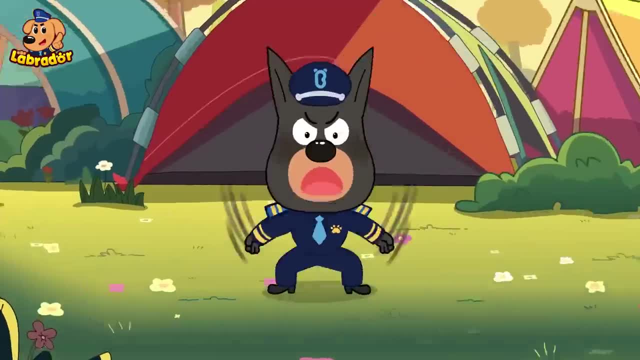 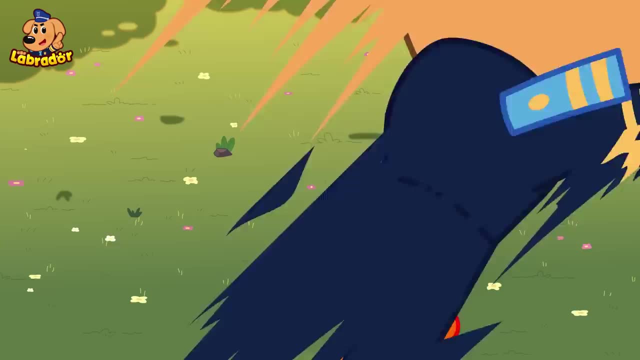 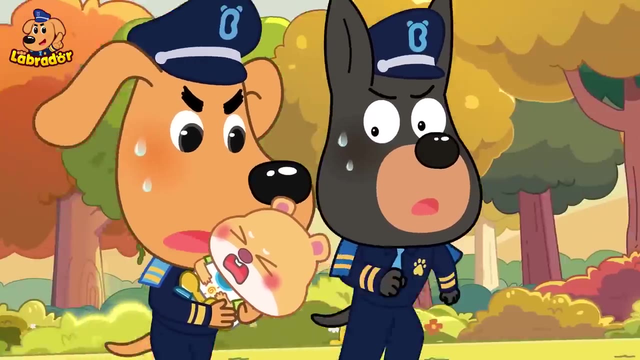 Toby, Leave it to me. Hey, hey, hey, hey, hey, Hmm, Ah Ha, Oh, Ha ha ha. My tummy hurts so much. Little Hamster, you've swallowed an earphone. We'll take you to the hospital now. 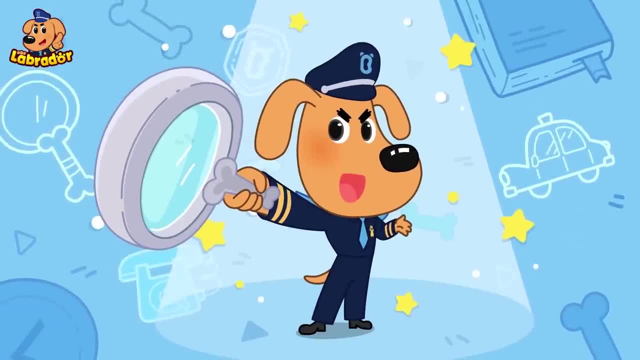 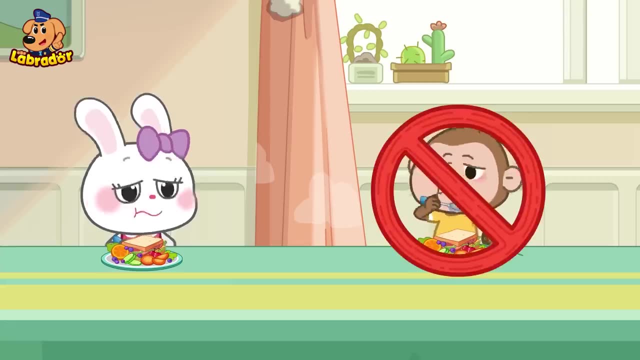 Sheriff Labrador's Safety Talk. Kids, when you eat food, you should chew it well, Don't gobble it up, Otherwise it might cause indigestion or you might accidentally swallow something that isn't food. If that's the case, let an adult know. 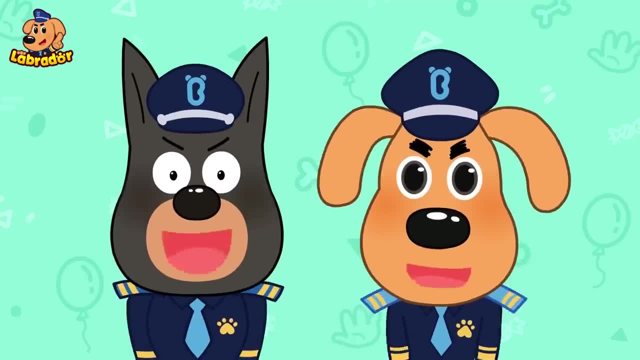 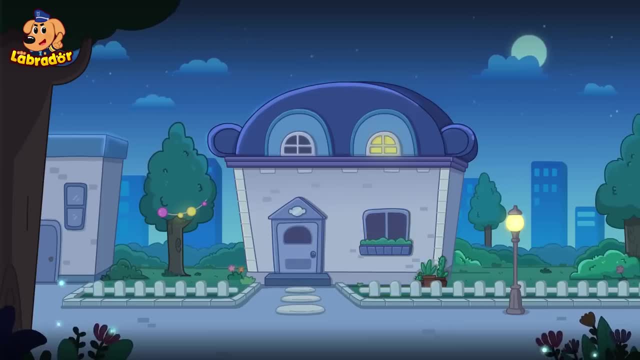 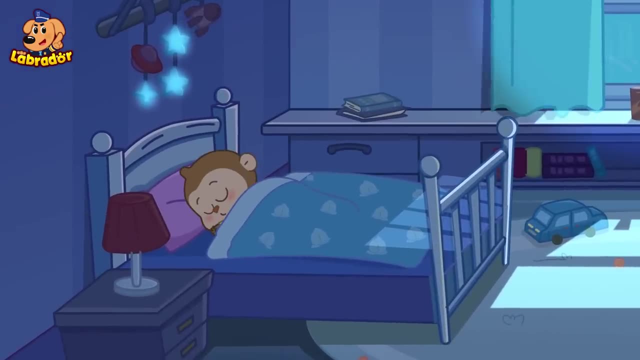 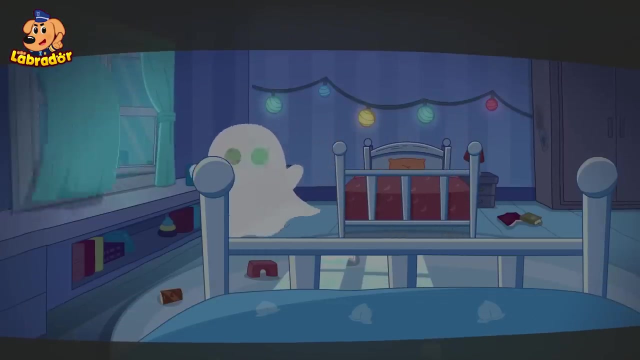 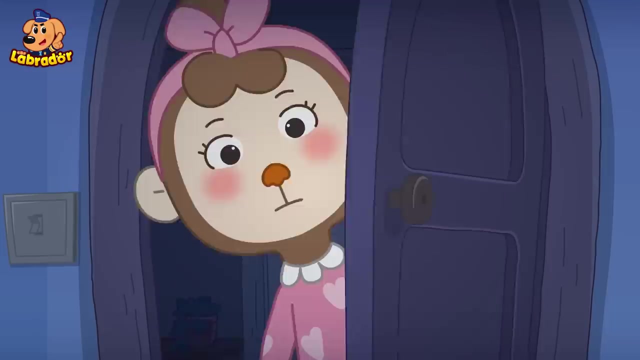 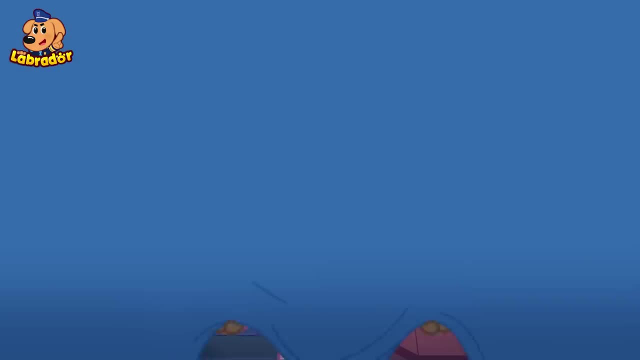 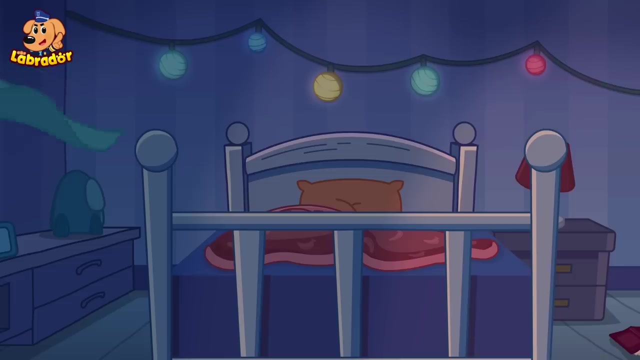 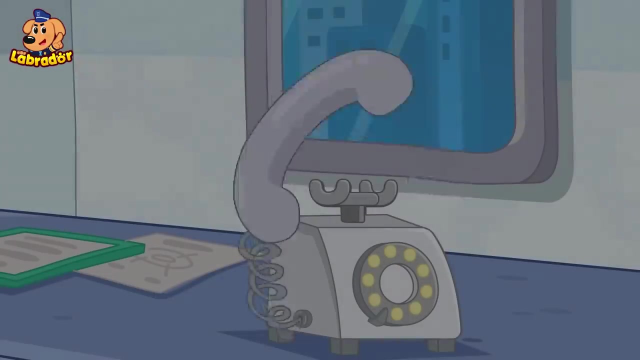 Uh, I saw a ghost. Oh, don't be afraid, sweetie, Mommy's here. Huh, Where's your sister? Oh, a ghost must have taken her. A ghost Woof. Hi, I'm Sheriff Labrador. my daughter is missing. 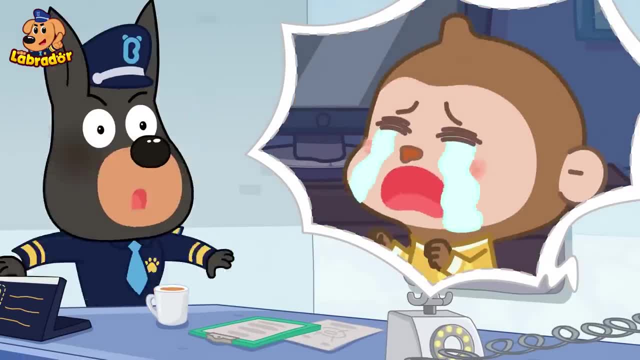 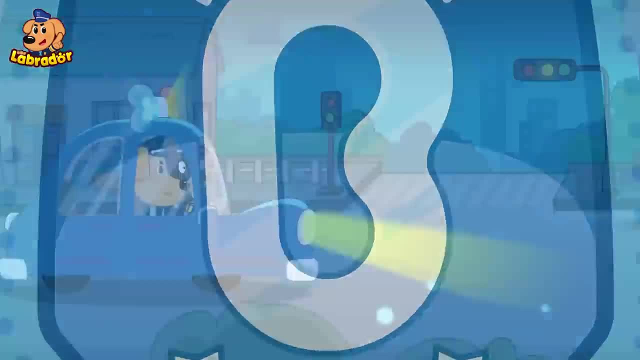 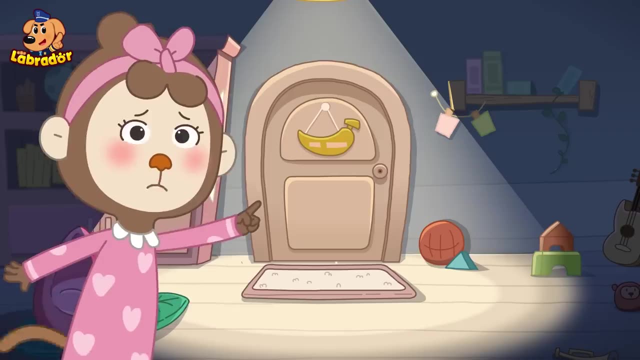 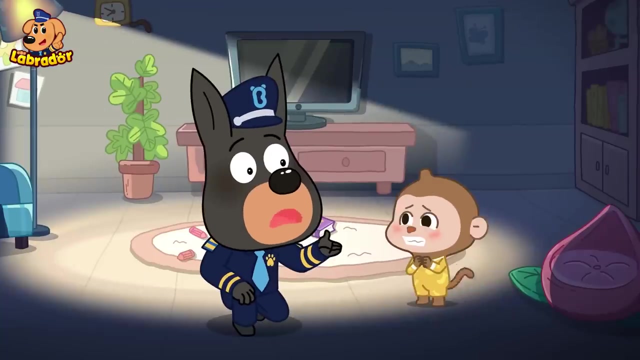 Please help me find her. A ghost. Help her A ghost, Don't worry, we'll be right there. Sheriff Labrador, my daughter was sleeping in this room And suddenly she disappeared. The ghost must have taken her. Hey, kid, there's no such thing as a ghost. 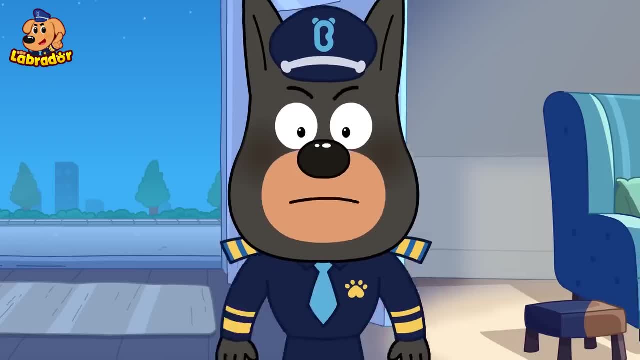 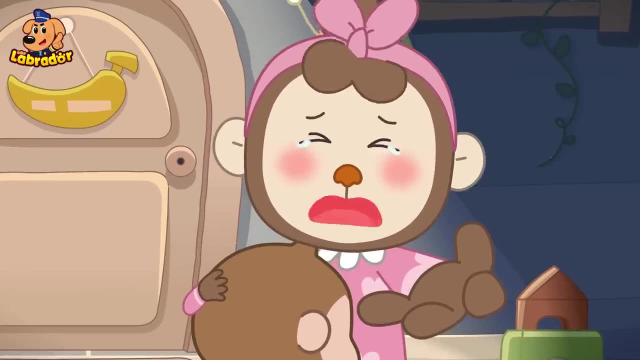 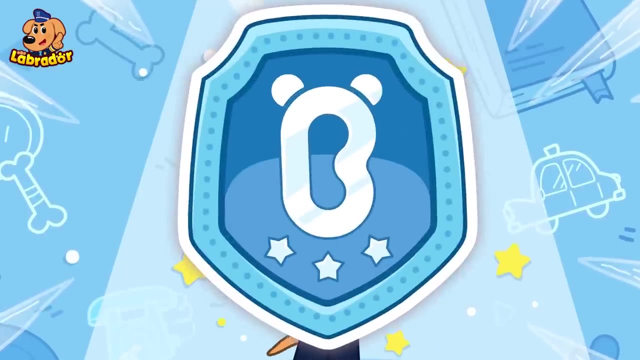 But I saw it. It was white and its eyes were bright and green. It was so scary. Sheriff Labrador, please save my daughter. Don't worry. There's no case that I can't solve. Let's search Sister Monkey's room first. 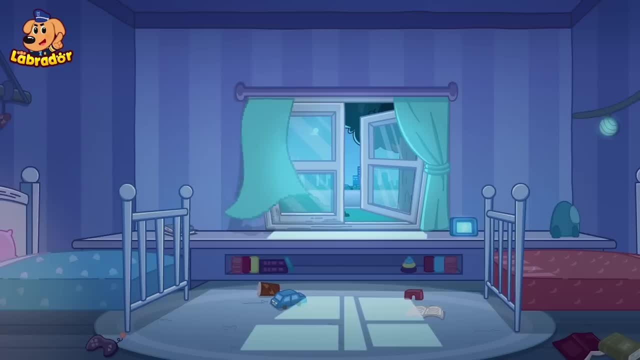 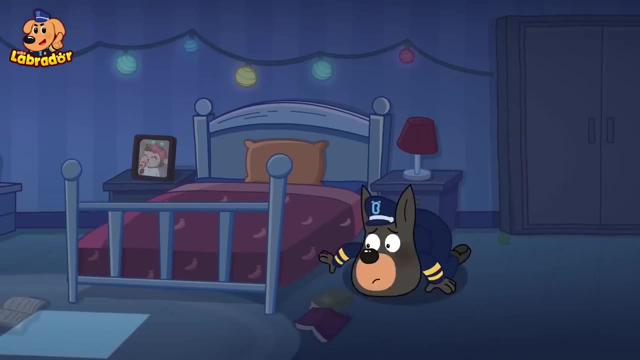 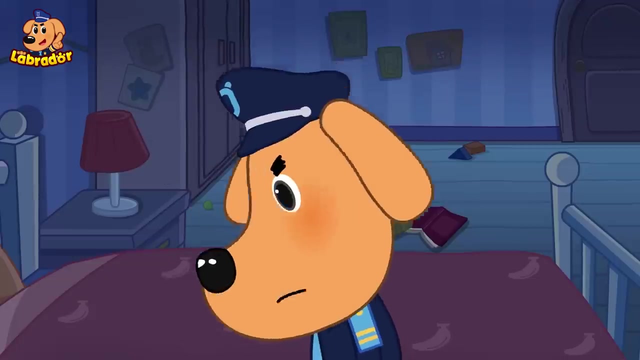 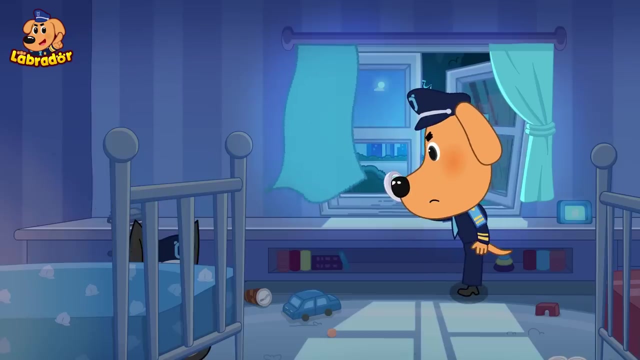 This is a photo of Sister Monkey. There are only child's footprints on the windowsill And there's no sign that the window was forced open. I don't think she was taken by anyone, So there's no sign that the window was forced open. There's no sign that the window was forced open. 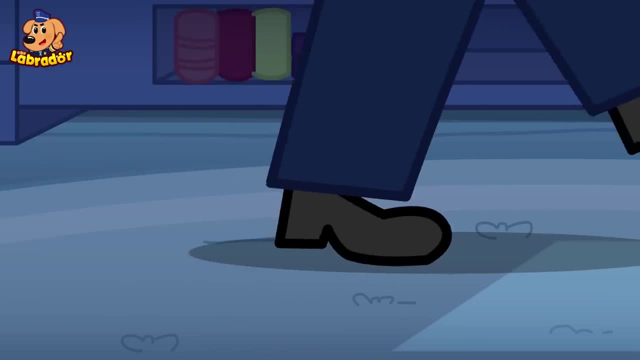 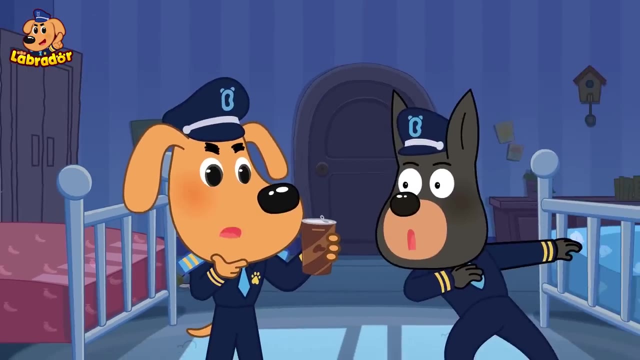 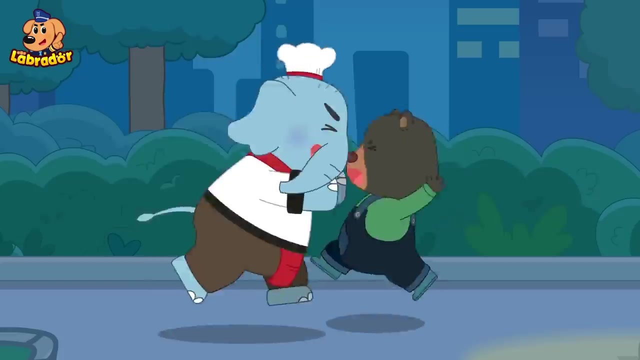 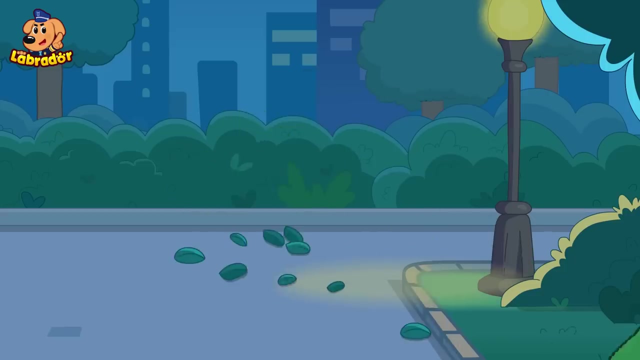 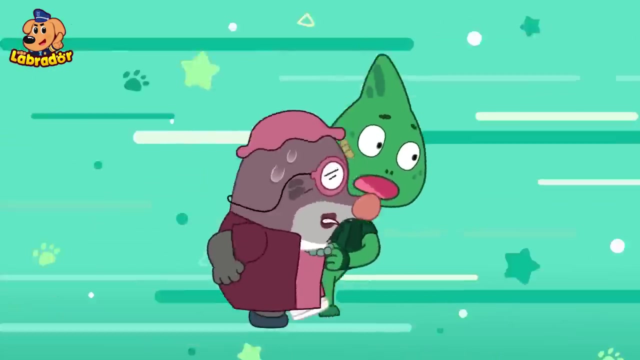 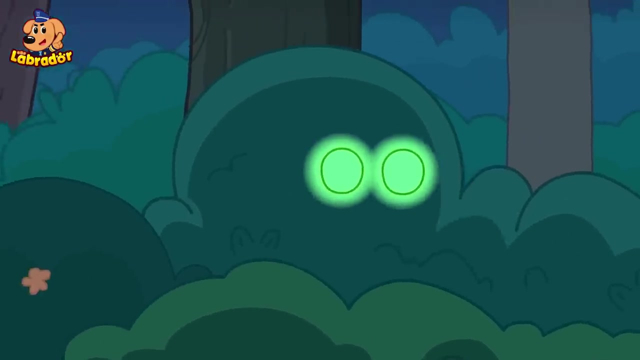 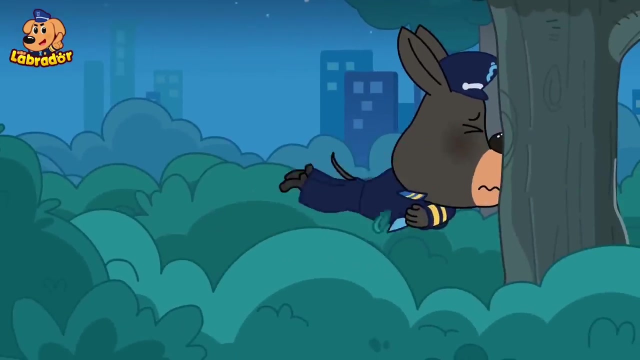 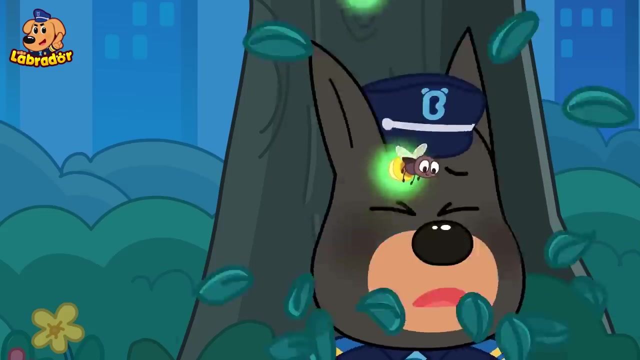 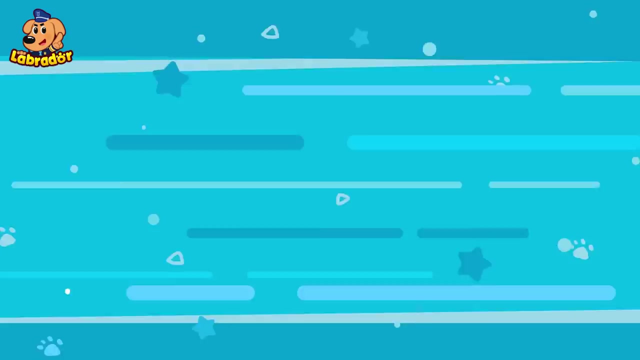 There's no sign that the window was forced open And there's no ghost. And there's no ghost. It's coffee. Coffee Ghosts Run, The ghost is coming, The ghost is coming. The ghost is coming There. it is Stop right there. 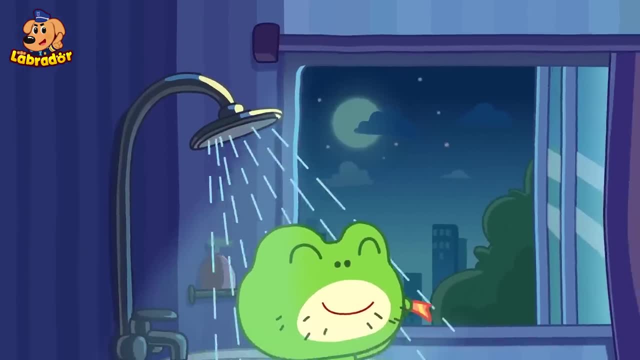 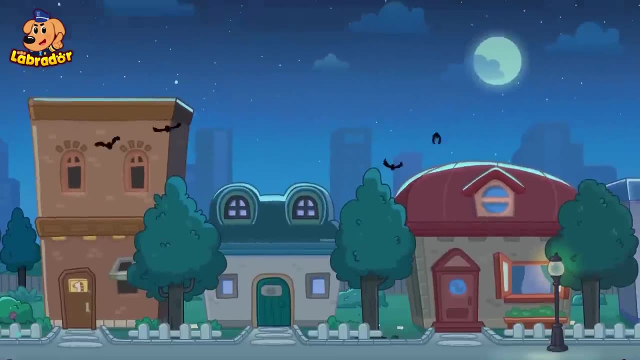 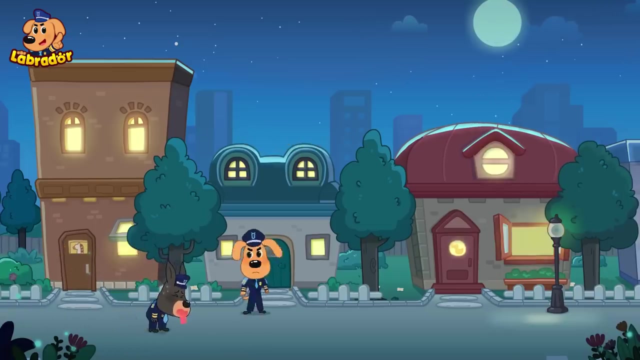 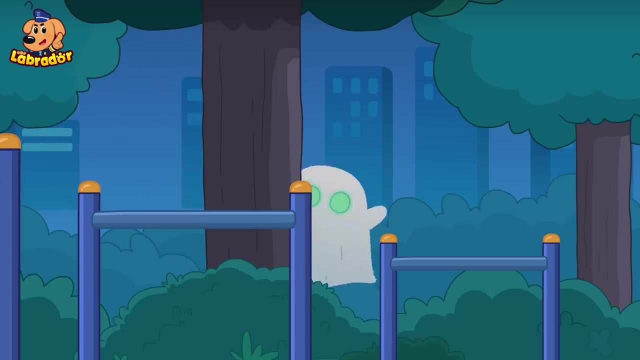 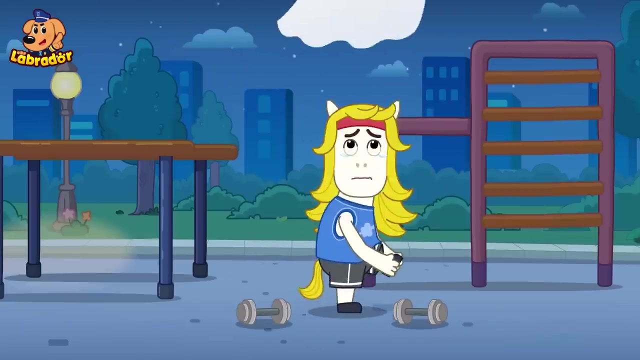 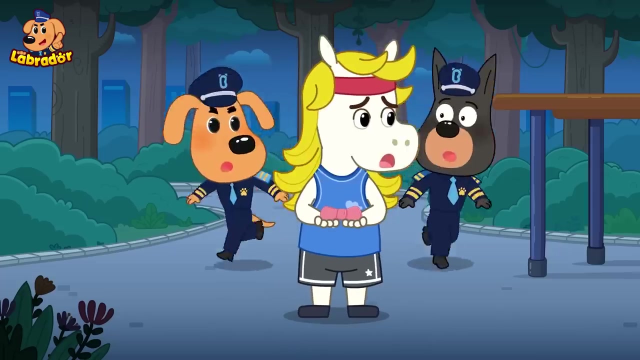 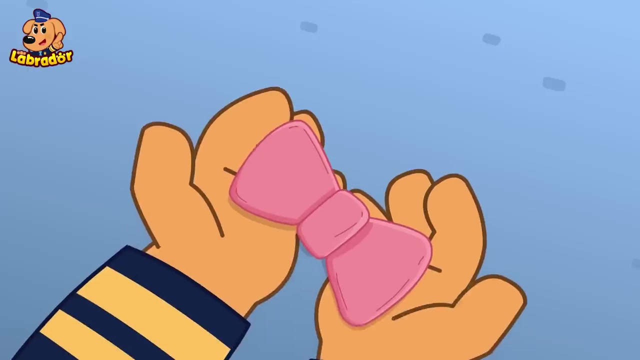 I'm gonna get you: It's a ghost Ghost. It's a ghost Ghost. It's a ghost Ghost, It's a ghost Ghosts. Sheriff Labrador, the ghost has just dropped this: A ribbon And a flashing headband. 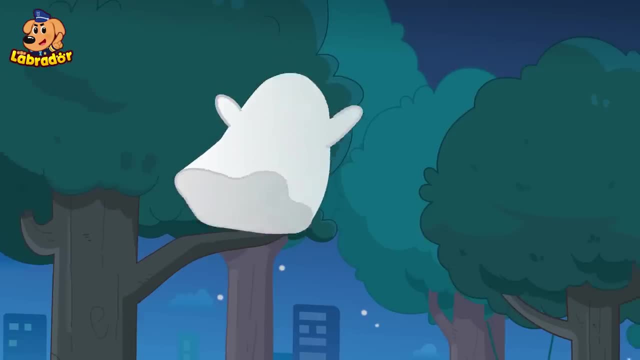 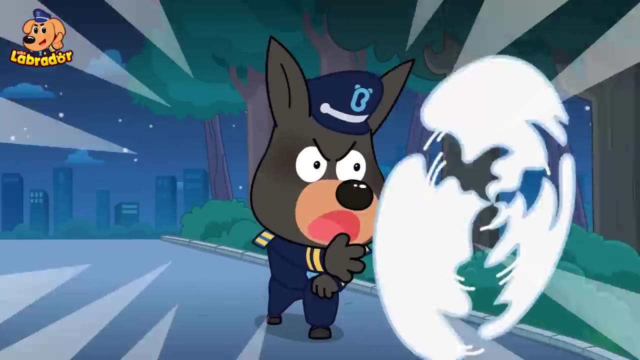 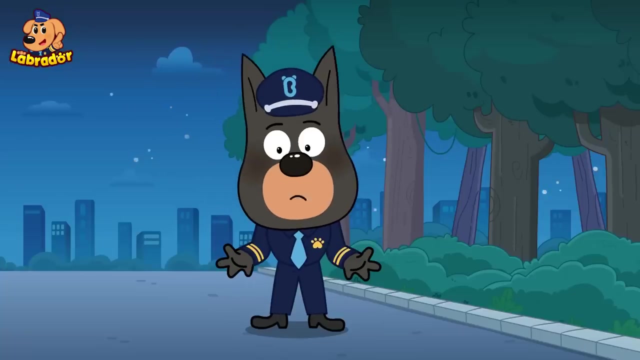 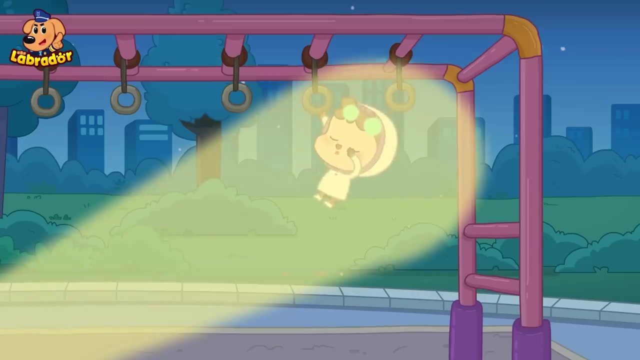 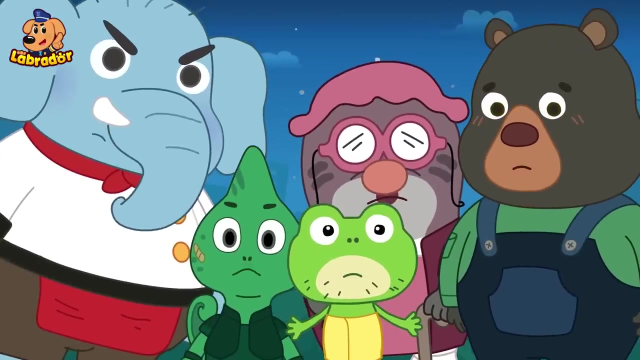 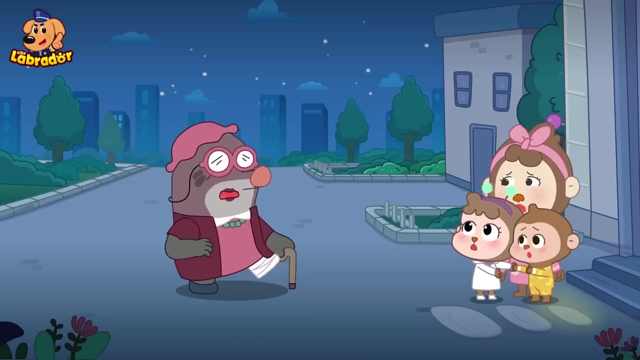 I know what it is. No one can run away from me. Why are you helping the ghost? It's not a ghost, It's Sister Monkey. Huh, So it was Sister Monkey, Sweetie. Children should be sleeping at home at night. 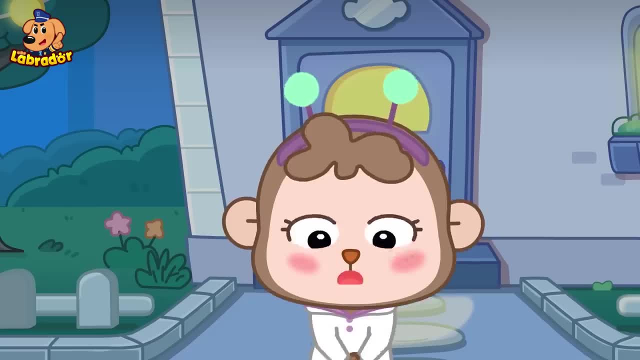 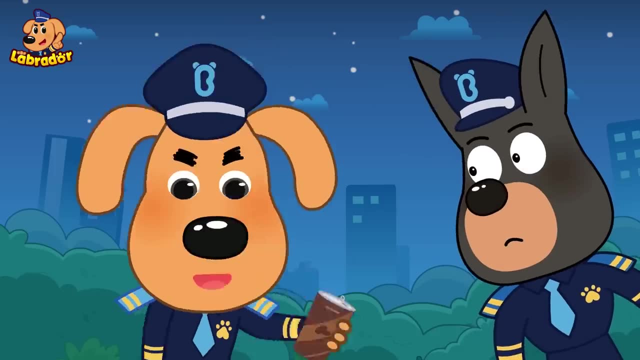 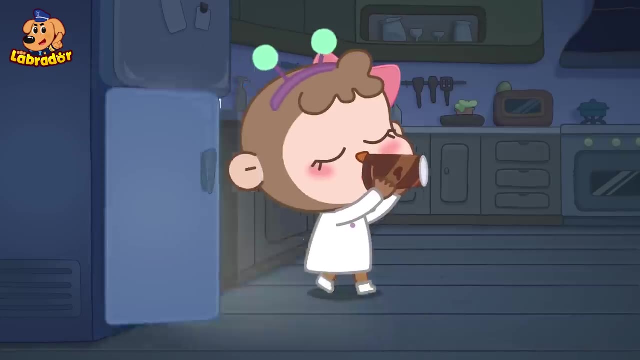 Why are you out and scaring people like that? I'm sorry. I couldn't fall asleep so I came outside to play Sister Monkey. did you drink this? Yes, I was thirsty, So I took it from the fridge and drank it. 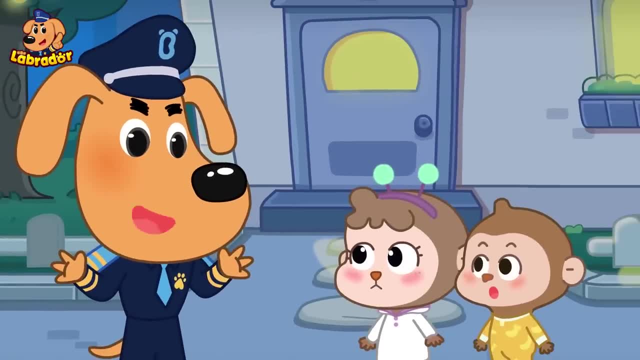 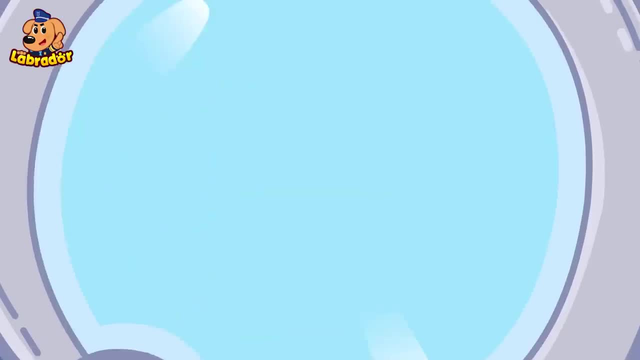 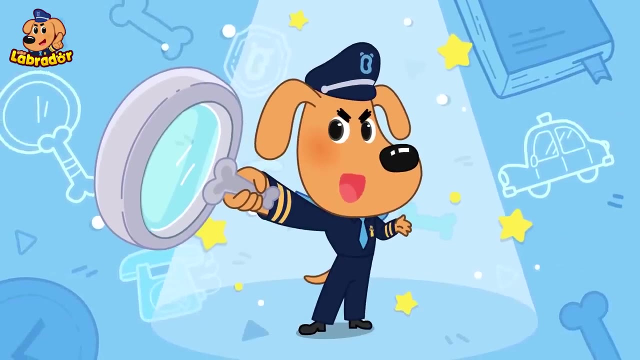 Coffee is for grown-ups. Children can't sleep if they drink it. Oh, I see. Ah, I'll be careful of what I drink from now on. Sheriff Labrador's Safety Talk: Kids coffee is a drink that's only for grown-ups. 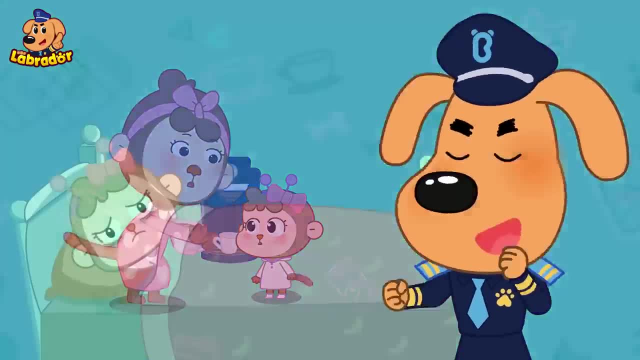 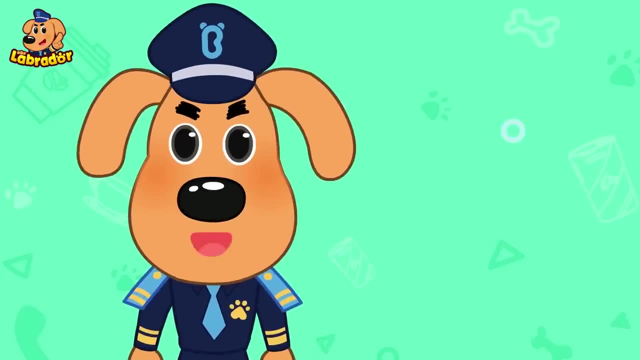 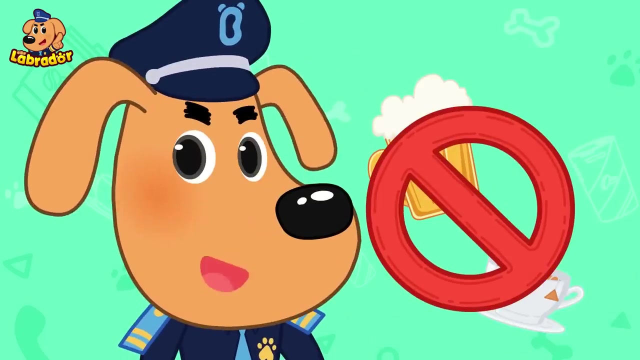 Because if children drink coffee, they can't fall asleep at night, And it's not good for their health. Also, tea and drinks that contain alcohol are not for children either, And you shouldn't drink them. Please keep that in mind. Woof.